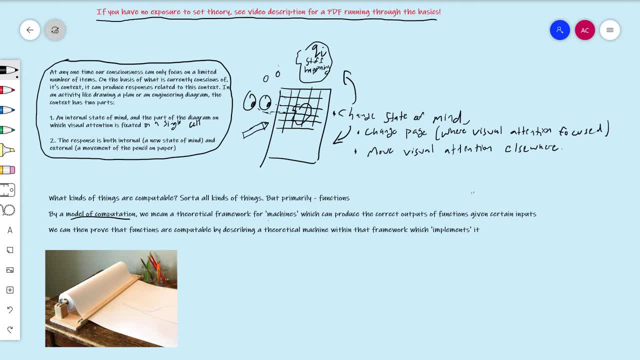 It was more based on how people think, And so we had this kind of idea in mind. We were starting to break down the process of somebody thinking at a desk with a piece of paper and a pencil And the breakdown kind of came. 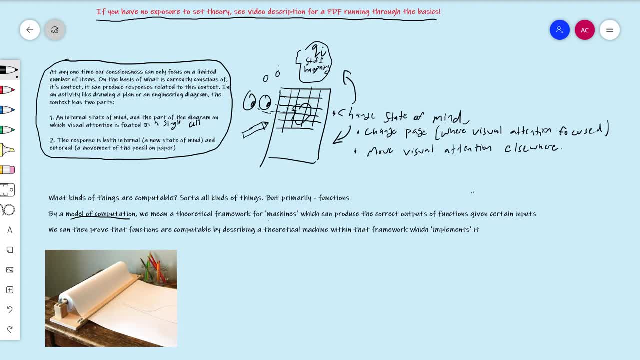 The breakdown was sort of something like this: And this is sort of. So we're going to begin with this kind of informal modeling of human thought and then we're going to formalize that gradually into a mathematical definition, But the formal, the informal model of our thinking. 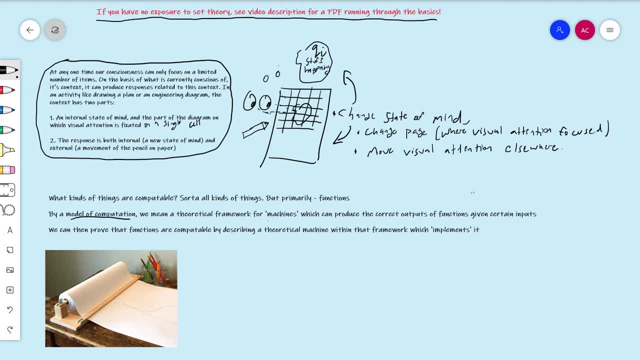 is that, basically, at any one moment, at any one discrete moment in time, we are focusing on a particular point in the page, Maybe right here, And we have. We have a state of mind, There's something going on in our head. 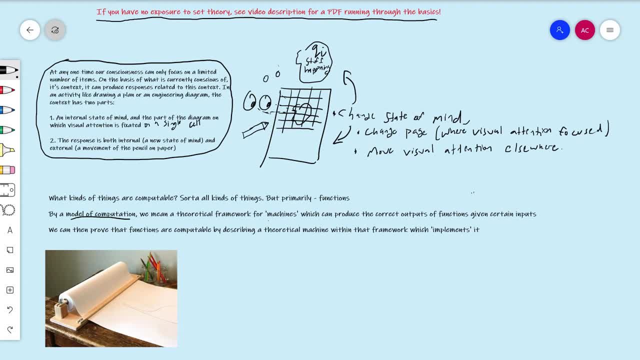 We have our pencil right here, and so there's two fundamental defining features of the current situation. is that I'm looking somewhere on the page. It's not really the location of what I'm looking, hat matters, It's what I'm seeing, right? I'm seeing something specific on the page. 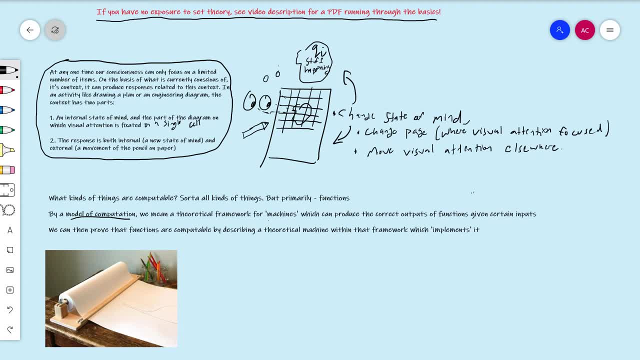 There's something going on in my head and I'm going to react to that. Based on what? Based on what I see and based on what's in my head, my state of mind is going to change. So the thing in my head is: I'm going to change my state of mind. 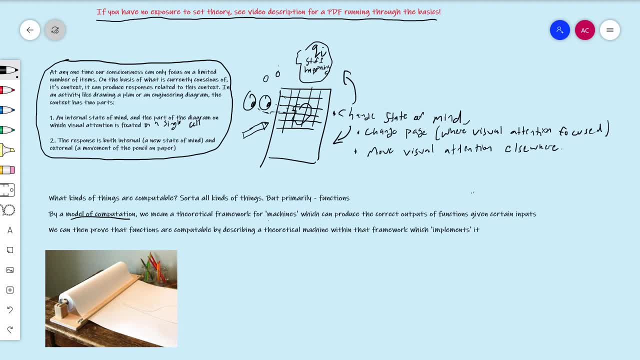 I'm going to change what's at the point that I'm looking at on the page My. you know the response. that's the internal, or, sorry, that's the external response. So the internal response is the new state of mind. 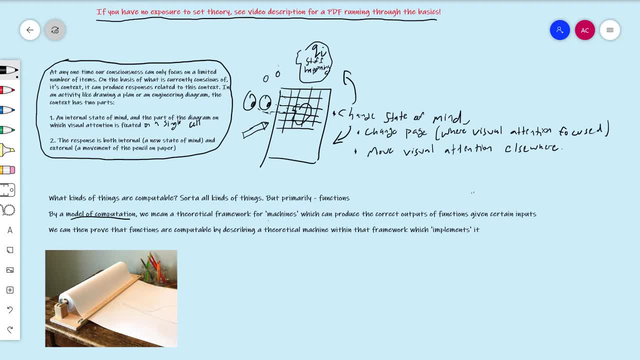 The external response is: I'm going to change maybe- maybe not- the place on the page that I'm looking, And then I'm going to move my attention somewhere else, And then the process is going to repeat itself. Now I'm going to be looking, maybe over here. 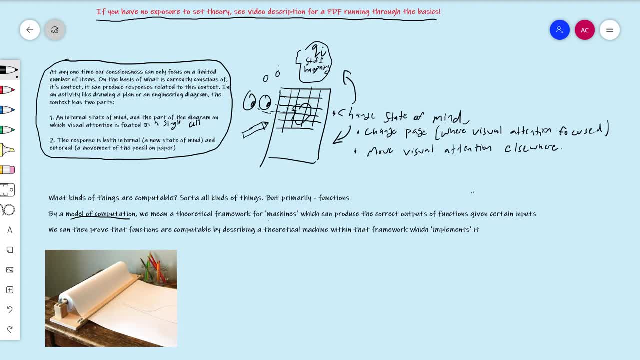 Actually, let me pause the video. I think I just remembered that it's not recording my cursor and I'm using my cursor to point at things. Okay, you should be able to see my cursor now. So effectively, you know once my state. so I'm looking somewhere. I have a state of mind. 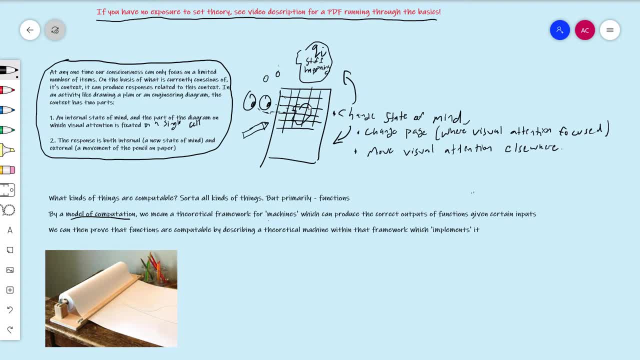 And then, based on those two things, based on what I'm seeing- not where I'm looking, but what I'm seeing- that's going to end up being important- My state of mind is going to change. I'm going to change. 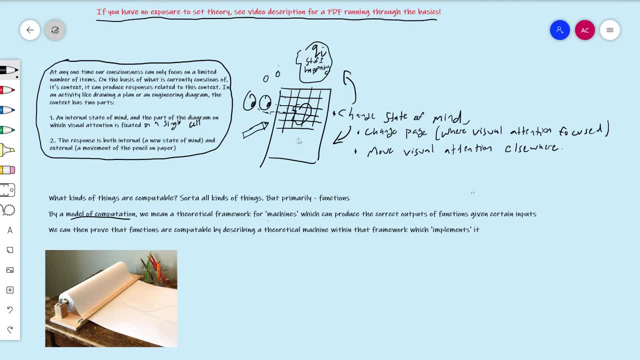 I'm going to use my pencil to change what I see, And then I'm going to change where I'm looking and I'll maybe be looking somewhere else. So maybe at that point I'll be looking over here and my state of mind will be different. 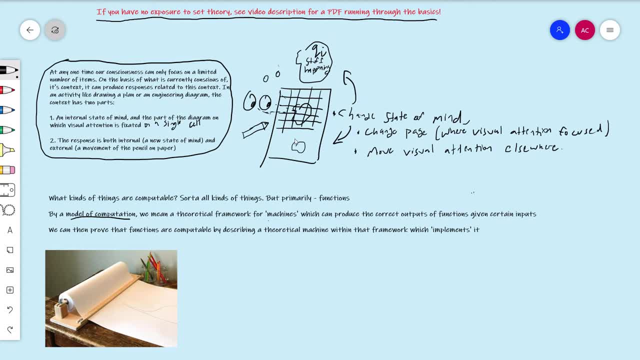 And then the process will repeat itself And then it'll just go like that. That's the loop, you know, and we'll have to add a marker, kind of informally to say when I'm done, It's sort of you know, that'll have to be defined. 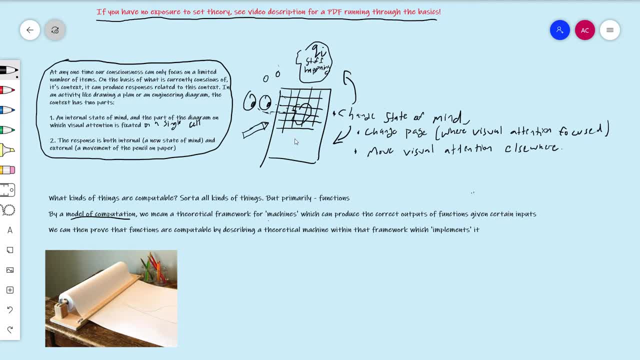 But that's the idea, That's the model for human thought, And what we're going to do is we're going to formalize this, And you can see I already sort of started the process by turning the paper that we're looking at into graph paper. 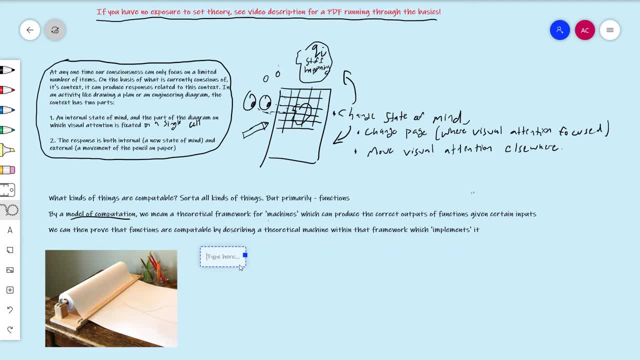 Okay, so what I want to start with is the process of formalization of this informal model. It's going to be: first of all, we need to make some assumptions in order to mechanize what I just finished describing. So I'm going to say this is a fundamental assumptions toward mechanization. 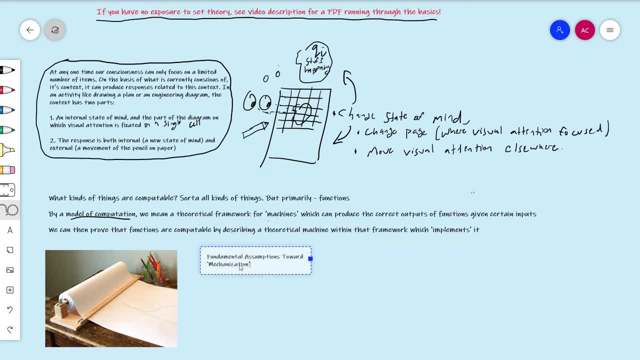 Toward mechanization. We want to make this process feel mechanical enough that we can mathematize it. Okay, so the first assumption I'm going to make is what I already sort of drew- Is that the paper is graph paper. I'll make this a bulleted list. 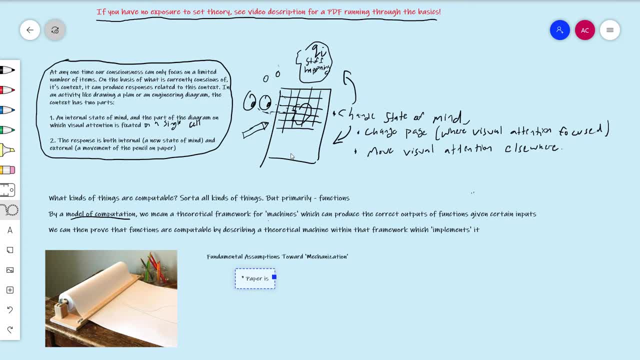 Paper is graph paper And the reason I want to do that is sort of obvious, right? I want to be able to tell you know it has to do with where my visual attention is focused and where it's going to change. If I have graph paper, then I can be precise about saying where I'm looking. 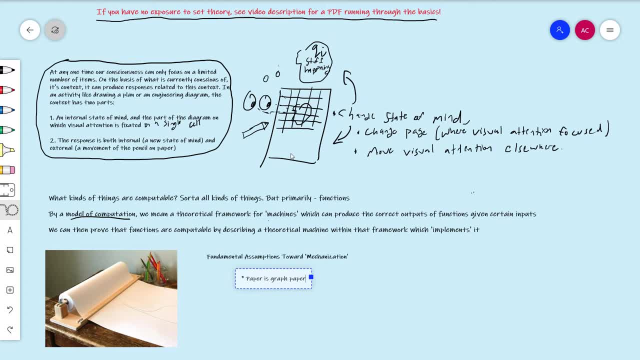 And I can also be precise about saying where I move. where my visual attention moves, It moves here. Specifically, there's no in between here and here and that's fine. I think everybody intuitively will understand that that's fine. That doesn't really lose me anything, because if you just look at this curve I drew here, you'll you'll know very clear. 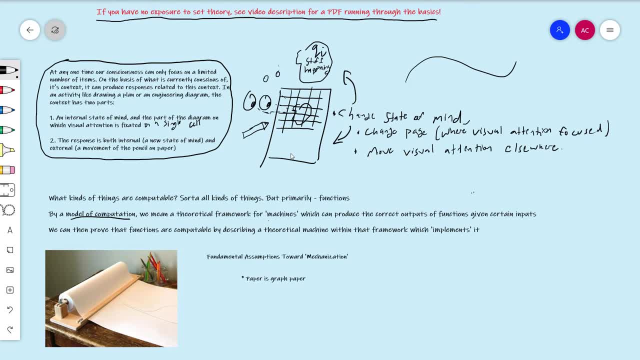 Everyone knows. this is not actually a curve, right? This is this. this screen that you're looking at is a pixelized grid. It is a. it is graph paper that you're looking at. It's just so fine that the squares are so small that it looks like a curve. 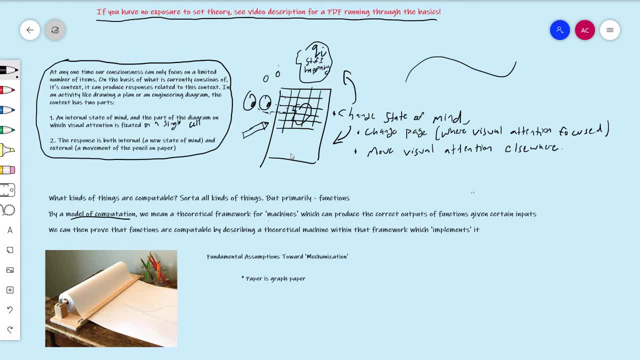 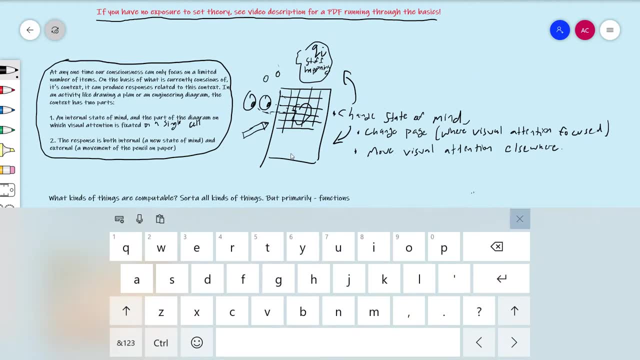 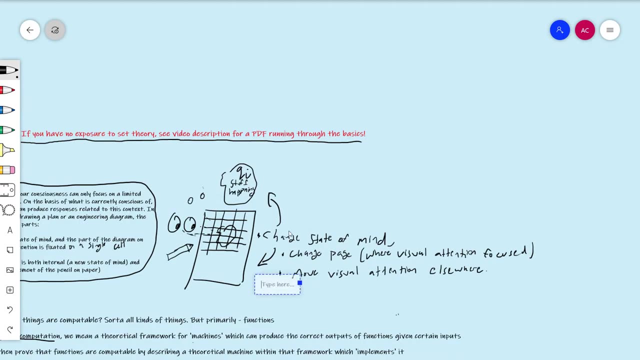 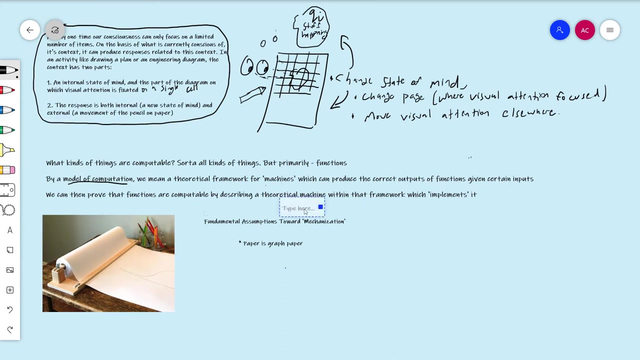 So just in that kind of based on that intuition, Okay, I think it should be clear that you're not really losing anything by sort of discretizing the paper. You're just being, you're just whoops. So. so that's our first assumption and that's what you know. that should give you a feel of what I'm going to be doing here in terms of what we're trying to do, in terms of mechanizing what I mean by the word mechanization. 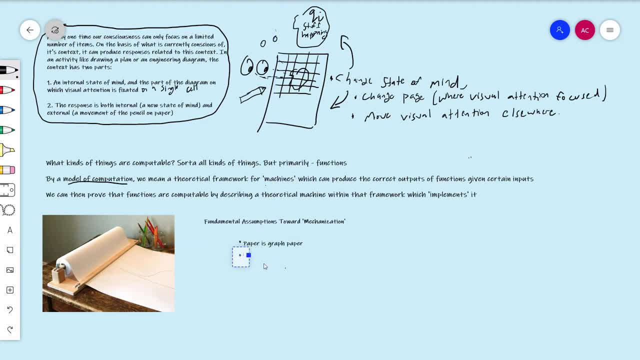 The next. the next assumption is has to do with this picture I drew over here. How much graph paper do we have? well, we're going to assume that we have as much as we want. so graph paper extends infinitely left and right, left or right. so, as you can see here, this is kind of the picture to visualize, right? 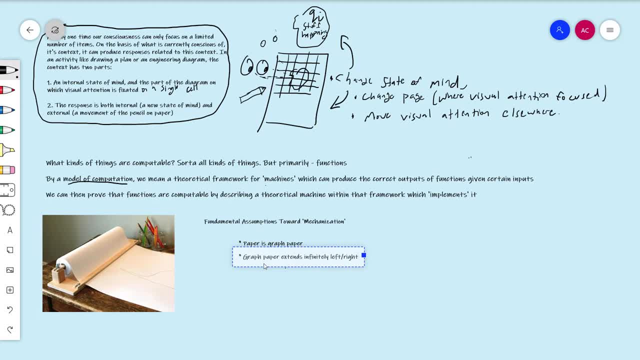 We just have. you know, I can just keep moving. I have infinite paper. but even beyond that, we want to be a little more precise. What do I mean by having as much paper as we want? It means I have one infinitely long strip of paper. 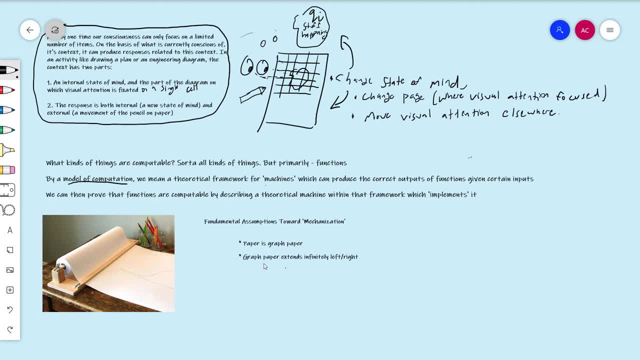 That's kind of what I mean. So this is the picture I had. I can kind of- you can kind of- think about it as, like you know, construction paper that gets wheeled out like this, You know, when I say infinitely left, right, 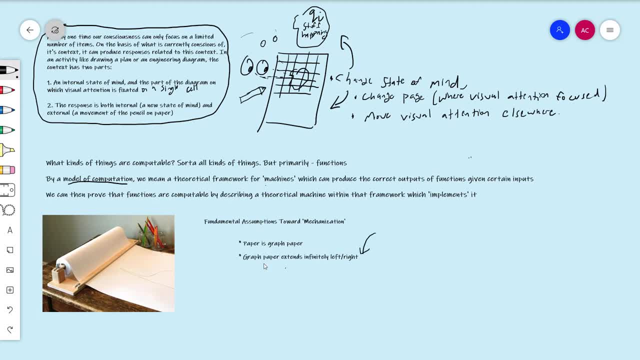 You know, I want to add the caveat. We're going to say some various things, usually both, usually both ways, But but it doesn't really matter as well. You know, one of the one of the things will prove That we just needed to be infinitely in one direction. but, but usually but. the standard model, I think, usually ends up being that the graph paper goes infinitely in both directions. 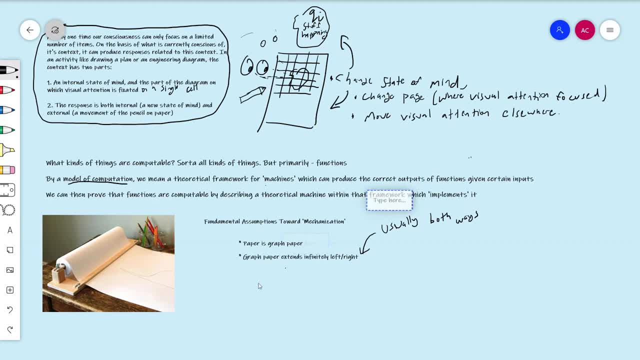 But more importantly, or just as importantly, is that it's going to be finite, though in terms of not not infinite in the up-down right. So we do have you know, we're going to have infinite in the up-down and we're going to have infinite in the up-down, and we're going to have infinite in the up-down and we're going to have infinite in the up-down right. 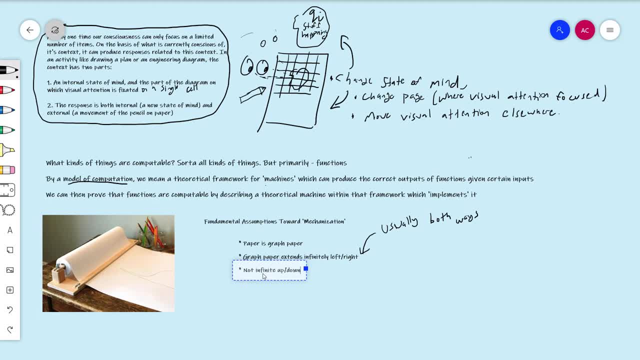 So we do have. we only have a certain number of rows on the graph paper. we have infinitely many columns, but we only have a certain number of rows, And that's just to kind of simplify what we mean by infinite we have, we still have as much paper as we want. we still have as much room for writing things down as we want. 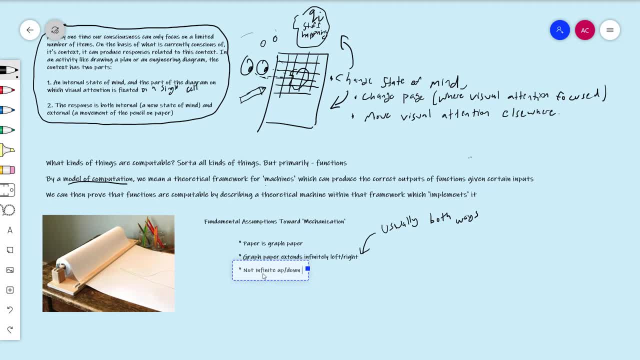 So there's no reason to give ourselves infinite, infinite rows. it's going to be simpler of a model to not do that and we aren't losing anything. So it's not an infinite in the up-down. we're going to prove that the number of rows really doesn't change very much. 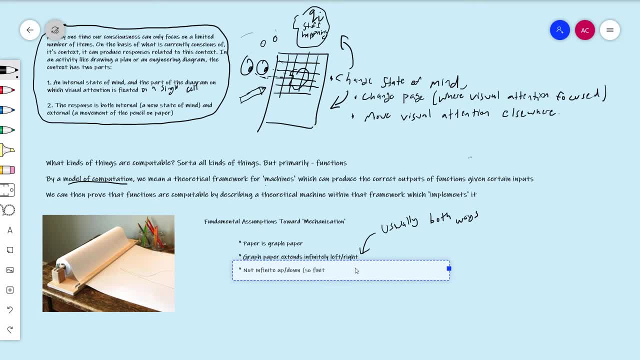 But so finite number of rows. Usually the number of rows will be one. So for the standard model- maybe I'll write that here- Usually just one row And so, and you know, at that point it's barely even graph paper at that point. 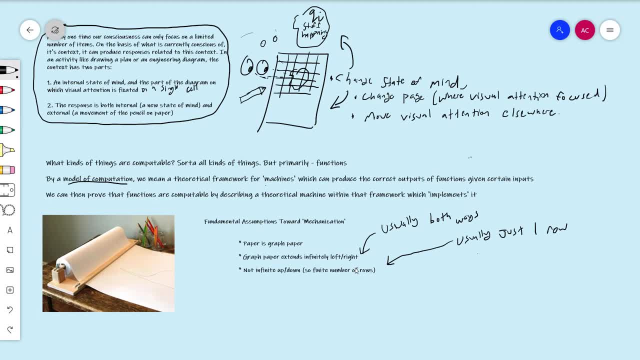 This is why you might be surprised that I say the word graph paper. The word that you usually hear is graph paper. The word that you usually hear when you're talking about Turing machines is tape. right, If you only have a single row of graph paper, it barely looks like, instead of having a graph paper at all. what we kind of have now is this like strip that goes infinitely in both directions, sometimes just one direction- and then we have a bunch of cells that have things in them. 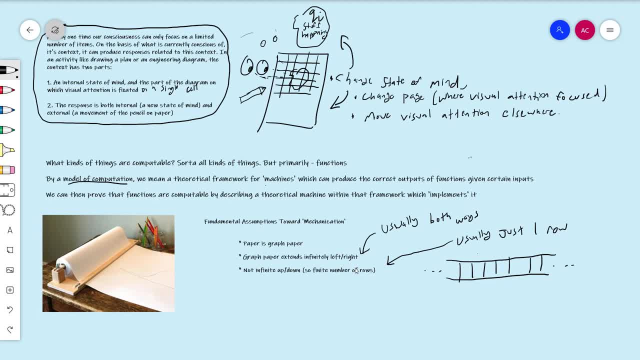 But it is built on. but we got here from kind of starting with this idea of graph paper And you can give yourself extra rows. You know it's often useful when you're designing Turing machines to accomplish specific things, to have an extra row. 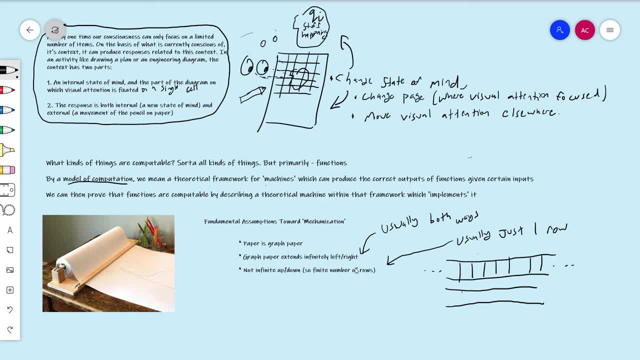 But even then, since we sort of lost at that point the idea that we have graph paper. usually people draw multiple strips of tape that are disconnected and then you lose all manner of having it be graph paper in the first place, But the bottom line is that you only have finitely many rows, usually one. 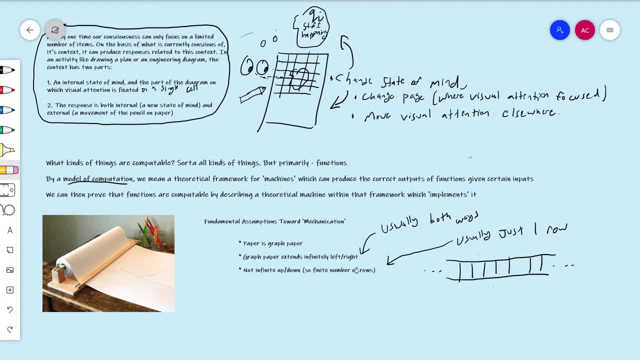 And at that point it stops being graph paper, sort of Other assumptions, what just happened. Other assumptions where you know I said visual attention is focused somewhere, well, where, how? you know what it would. you know, can my visual attention be the whole page? can my visual attention be four cells at once? 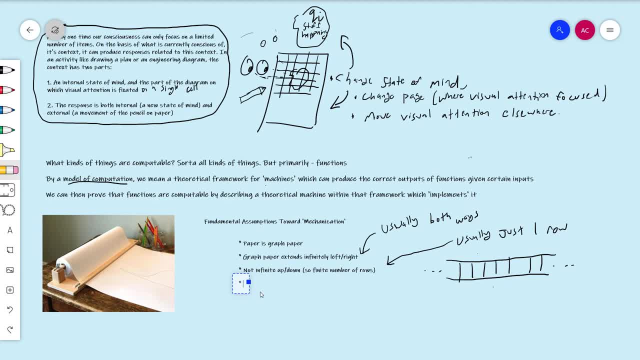 No, we're going to standardize things by saying that visual attention is focused on a single cell, one cell at a time. So at any one point, my visual attention is just a single one. One of these guys? Whoops, no. 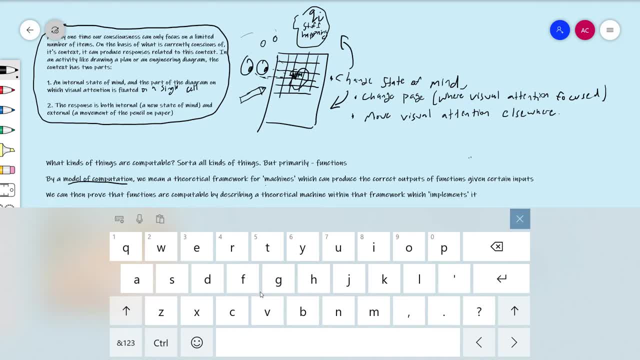 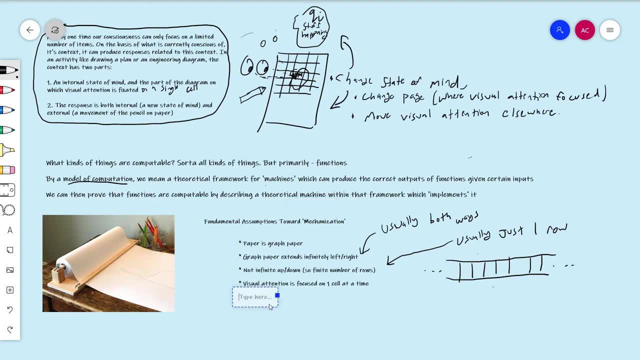 Just a single one of these guys. What else? Visual attention can only move. So now let's think about my visual attention after one step is going to move elsewhere. But we're going to say, to simplify things or to mechanize the process, and this will also give us a. this will also help us when we're talking about space. 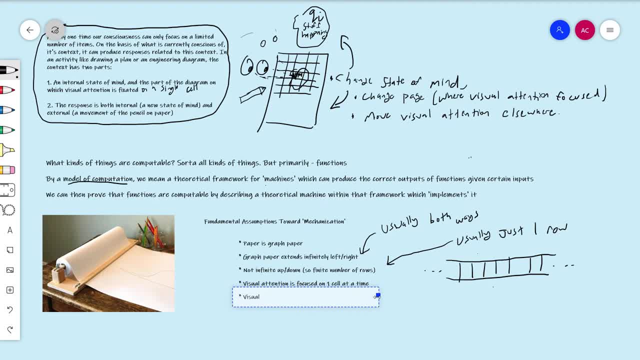 complexity later is that visual attention in one step can only move to an adjacent cell. How do I say that Visual attention on next step? Well, let me say it like this: Visual attention can only move one cell at a time, So it's focused on one cell at a time, and then, in the next step, I'm guaranteed to be So. 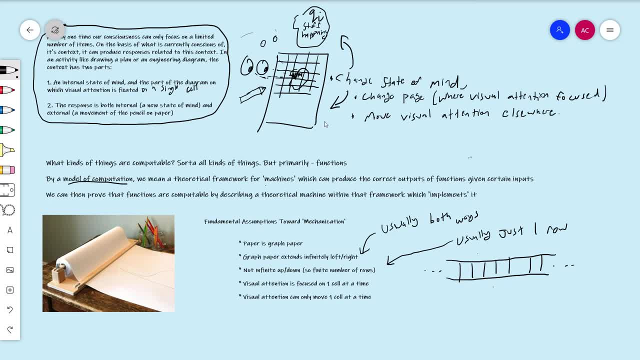 you know. going back to the graph paper, Well, if I'm here, I'll just say it like this: you know, if my visual attention is here, then my visual attention on the next step is focused on one cell at a time, and then, on the next step, I'm guaranteed to be. 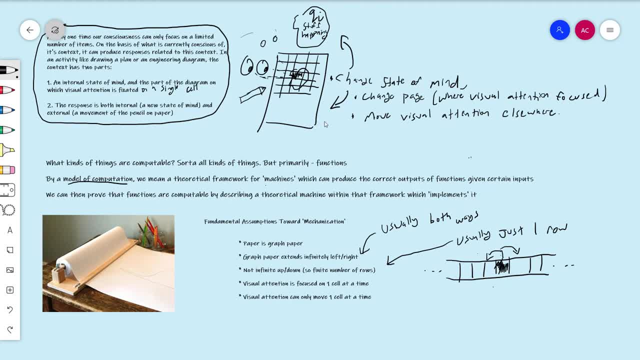 The next step will either be here or here, or here and nowhere else. So we're kind of mechanizing. you know what? We're kind of mechanizing this thought process. right, We started with a very kind of fluid idea of a human being at a page. 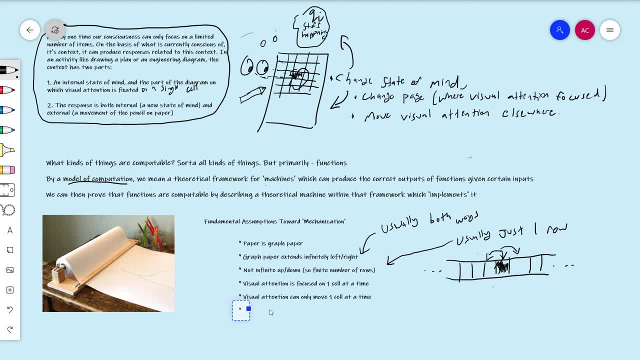 and we're sort of turning this into a robot. What else Let's see. Now we need to talk about states of mind, right? So we had the three fundamental components of our model for human thought was mind, pen and paper, right? So we've talked a little bit about. 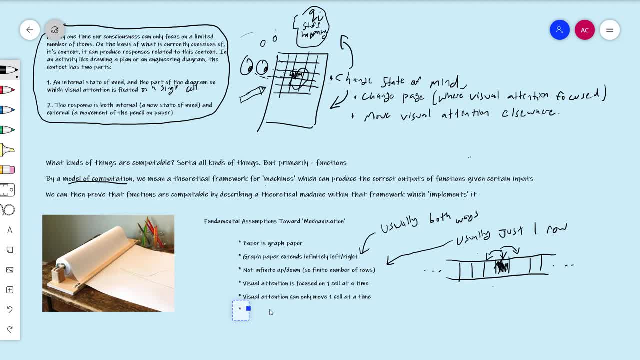 where our eyes are. but states of mind, we're going to assume that they're finite. So number of states of mind, number of possible states of mind, is finite. It's going to vary from Turing machine to Turing machine, but it's finite. It's kind of a resource. 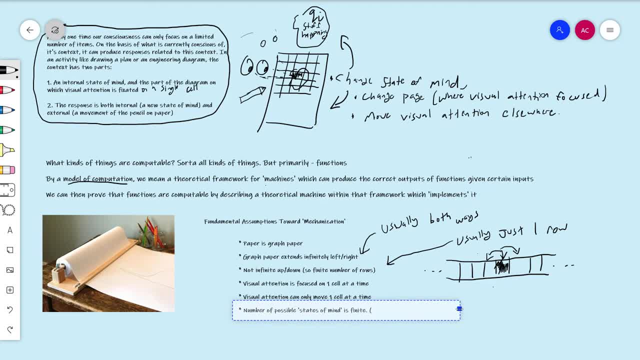 And also one state of mind at a time. So basically, in other words- And it's going to vary from Turing machine to Turing machine, I can divide My Turing machine is going to involve, you know, for the situation it can involve. 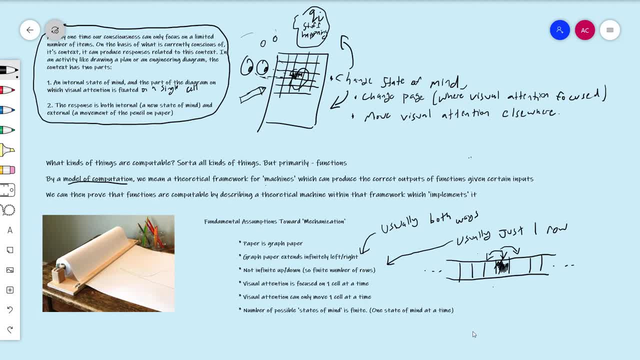 however many states I want, but it has to be a finite number, And so, typically, we're going to use: Q equals Q0,, Q0,, Q1,, Q2, dot, dot, dot Qn. This is our set of states. 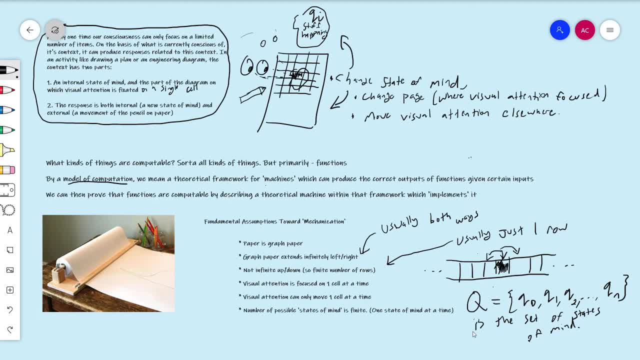 The number of states in a Turing machine is usually the part that gets people conceptually mixed up the most in my experience. But maybe to help you think about it, this is something I thought about pretty recently myself. What does it mean to have more states? 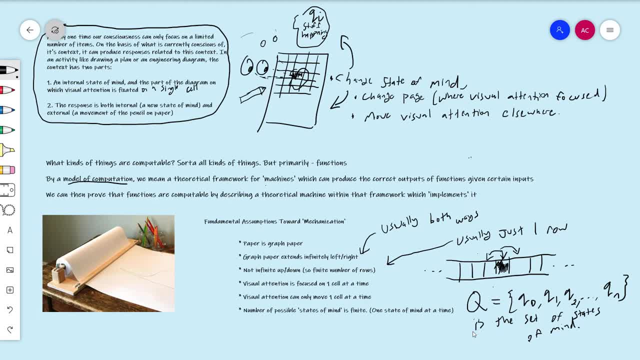 Suppose that my brain does like something regularly. Suppose I need to like: add numbers in my head right. That's a computation. We can think about this: What happens when I give a Turing machine lots and lots of states? If a Turing machine has tons and tons of states to work with, 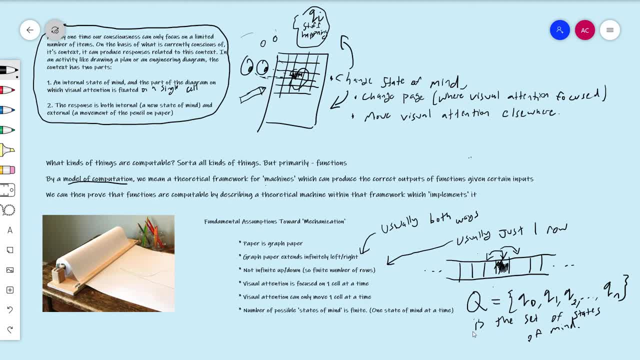 if you have lots of different states to work with, then that sort of indicates how smart you are. in a limited, kind of restricted sense, The size of Q is in some sense a measure of intelligence, because- think about it like this- The more states that you have. 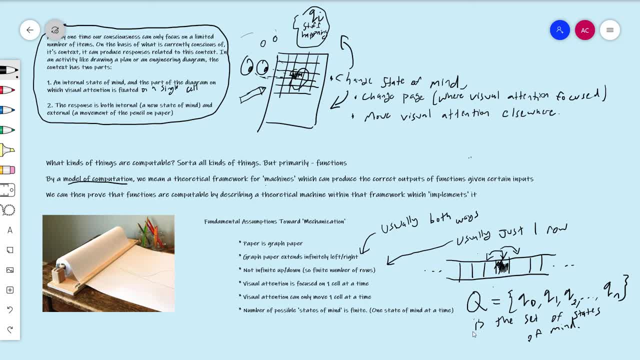 the more things you can do in your head without you know. if I have like, suppose you know. if I have a state in my head for every like possible addition of two numbers that's only a single digit, then I can do those in my head without actually doing any work on the. 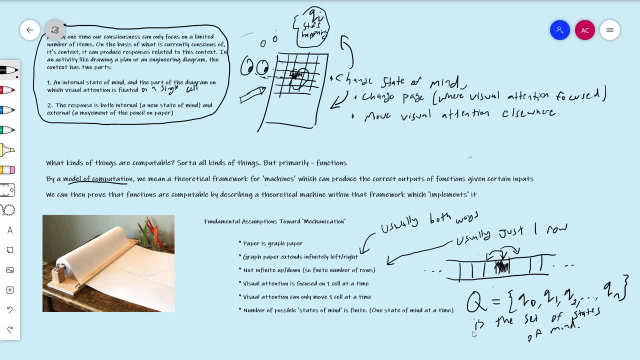 paper. So and the idea is that the more states you have, the less work you have to do on your paper, In other words, the more things you can do in your head. So you know if you're talking to somebody that can, you know, take square roots of large numbers in their head really fast. 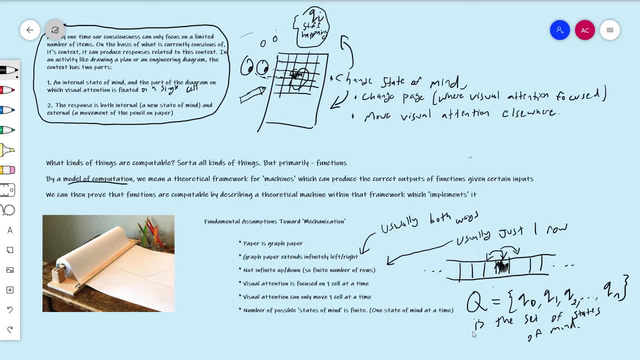 or do any of those mechanical nerd things that are impressive to people. you can sort of model that in our model by saying he has a lot of states. The number of states of mind that he had he can cycle through is big, is a big amount. 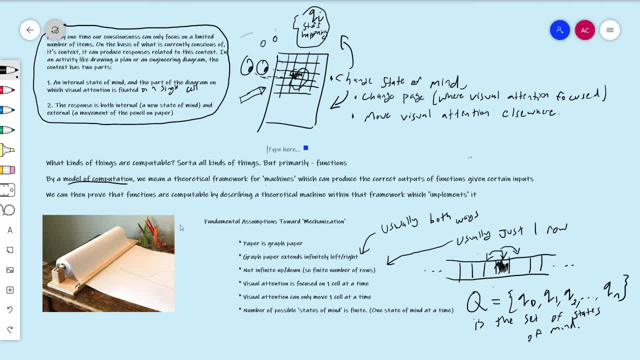 So maybe we'll talk more about that in the future, But we're going to assume the number of states, no matter what, is always going to be finite. What else We have to talk about? what symbols are allowed to be on the page? 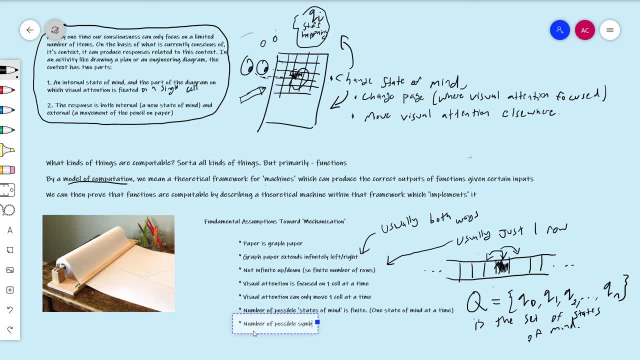 Number of possible symbols that can be written is finite, And so at this point we're sort of talking about the language that he's using to write on the page, Or, to be a little more precise, we're talking about the alphabet. 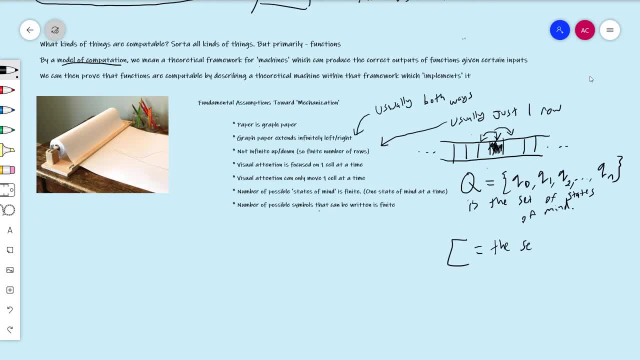 I guess I'm sort of out of space. I have to move the set of symbols. This is a capital sigma And we call it an alphabet. This is sort of yeah. so I mean, you know, sometimes, you know, the typical alphabet that you use is a combination of like: 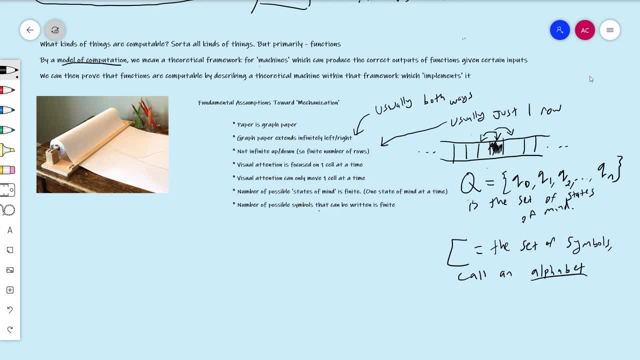 the. you know the English alphabet, Greek letters, digits, But it's a finite set- ASCII, you know, And this is going to vary from Turing machine to Turing machine 2.. But what we will show is that it doesn't really matter, in the same sense that the number of rows doesn't matter. It doesn't really. 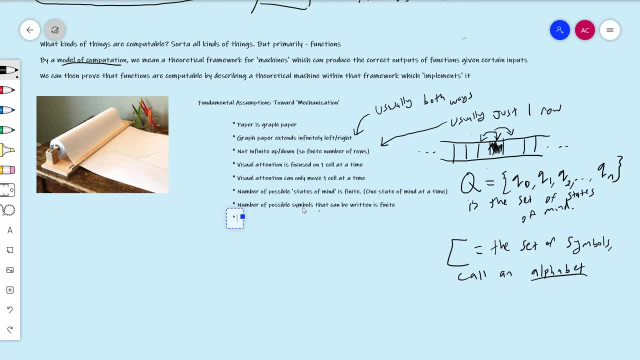 change anything. What we'll show that you, we will show that there's a minimal number of states that you need or a number of symbols. The minimum number of symbols that are that are needed for every Turing machine, For Turing machine model of Turing machines that can do everything, is two. You always need at least two symbols. 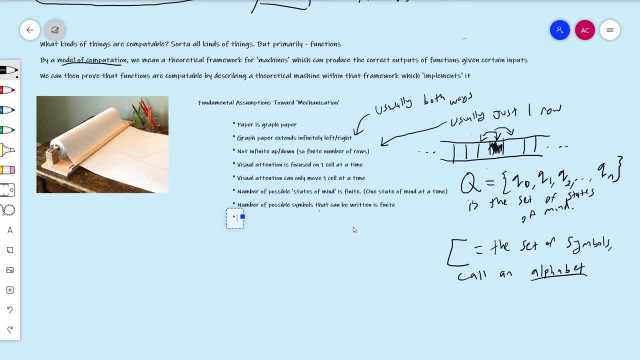 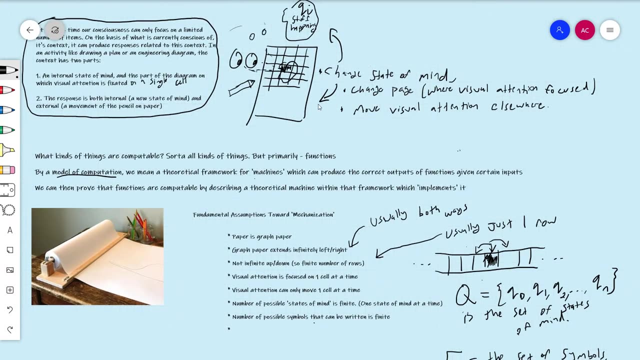 that's the simplest kind of Turing machine And anything else. Okay, one more thing In a single step. what can happen? So let's look back up here. So, in a single step, what am I allowed to do in terms of writing things down? 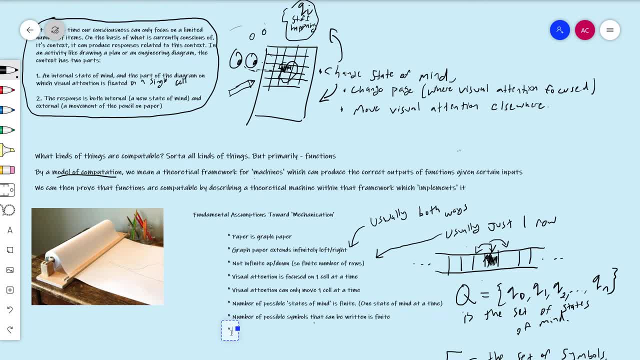 Well, what I'm going to be allowed to do is only the cell that's being looked at will be allowed to be edited In a single step, only allowed to edit. So I mean, this is going to be the external response. So the external response is going to be limited to. 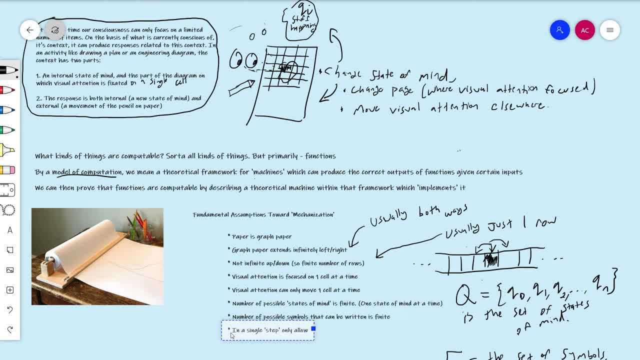 only being able to edit the chain, I'm only allowed to edit the symbol that I'm staring at. So, in a single step, only allowed to edit, to change the symbol in the cell where visual attention is focused. So, again, my state of mind is going to change. 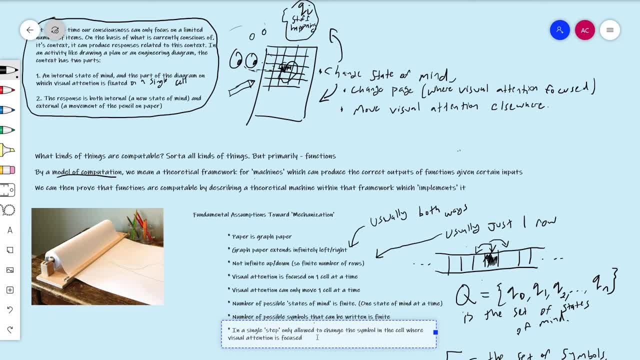 although it's finite and it can, but the state of mind can be anything, Yeah, so maybe I'll add a second thing: State of mind, any state can change. states can change into whatever other states. I'll just say: states can change, however, And I think that's all of the assumptions that we need. 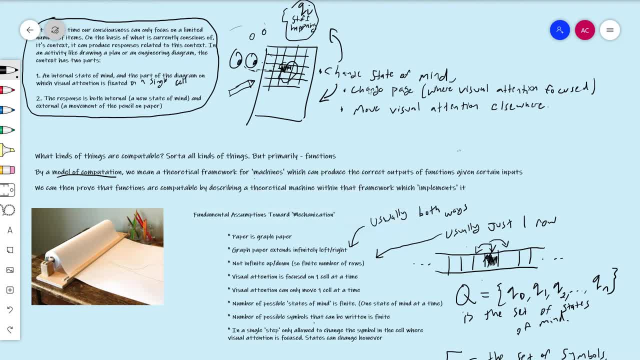 towards like mechanizing, So let's go over them. So we started out with this fluid process where I'm staring at a page, I'm staring at a particular place, I'm thinking about something in particular and then, based on those two things, what I'm seeing- not where I'm looking, but what I'm seeing. 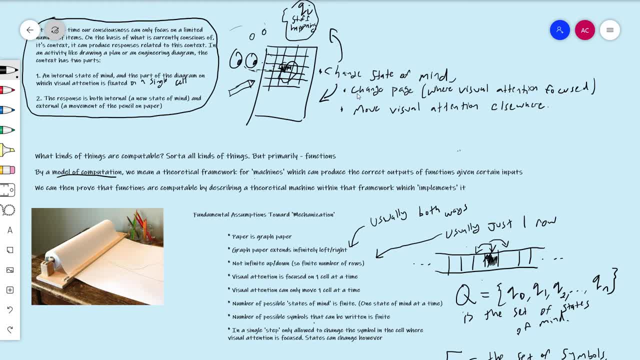 and also based on what's in my head. what's in my head is what is going to change, as well as the symbol that I'm looking at on the page, And it's only one symbol at a time. That's part of the 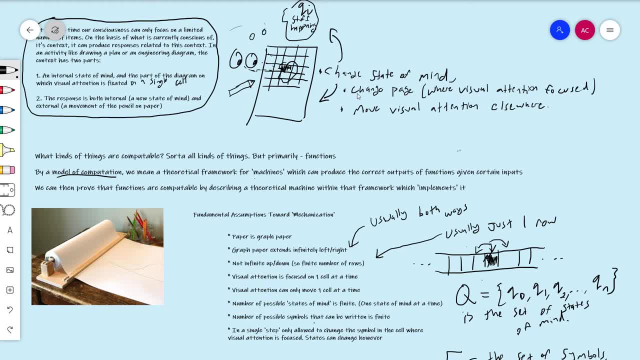 mechanization process. And then we mechanize this by saying, okay, the paper is graph paper, the paper extends infinitely left and right, but only one, but usually only one row. Our visual attention is going to be focused on one cell of the paper at a time. 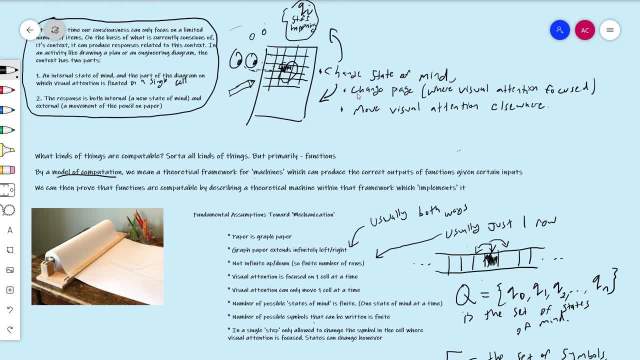 and obviously, one cell of the paper can only have one symbol. The number of symbols is finite. The number of states of mind is also finite, but can be as big as we want it to be, and in a single step. the internal response is going to be the change from one of these q's. 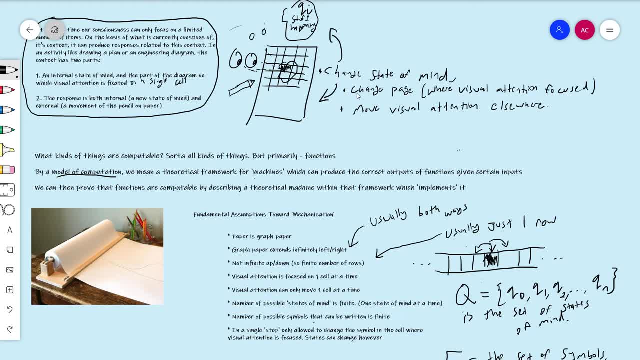 to some other q, one of these states to some other state, doesn't really matter which one. I can go from q to q, 1 to q5 or whatever, and i'm allowed to change the symbol that i'm looking at into any other symbol. 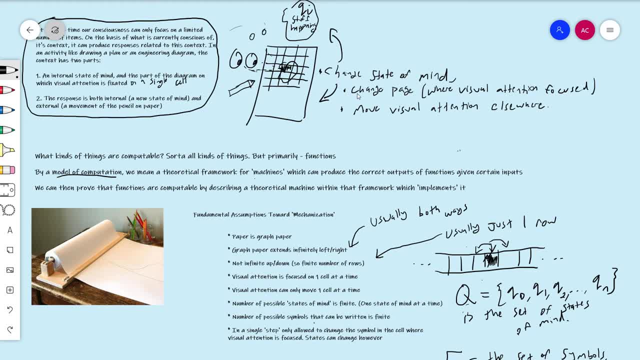 including the symbol i had before. that would be basically doing nothing, or i could erase it. we're going to have a symbol for a blank um, but i can only change that one cell and then my visual attention is going to focus, refocus elsewhere, but it can only focus, refocus to an adjacent cell. 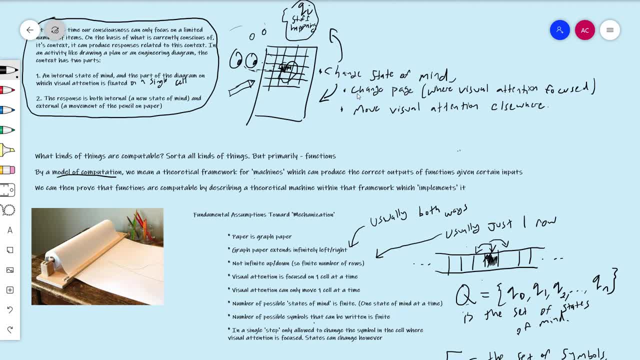 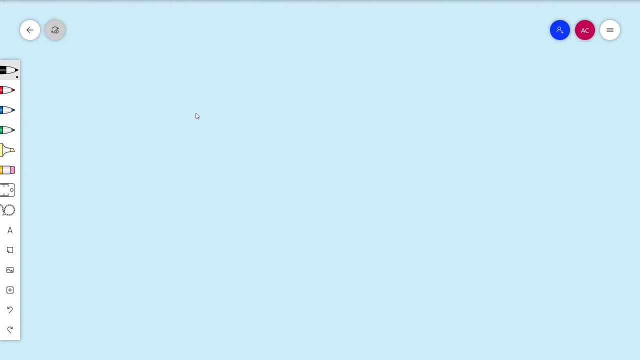 so through all of that we have, we've made a large step towards mathematizing this model for human thought and human information, human processing, i suppose all right. so now that we've sort of mechanized the idea, we've started with an informal idea for a model and then we sort of mechanize that model and then we now know enough about what we. 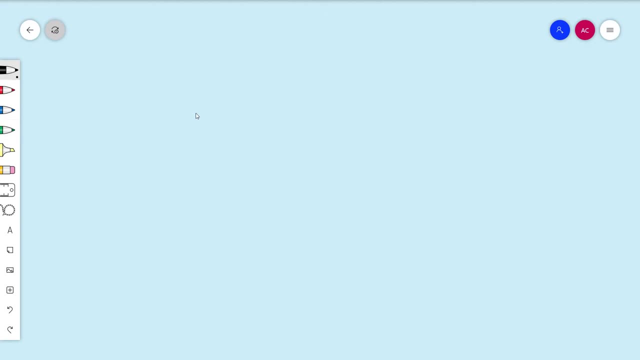 want to do that. we're sort of ready to finally write down a full-on mathematical definition of a turing machine. so a turing machine is a kind of object. what kind of object is it is going to be? a turing machine is going to be a kind of object. what kind of object is it is going to be? 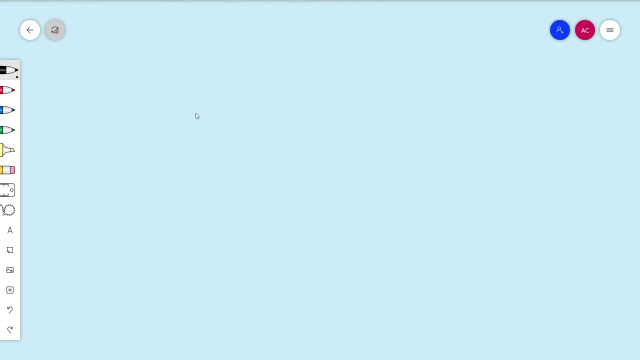 characterized by three things. um, turing machines- whoa, this is a little thick, let me. so turing machines involve three sets, involve two sets and a function. so, on the one hand, you have sigma- that's the worst sigma- the alphabet set of symbols, which will usually be standard, standardized. 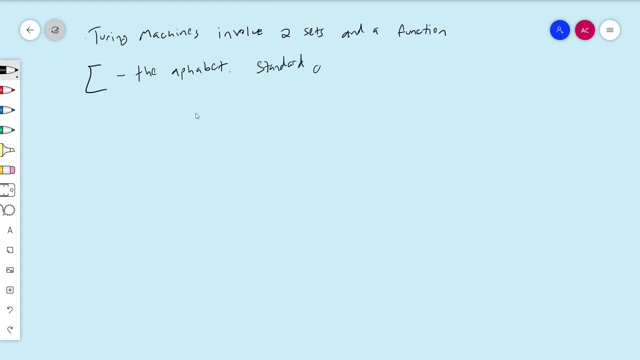 standard alphabet. uh, is this? the standard alphabet is going to involve zero and one, but then it's also going to involve this guy, this triangle thing which looks like a play button, and also this i'll use like a square, square u. this thing is going to be known as a start symbol. 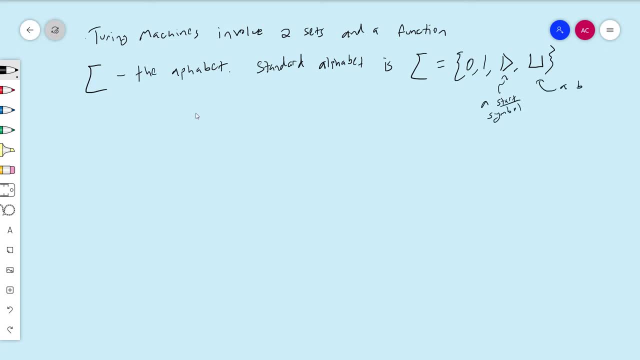 and this is a blank, and the idea is that we're not going to have a page in like the definition anywhere. we're instead going to have, um, the pages in our imagination, and so if the page is in our imagination, then we're going to have a page in our imagination. 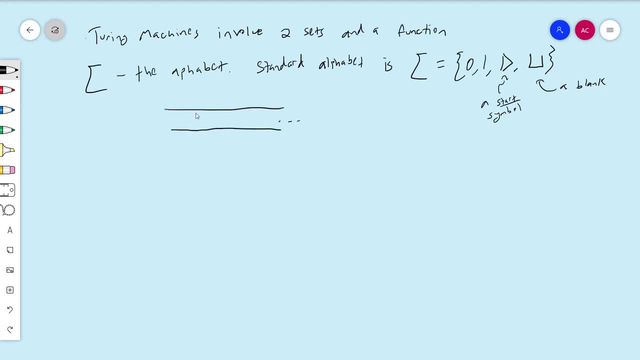 and i need a symbol to represent that the cell is blank. so this, right here, if i, if i have this, if i have the u symbol somewhere, then the interpretation is that that's a blank. so i need a symbol to say that i have a blank cell. i also want at least two numbers to be two, two. 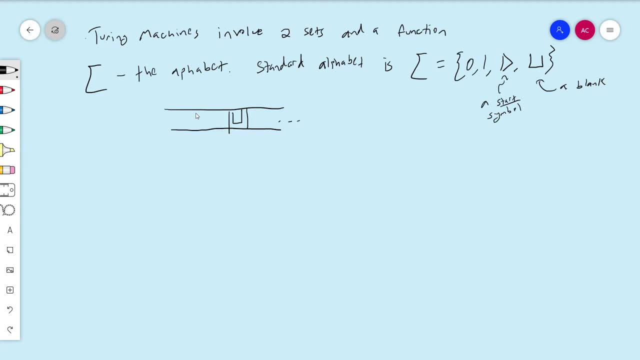 symbols that i can print on the cell, and then the start symbol basically indicates where, where my cursor is, where my focus is, so. so blanks represent blanks, and then a start symbol represents where attention is focused in the beginning of the computation. so that's the purpose of these two s special symbols and, in reality, like i said, the minimal. 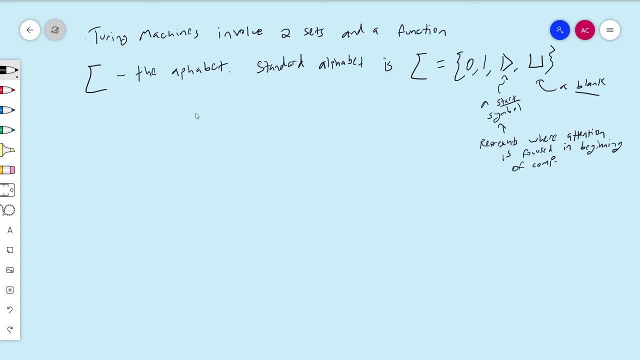 size of an alphabet is two symbols, um, so, in like the most primal form, a turing machine really just has a two, two symbol alphabet, zero and one binary. these, these things are here for our convenience. um, but this is kind of in terms of when i'm proving things about turing machines. 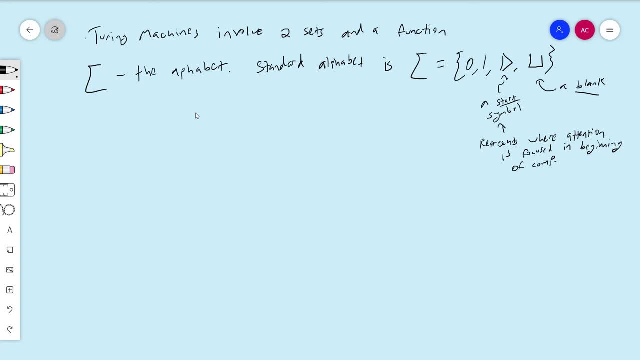 this is the alphabet i'm usually going to be using, but when you're doing turing machines- and i will assign you a few exercises in terms of make turing machines to do specific things- you can make the alphabet whatever you want. if you, if your alphabet, if you're trying to do something, 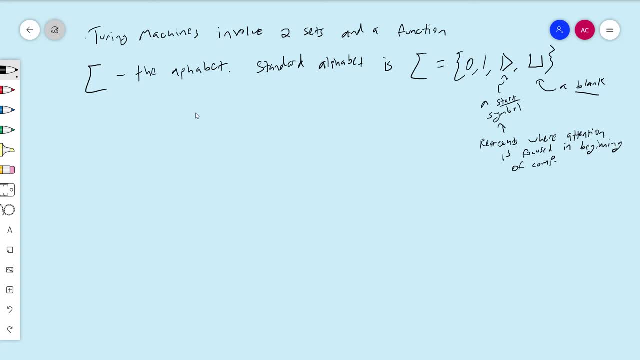 with numbers, with, like you know, numbers, then you can make your alphabet equal. you know zero through nine, right that? that would be your alphabet. if you're trying to do something with with numbers, then this would be your alphabet. if you're trying to do something with numbers and you want to write, 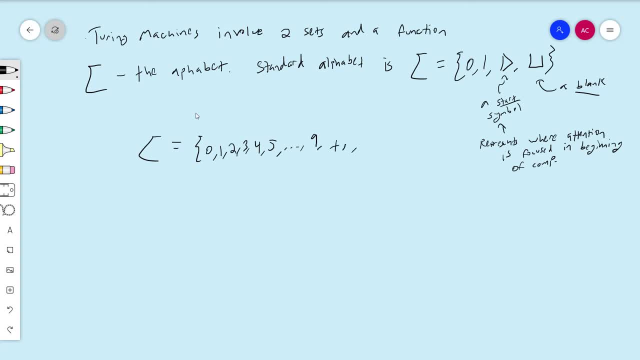 out expressions for some reason, like: add a plus sign, you do you. it can be whatever you want it to be, um, and, and sometimes, when i, i will do some examples, and, and for those examples i will use whatever alphabet is convenient, but i'm also going to prove to you that the alphabet is arbitrary. so 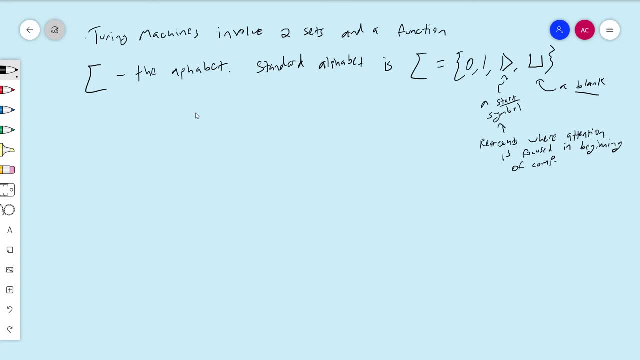 that that so that we can switch around, but this will be the most common one that we use. um, i'll use a two symbol alphabet, i think for exactly one proof, but it's a pretty important proof. um also, we've got that set of states and it's also important to note. you know, turing machines have two. 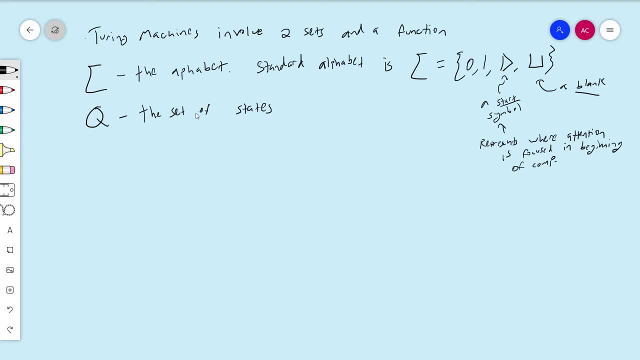 sets in a function. this thing is going to be fixed for all turing machines, the you know in our heads. there's going to be a standard model of computation and that standard copy model computation involves a fixed set of computation and it's going to be a fixed alphabet. but then there's tons of turing machines past that and 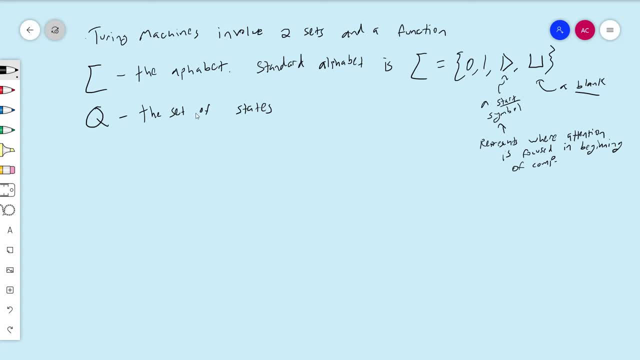 and this is going to be something that does fluctuate. um, there's no standard for the set of states. you you have as many states as you need, but it's important to note that it is sort of a resource: the more states that your turing machine uses, the more complicated your turing machine. 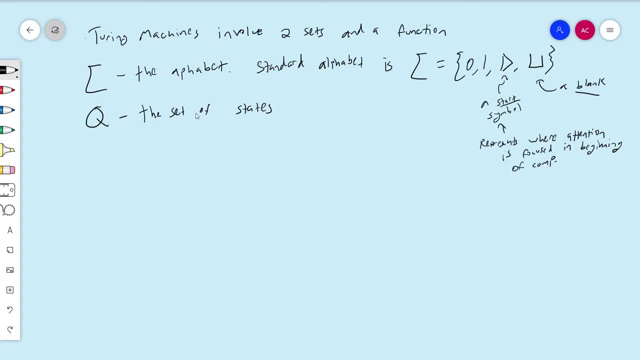 fundamentally is: um, so that's, that's that, and then finally, we have the function that tells us this. so what if we were to have state set pieces at a right example? for example, let's put it in a circle, and we're just going to decide is if we manage to have turves for a one- calculated the multiple of Nambo thanks. 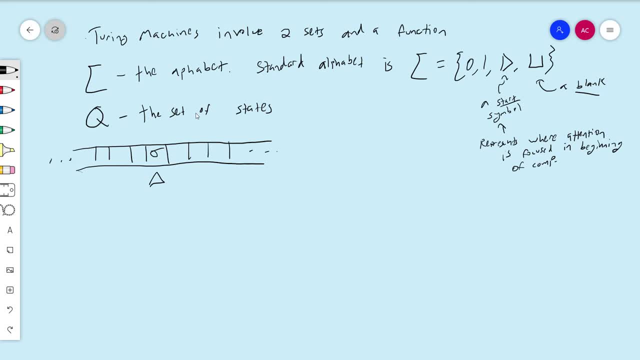 so i'm going to call this symbol. at any one point i'm going to be looking somewhere, so i'm going to be seeing some symbol- let's call it sigma- at the stuff i'm looking at a specific place, i'm in some specific state q, so at any time, 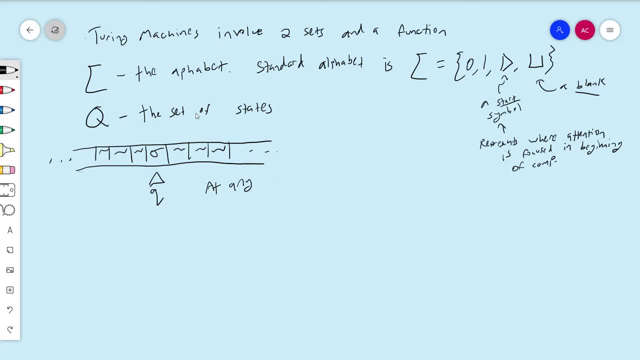 at any at any moment in time, looking at sigma, looking at the symbol sigma and then in state, q. so i have these two symbols, sigma and q, that dictate kind of everything that's going to happen is going to be dependent on these two symbols. and so what's going? 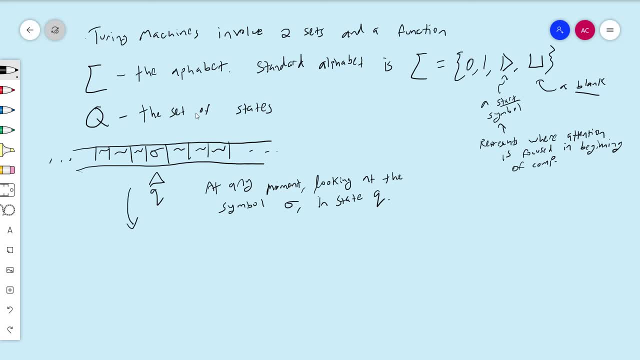 to happen is there's got to be a function, there's got to be an instruction telling me what to do, and we already know what's going to happen. i already kind of specified it. So what's going to happen is that, first of all, this is going to move either left or 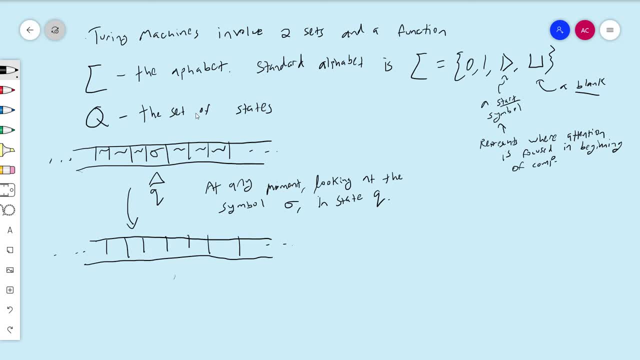 right or not at all. Let's just say it moves for the sake of argument. it's going to move here, so my visual attention will change, but only to one adjacent cell. It's going to change into a new q, so the state of mind will change. so it'll change. 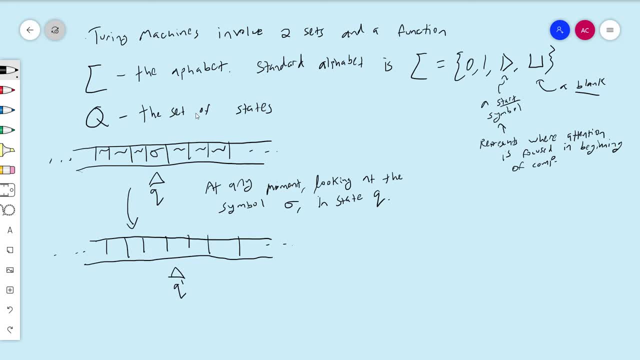 from q to q prime, and then this symbol here will have changed into a new symbol, sigma prime, And then I'll be focused on a new symbol on the next step, And so there's got to be a function. there's got to be a function that has all the information. 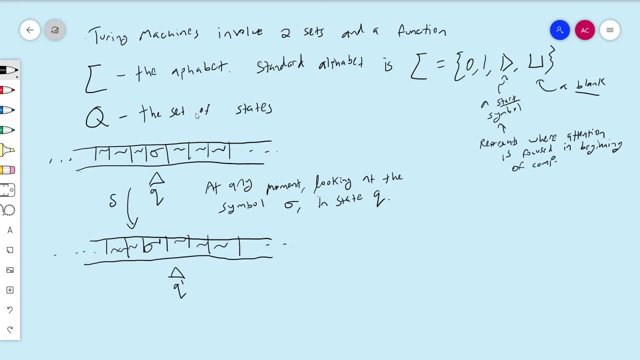 I need in order to do this step. I'm going to call that function delta, and delta is the transition function. The transition function of a Turing machine is basically the program. It tells you what to do given that you're in a specific state of mind: q and looking. 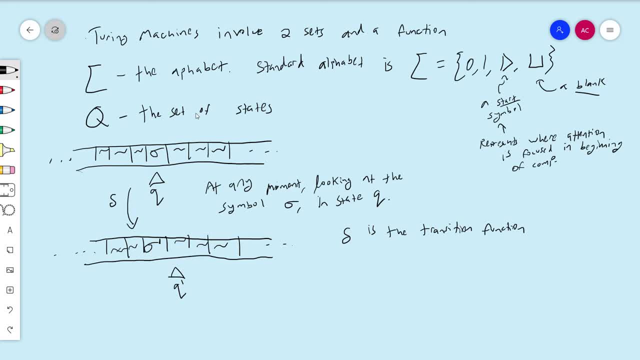 at a specific symbol, sigma, And what it does in the case of the picture I just drew here. it's a function. It's a function which takes as an input takes the pair sigma q and as output returns three things. 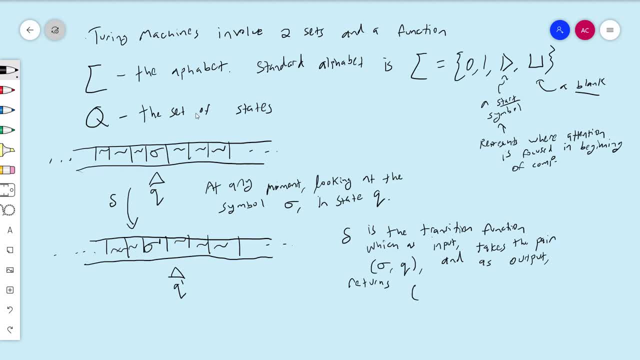 It returns three things. It returns, first of all, a new symbol that I want to replace the old one with a replacement symbol. It returns a new mental state that I'm supposed to go into And, finally, it has to return a direction. 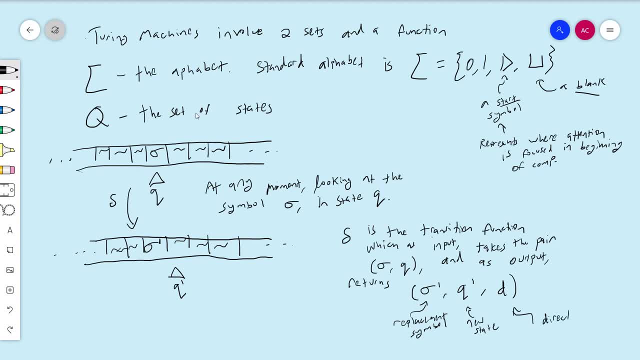 It has to return a direction, And the direction is only going to be one of three things, And those three things: if it moves right, I'm going to say negative, I'm going to say if it moves left, is an element of negative one, zero one where negative one implies move left. 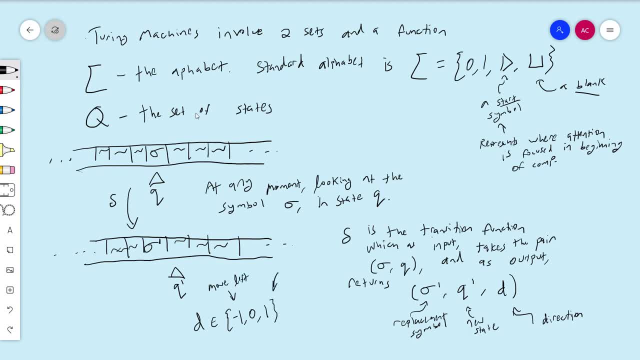 one implies move right. and then zero implies of course don't move. and this is an optional one. you don't lose any. your Turing machine doesn't lose anything with a with a don't move option. so just kind of like the start symbol and the and the blank symbol. 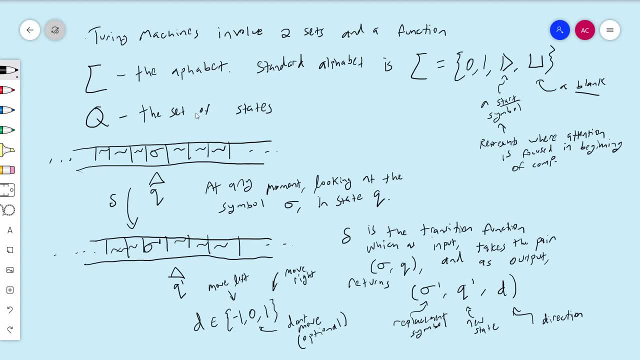 were arbitrary. I mean, we're not arbitrary, but there for convenience and not actually super necessary. the zero option, the option for not moving, is also something that's just there for our convenience. really, you just need to move left or move and move right option, but that's what. 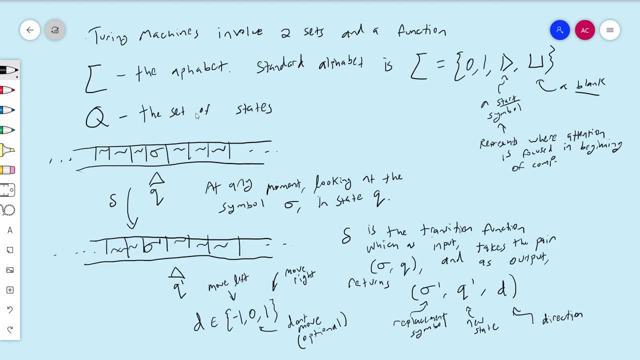 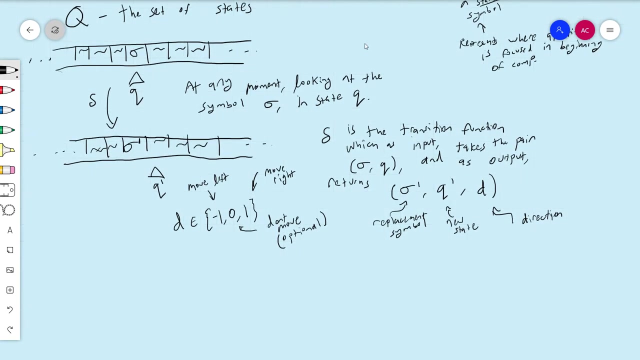 that's what the transition function fundamentally is. so you've got three, three characteristic kind of objects that together constitute theoretically a Turing machine: the alphabet, the set of states and the transition function. and the transition function, just to kind of you know, if you, if you're familiar with Cartesian products of sets, delta is a function that 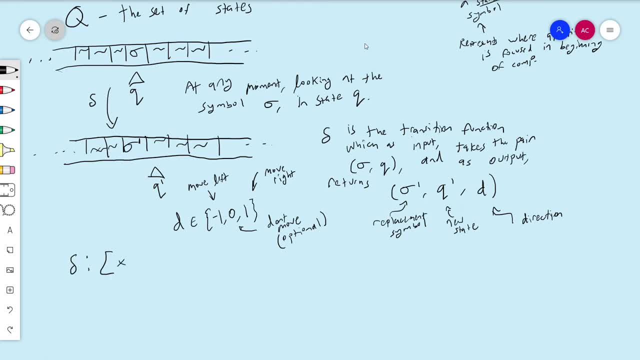 takes the product sigma cross q to the product sigma cross q, cross minus one, zero one, so that that's fundamentally the kind of object that delta is the transition function. it's a function that takes a pair, it takes a symbol and it takes a state and his output: it returns a new symbol, a new state and a direction to move. 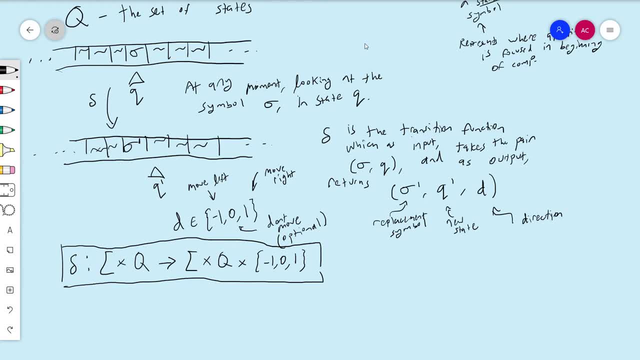 so that's the idea. now We're going and that's the syntax of a Turing machine. That's just the syntax. We still have to define the semantics. but let me summarize in a full-on definition what I just did, what I just said. So definition: 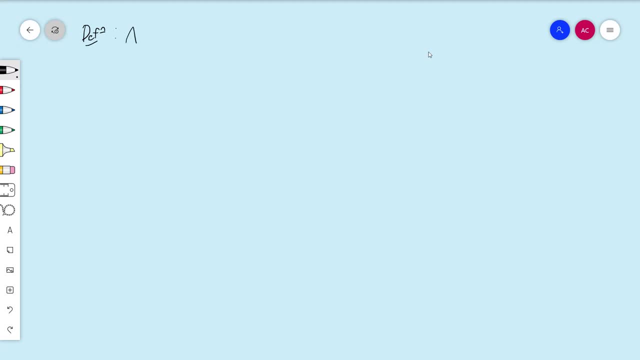 When I write D-E-F-N here, it means definition, A Turing machine, which I'm going to often abbreviate T-M is a triple, is a triplet of objects. It's a triplet, it's a pair, it's like a pair, but it's three things. It's a set sigma. 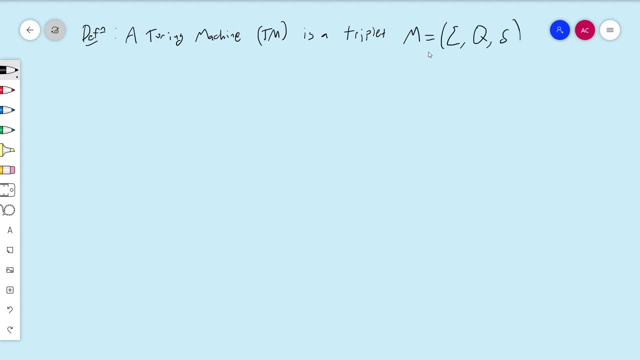 it's an alphabet, a set of states and a transition function where sigma is a finite alphabet, Q is a finite set of states and delta is a mapping. It's a function that takes sigma cross Q to sigma cross Q cross negative one, zero one. 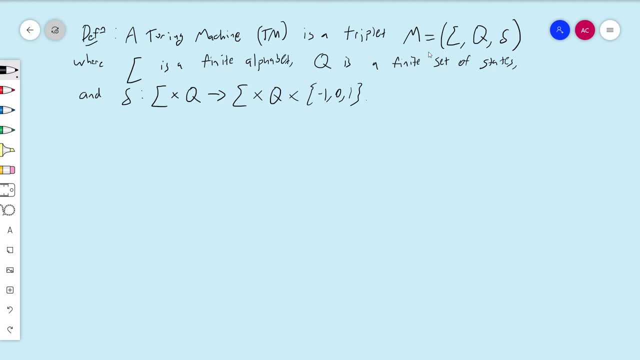 There's a few extra things I wanna say about what a Turing machine is kind of as a syntactical mathematical object. We're going to require a q equals Q, zero, Q one, dot, dot, dot, Q n. put n things in it. We're gonna always kind of imply that Q zero has some. 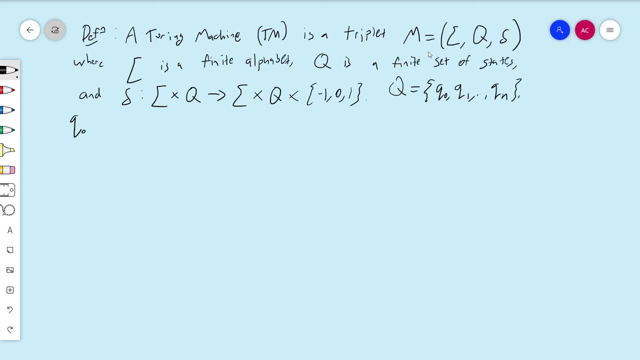 special meaning, q0 will be called, and sometimes I won't use q0, sometimes I'll use like qi if I want to, if it's more convenient to use q0 for something. q0, the first one, you know, there's. 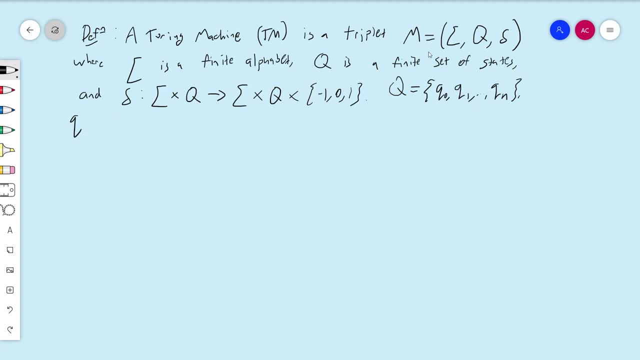 a special- let's say this- in q, we always have a special symbol, a special state: qi, which is the initial state. So this is going to be kind of the standard starting state, Usually q0.. And it's actually special states plural, because we're also going to have 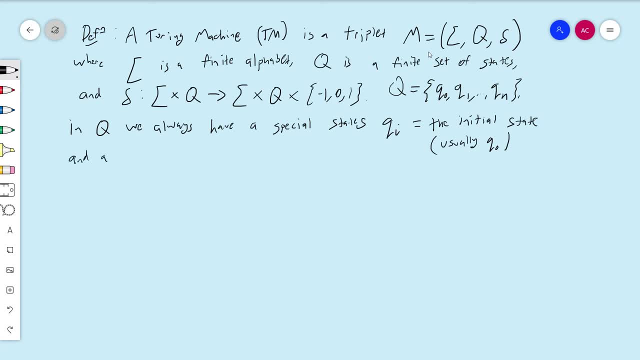 and qh, which is the halting state. Now we're going to have a halting state qh and usually that'll be the last state. But sometimes, like I said before, we're usually going to be interested in decision problems. 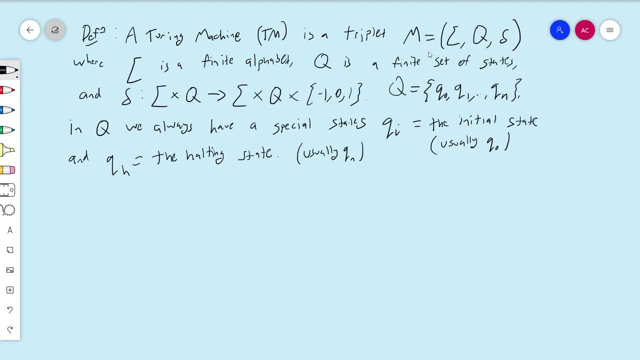 right Problems where the Turing machine is supposed to return a yes or a no And to indicate yes or no semantically. we could have it be the case that the Turing machine just erases everything and puts a 1 there and stops and halts and goes into the state qh. 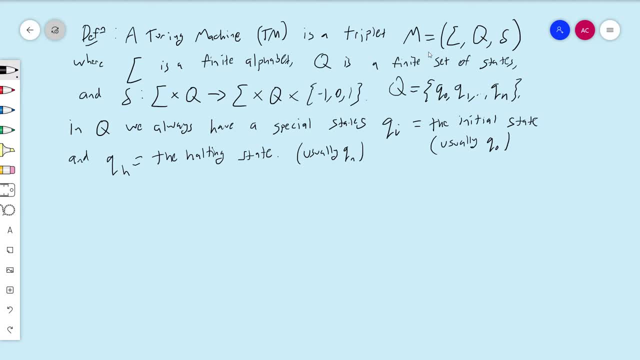 That would be one way to return a yes answer and zero for no answer, But to make our lives easier a lot of the time. instead of qh, we'll have, you know, qy and qn, which will you know, for accepting. 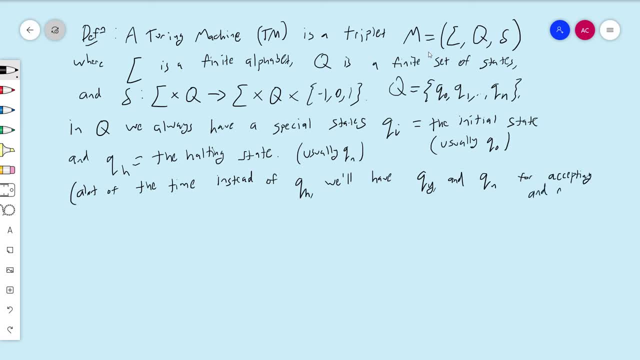 and rejecting respectively. So q yes will be like an accepting state, q no will be a halting state for yes and no respectively, And sometimes it'll be convenient, you know, to interpret the qy answer as an accepting state. 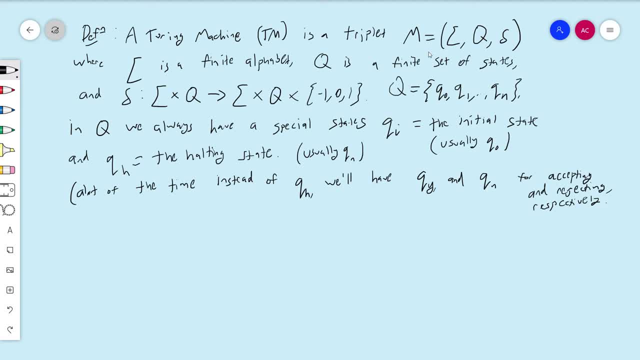 rather than program in delete everything and replace it with a one Again. that's just for convenience, but that'll be the interpretation. Sometimes we'll have one state for halting and sometimes we'll have two, depending on what we're doing with our Turing machine. 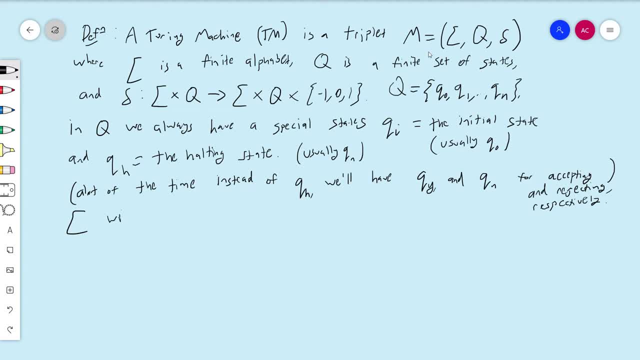 Also, sigma will usually have the play symbol and the blank symbol. The bottom line is that, just like queues, we'll kind of cheat sometimes in terms of what's going to be interpreted as the blank and what's going to be interpreted as the play symbol. 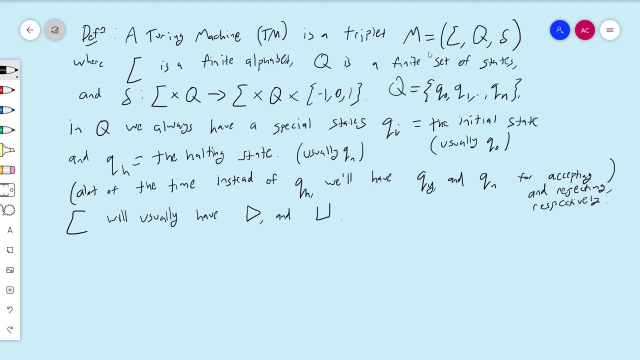 And technically, these are all you need. All you really need is a play symbol and a blank symbol. The blank can function also as just kind of arbitrary content somewhere. You can print these start symbols wherever you want, and I defined what those are. 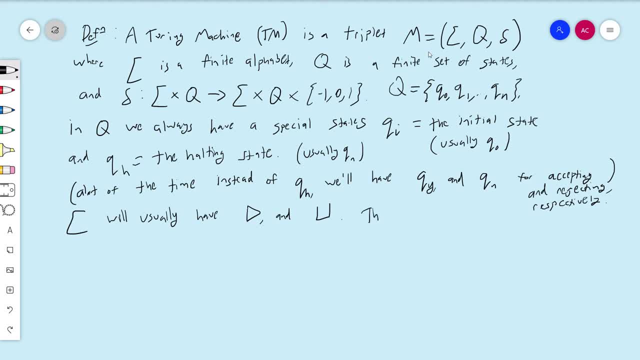 So that's the syntax. So this defines the syntax of a Turing machine. Now we need to define the semantics of a Turing machine. How do I interpret what a Turing machine does? What I really need to do now is I want to define this picture I drew up here. 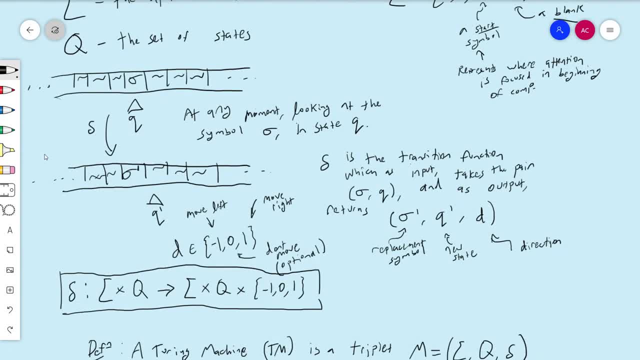 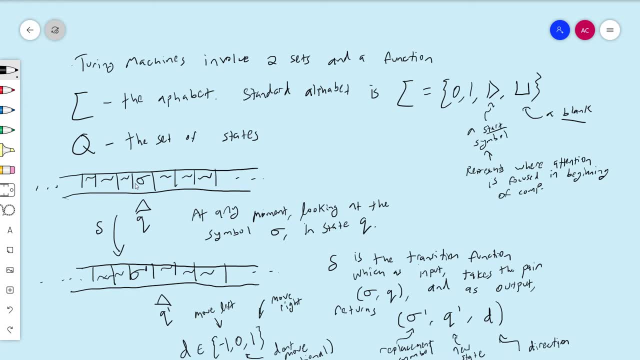 I want to mathematize this picture right here. This is a configuration You can see at any one step. what I'm going to have is I'm going to have a set of tape cells that have some content on them, and then I'm going to be in a state and I'm going to be looking at it. 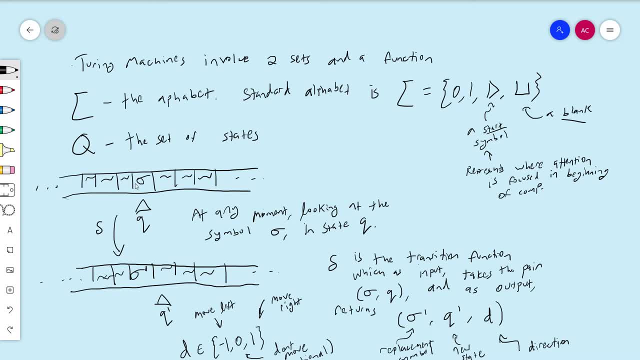 And then I'm going to have a symbol, And so I want basically a mathematical object called a configuration that represents all of this information together at once. So I'm going to define configurations and then I'm going to define what a step means. 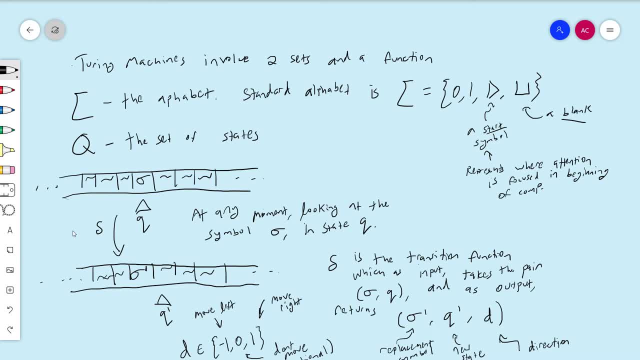 what a step of the Turing machine means out of that configuration. So what does it mean for one configuration, What does it mean for a step to happen is going to be basically to say that this one configuration C yields this new configuration C prime in one step. 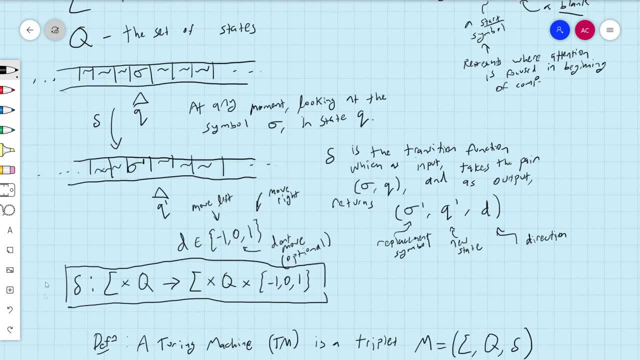 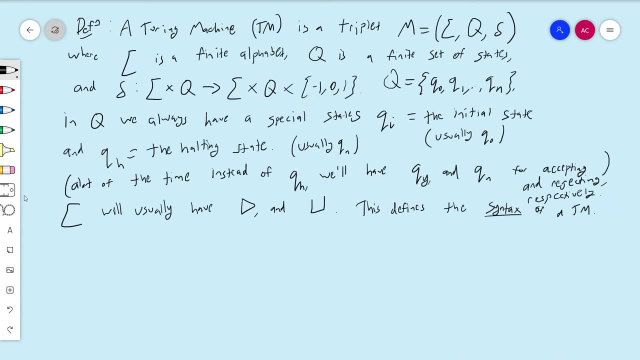 So the configurations are a step, And then I'm going to be looking towards defining what I mean by the word step. So that's the next thing I'm going to define And you kind of just have to see all I mean. the first time you see all this defined, it's kind of overwhelming. 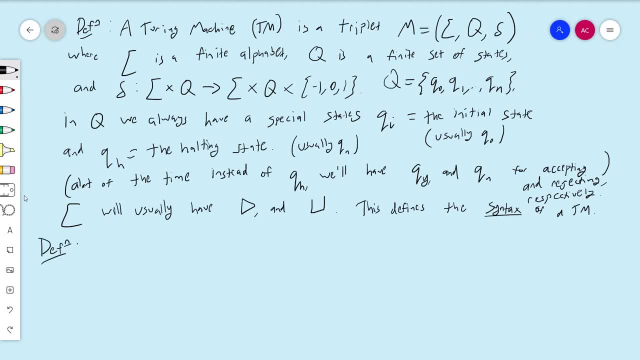 You'll probably have to go through it twice and see some examples with me- And I will do examples for you- to really see how all of this comes together and models the thought process that we had. So a configuration is the next thing we want to do. 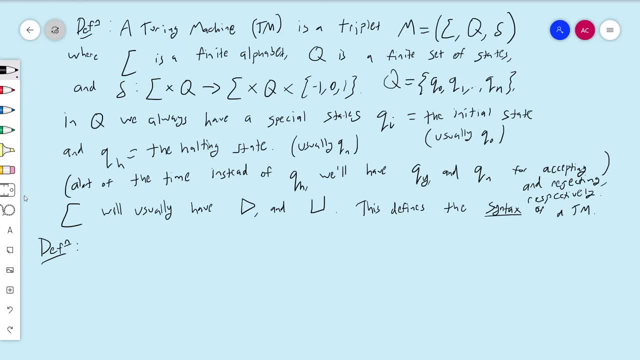 Oh yeah, and I forgot to mention: delta is the transition function, but whatever. So a configuration And a configuration, we're also going to sort of cheat. It's really, really hard to standardize computability theory in like one collection of definitions. 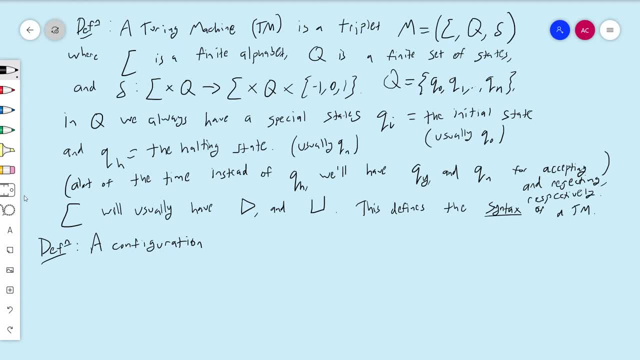 It's sort of no matter what you do, you're always going to encounter one proof where you just sort of wish that you define something a little bit differently, But it doesn't really change much because fundamentally what a configuration is? I should underline my definitions. 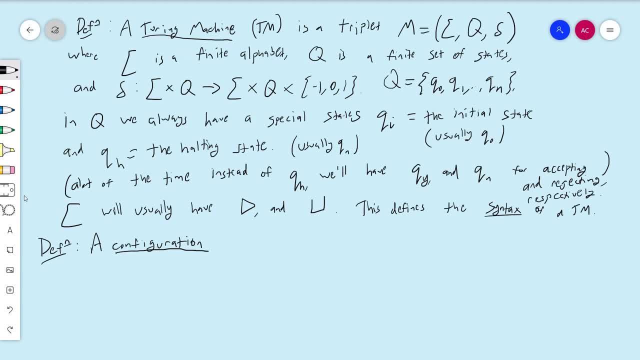 Fundamentally, what a configuration is is just a complete description of the Turing machine at any one step. It's the formalization of that picture I drew with the tape and the stuff. So a configuration is a triplet, Just like the Turing machine. it's a triplet of objects, but they're different objects. 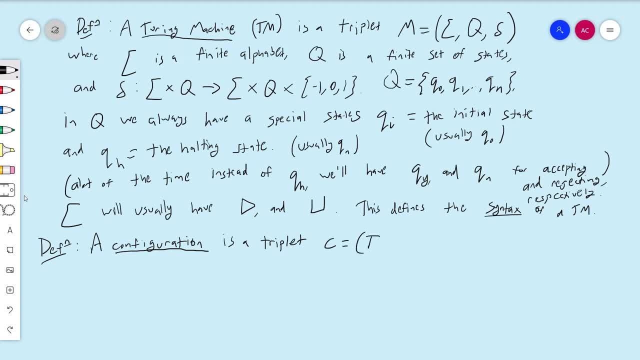 And we use like a lowercase c to do that. We denote it T, Q, Z. So what are these things? T is a finite string. Oh no, I should have probably defined what a string is first. Dang, I'll just say collection of symbols. 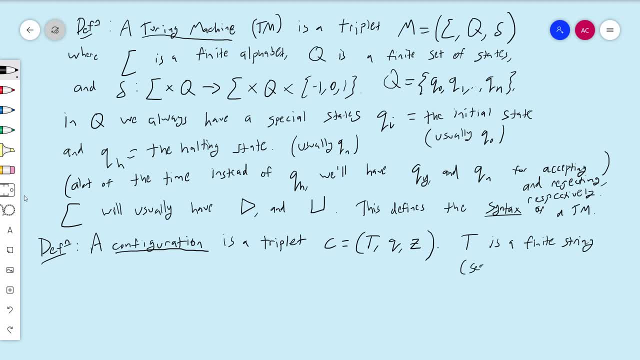 Sequence of characters. Sequence of characters, That's what a string is. So if I have a bunch of characters in my alphabet, you know, if sigma is equal to A, B, C, then you know, then a string in the alphabet sigma would be, you know, A A, A, B, C, E. 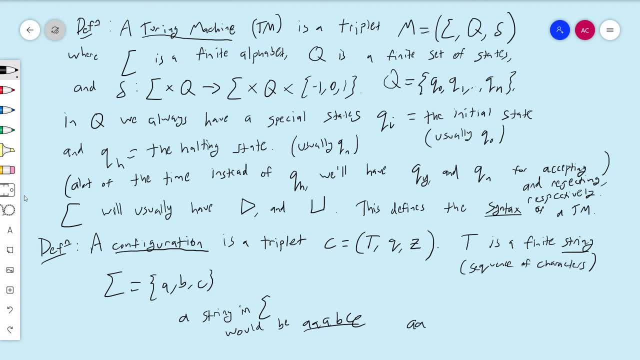 You know, that's, that's a string. You know, A, A, that's another string. B, C, that's a string. That's what I mean by string. Oops, So the string, what T is going to stand for the word? the letter T stands for tape configuration. 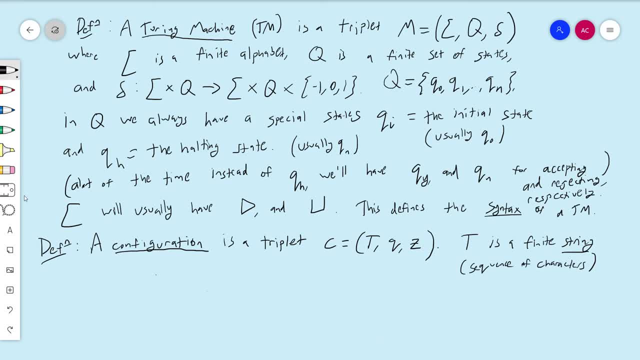 This was kind of laggy. T is a finite string called a tape configuration, Which represents, which represents what's on the tape. So keep in mind, we have a starting step. So at any point in time the Turing machine is on, say step 20,, step 30.. 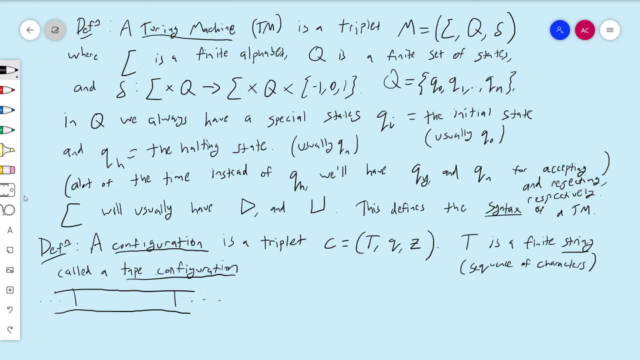 But the number is finite, meaning that the number of non-blank cells on the tape is also finite. So you know, if I have a, if I have a tape that looks like this and everything is blank, everything else, to the left and the right, is blank. 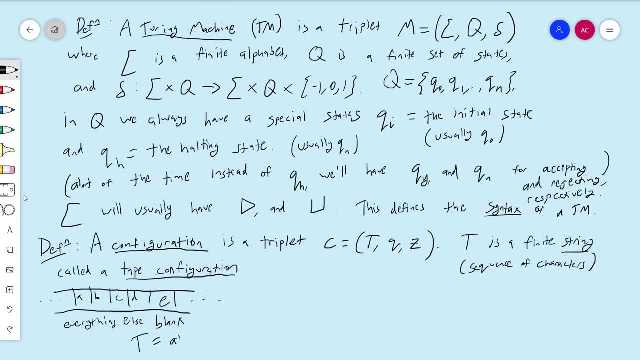 then T, for the tape configuration would look like this It would look it would be this string: A, B, C, D, E. So the tape configuration is a finite string. that basically shows me exactly what the tape looks like. It's a finite string and it can be always assumed to be a finite string. 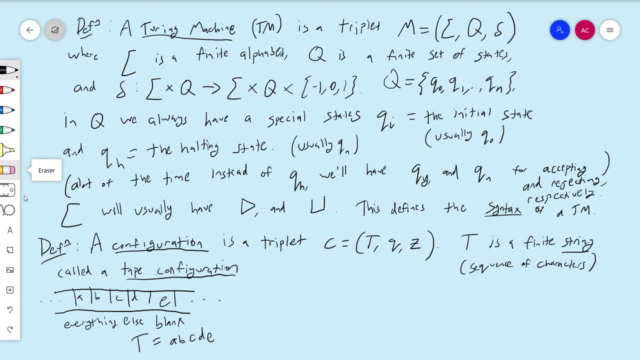 even though the Turing machine is allowed to do infinitely many steps At any one step, it'll be on a finite number of steps. So it's a finite string that encodes everything of value that's worth looking at on the tape. Initially, the tape will be all empty, except for, like your input and that starting symbol. 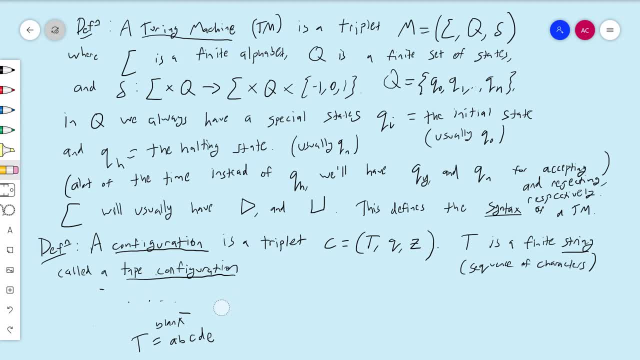 And so we'll talk about that too. But that's what the first thing is. So the T in this configuration C represents the contents of the tape, the contents of the page. what's on the page Q is, of course, the state. 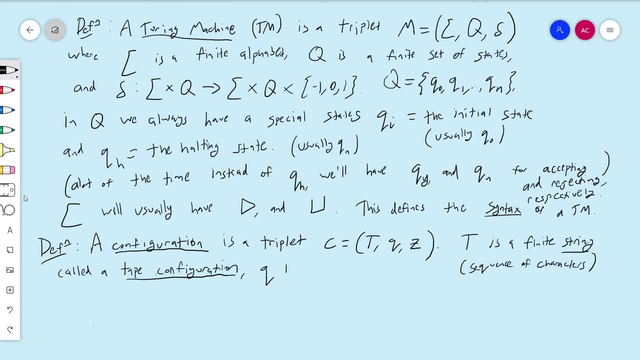 Q is a state. I'll just say Q is in, Q It is a state And Z is an integer. By the way, the integers are, you know, it's all of the numbers: Negative, 3, negative, 2, negative, 1,, 0,, 1,, 2,. dot, dot, dot right. 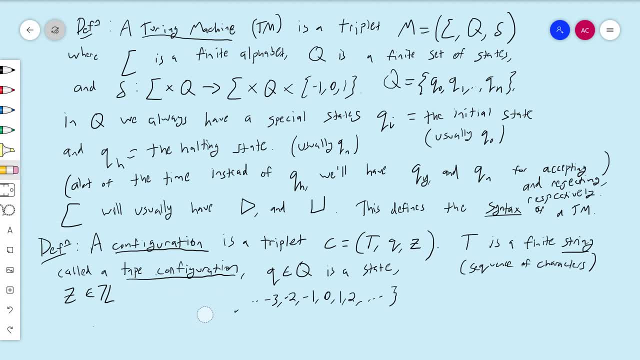 So that's the integers. Again, if you're not familiar with set theory or anything like that, you should check the video description for a PDF that runs you through these basics. There's an integer, And what does this integer represent? Well, I have the tape contents. 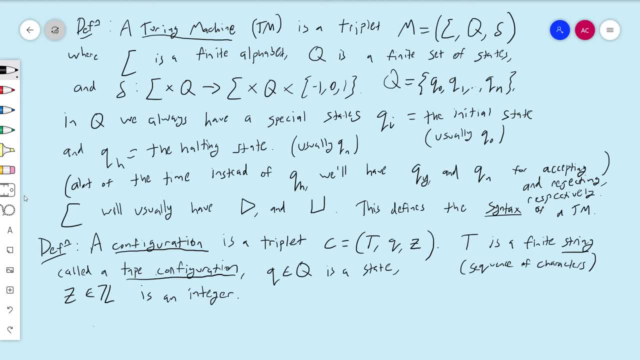 I have the state that I'm in. I also need to know where the cursor is, Where are my visual attention Indicating intuitively represents where attention is And I'm going to start calling that. I'm going to start calling the visual attention area, the visual attention foci, the index. 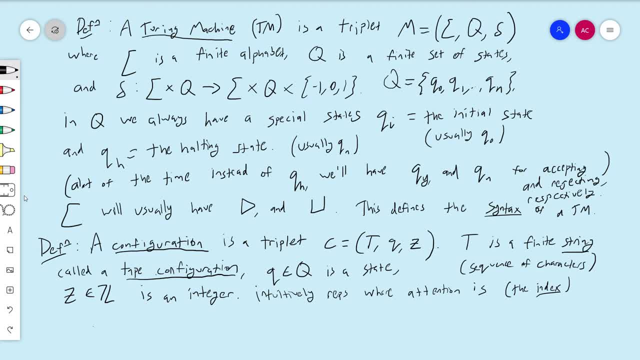 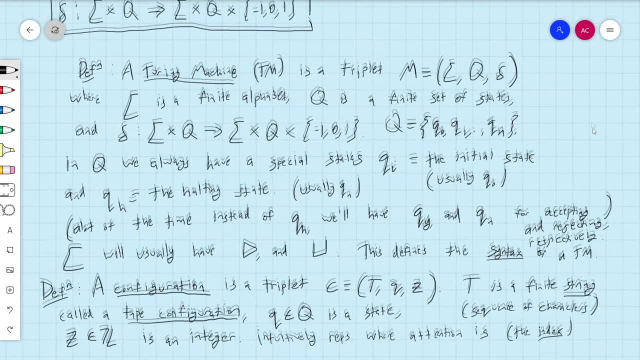 That's sort of a pseudo-vocab word, So intuitively it represents where the attention is. I only I can get away with an integer as an indication of that because, remember, I only have one row of my graph paper And since I'm 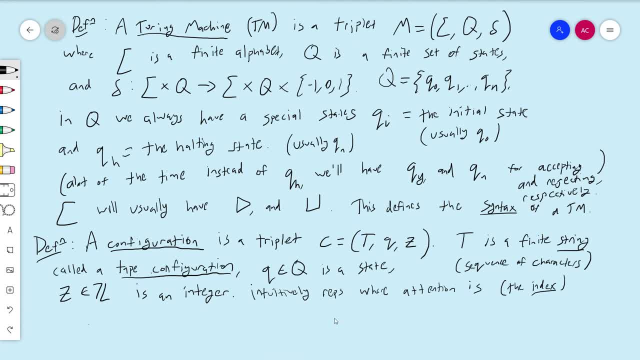 Since the idea is that I'm going to start somewhere. you know I'm going to start somewhere. You know I'm going to start where the play button is. The play button tells me where I'm going to start. I can just declare this to be z equals zero. 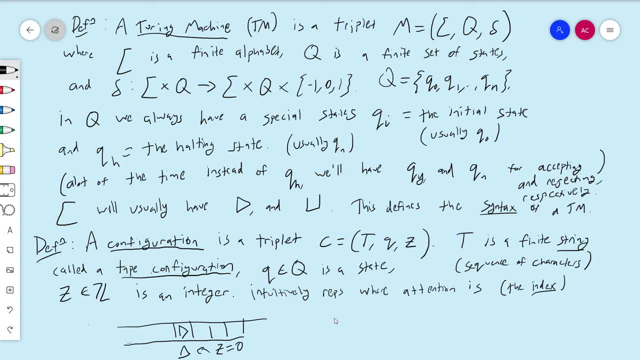 So that the cell- you know three cells over here, this is z equals three, You know. and then I can say: over here, this is z equals negative two, Right, So these three things together: The tape, The tape contents, the tape configuration, the state and the indication of where my focus is, if you think about it. 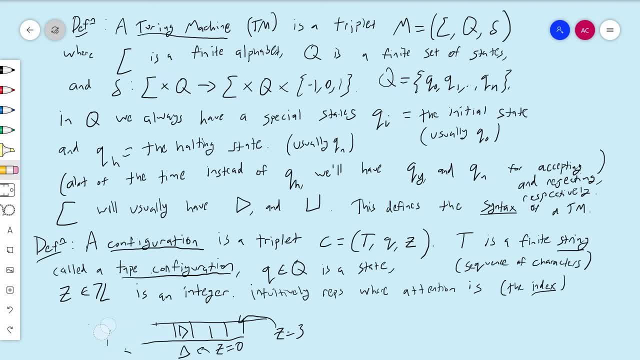 that does represent, That does give you everything that you need to know about what the Turing machine is doing at any one particular moment in time, And I might at some point, for some proof in some future time, I might conveniently pretend that I defined configuration slightly differently. 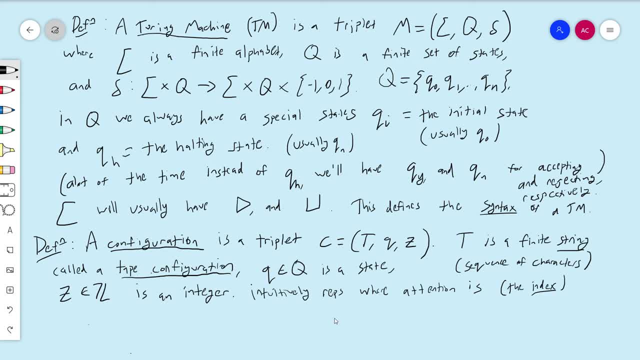 But as long as the configuration does encode these three things, there's a one-to-one correspondence between the definitions and it still kind of works out. All I really need with a configuration is a complete description of the Turing machine which includes what's on the tape, the state I'm in and where my attention is. 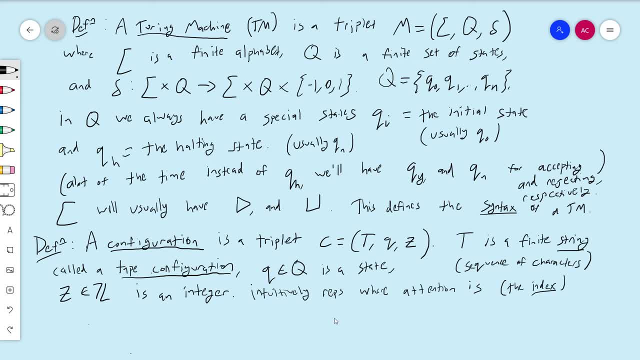 So this is the way I'm going to do it right now is a triplet. By the way, for any z, any z, it doesn't have to be this one. I'm going to say for any like n: Okay. 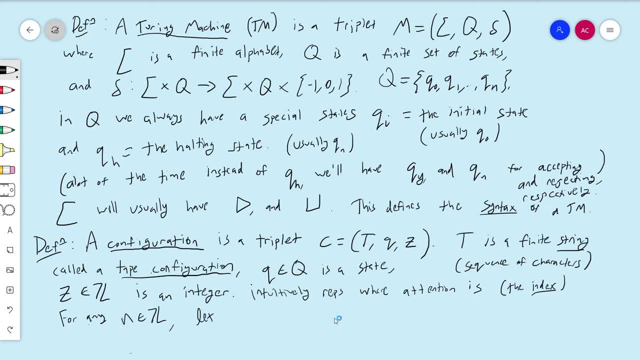 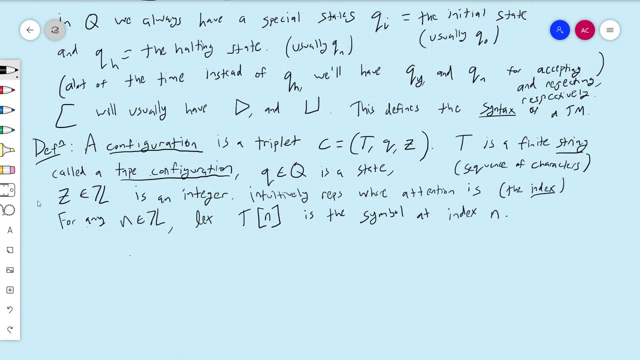 Okay, Let T of z. I'm going to put these brackets. If I write T of n like this, the is the symbol at index n, So you know. so, for example, you know if T is equal to three, a four plus negative. 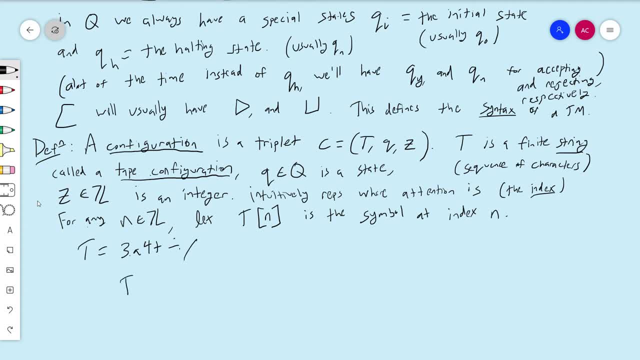 Let me do this. I'm going to divide, sign this, Then t of. I'll call this zero. Actually, I'll call this one, you know. then T of three will equal four, right, The third thing. So this is just going to be my way of indicating, of talking about specific symbols on this tape configuration. 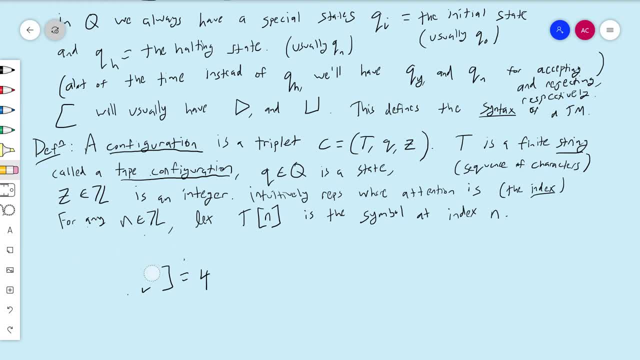 That's the idea, So that's configuration. finally, we're going to define the, the all-important yields relation. So now we're going to talk about how to what a step kind of looks like in the abstract. Okay, so here's kind of a third definition that involves Turing machines. 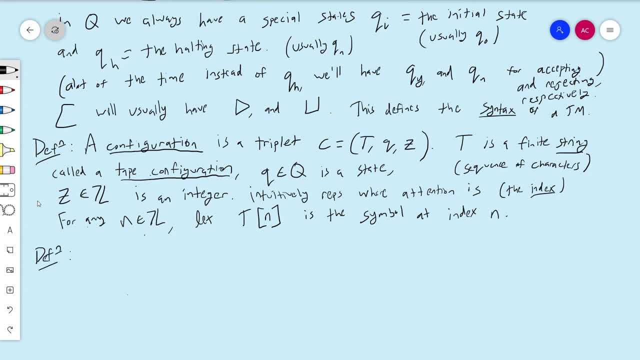 So let m equal sigma q delta be a Turing machine and let and c1 and c2 be configurations of m. So you've got these two arbitrary configurations and we're going to define the all-important yields relation. So here's kind of a third definition that involves Turing machines. 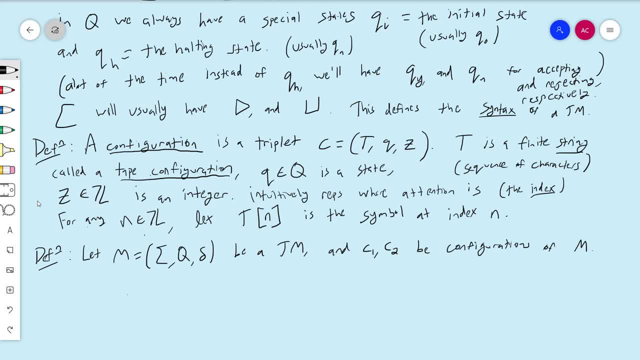 So here's kind of a third definition that involves Turing machines. So here's kind of a third definition that involves Turing machines. What I want to define is what it means for this configuration to yield this configuration in one step. So we say that c1 yields c2 in one step. 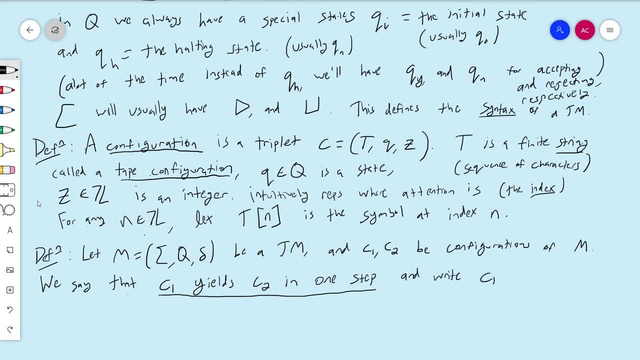 and write c1, c2, and we put an m here. This is the notation, to say c1 yields c2 in one step, If, and you know before I just write down what it what it means, let's figure out what it should mean. 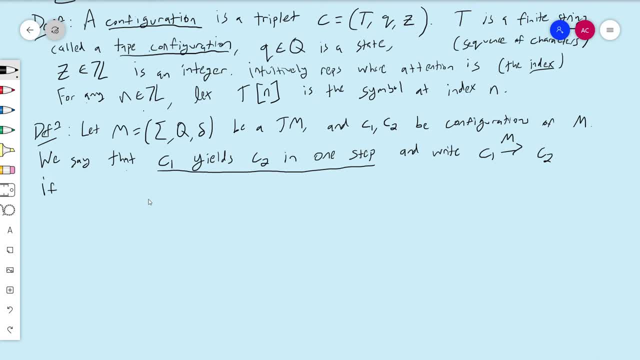 So what should it mean to yield a configuration in one step? Well, here's a configuration. Here's what it represents visually. I should probably actually define crap. Let me do this. I want to give c1 equal. I want to make it equal to something. 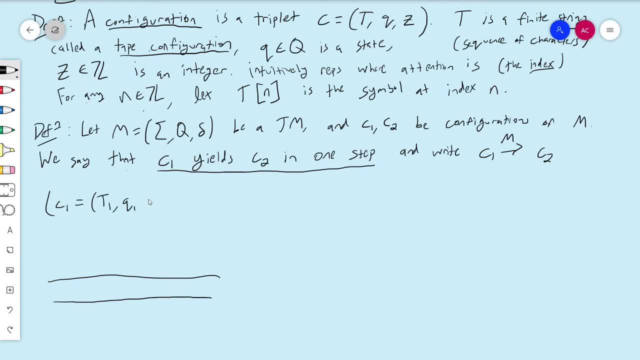 So c1 is going to equal. let's just say t1, q1, z1 and c2 is equal to t2, q2, z2.. So c1 is going to equal. let's just say t1, q1, z1 and c2 is equal to t2, q2, z2.. 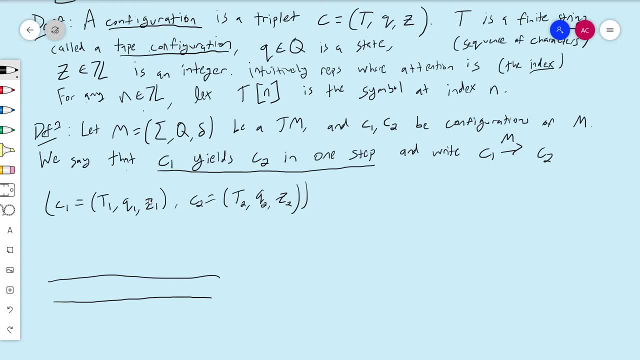 So c1 is going to equal. let's just say, t1, q1, z1 and c2, q2, z2.. There we go. So what does this configuration look like? Oops, no, no, no, no, no. So this configure so t, so c looks like this: 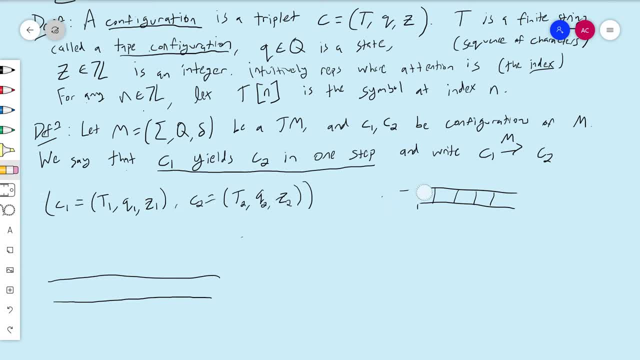 I'm gonna make that bigger, I'll use this. so here's c1 and my cursor, let's say, is right, here, I'm in state q1 and I'm in. what is this here? Well, t, t1 is all of the tape contents. 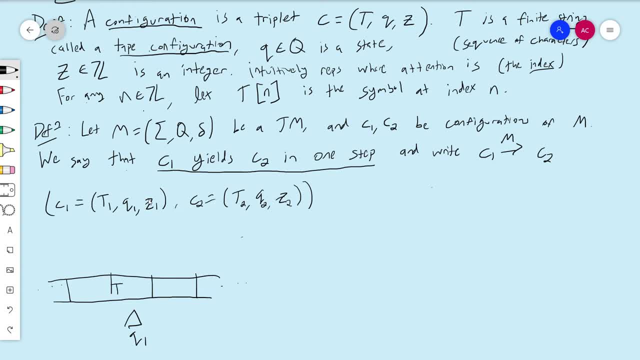 T. so what's in this symbol right here? the symbol in this cell is actually t of z1.. So this is what this is what configuration c1 look. c1 looks like I mean there's. I mean, if you look at the whole thing, you'll see t1,. 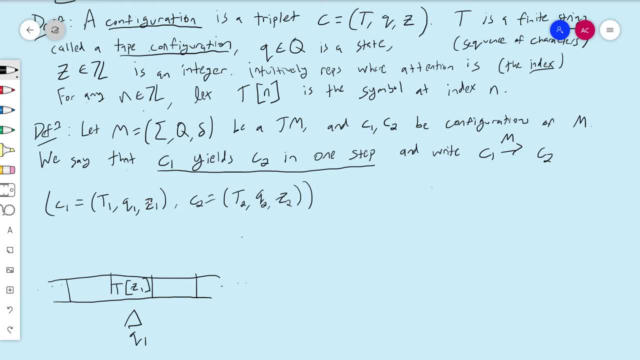 but in one step. this is what I'm looking at, And so what would it mean for this to yield this? Well, it would look like this. So how did I say this? So, first of all, how are these integers related? So this is z1 as an index. 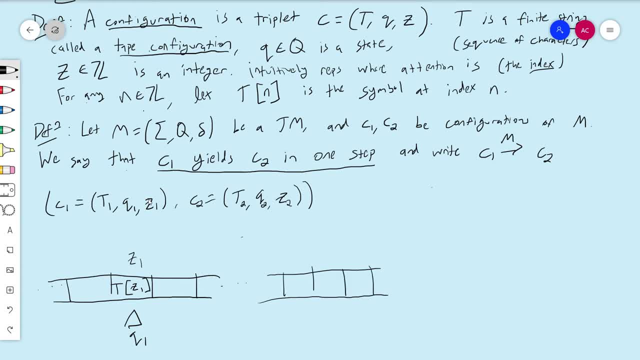 What does z2 have to be? If c1 is to yield c2 in one step, well then z2 would have to either be this or this or this. It can only be one of these three things. And either way, no matter what it is, it's d. 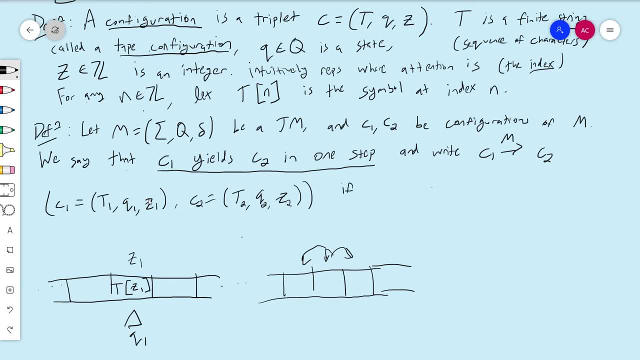 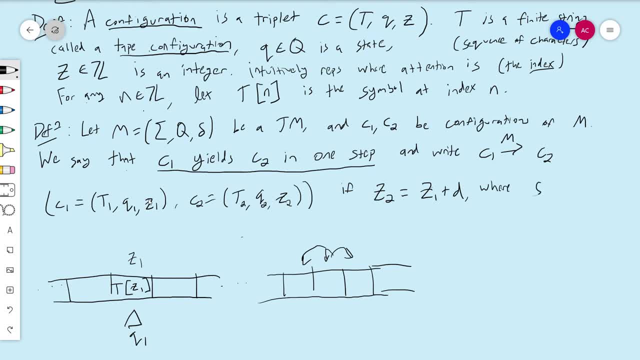 If z2 equals z1 plus d, Where you know delta of t1 of z1 q- ah crap, I'm out of space- Where delta of t1 of z1, so I have you know, obviously. 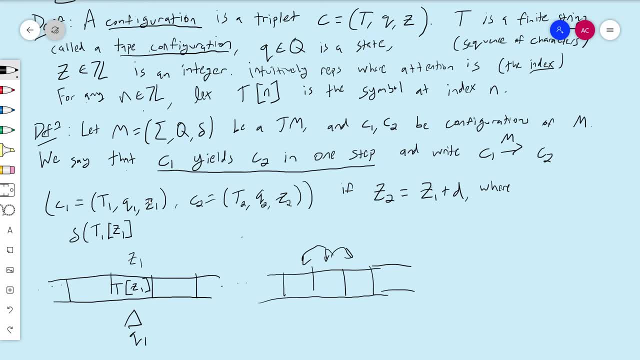 I have this transition function, I have a symbol that I'm looking at and I'm in a state, And so the transition function is going to take the symbol that I'm looking at and the state q1, and spit out three things. 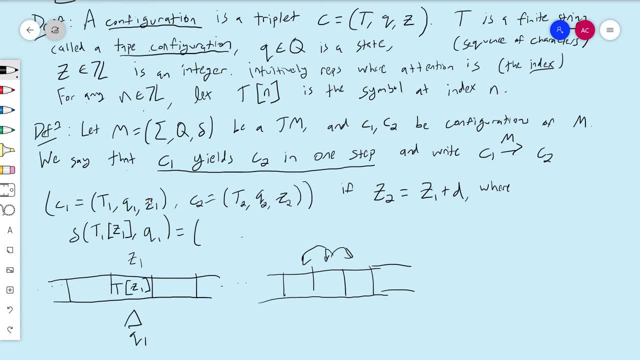 Remember it's going to be. it's going to be a new symbol: sigma2.. Well, I'll leave that empty for now, but it's also going to give me a new thing: q1.. q2, well, okay. 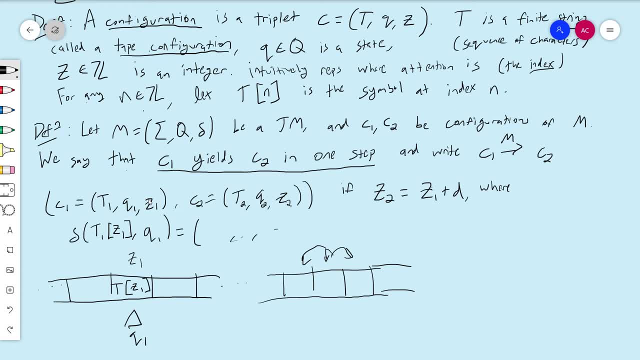 What does delta have to be? Whatever d is here, that's the d that's right here. So it's going to have to be d. So z2 has to be z1 plus d, where d is the thing that spit out by delta. 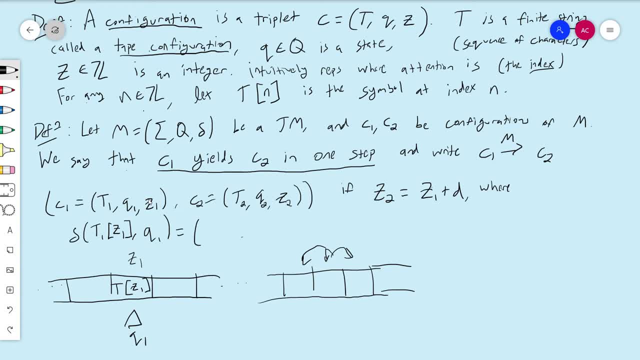 so the third argument given by the delta, And then also this: I'm going to place this boy with an and And: delta of t1.. z1- q1- t1 of z1, comma. q1 has to equal. the next symbol has to be whatever t2 of z1 is. 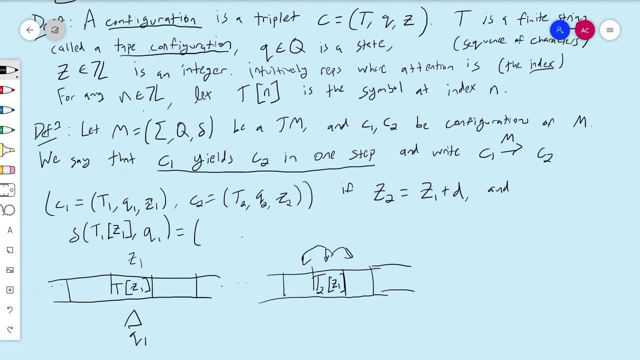 that has to be what's there in the next state. so this has to be t2 of z1, and then q2 has to be the state that it outputs, and then d is the direction where z2 equals z1 plus t. i probably should have said this first and then this second, but these are the two conditions: z2 equals z1 plus. 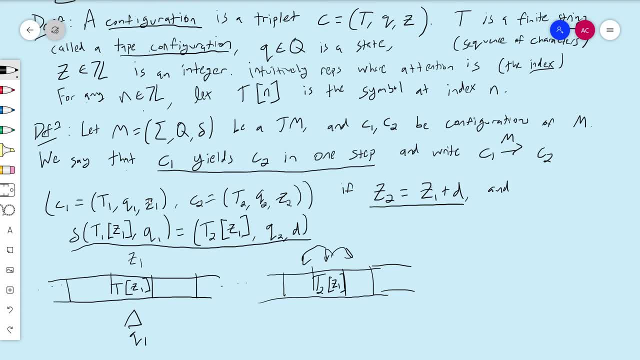 d and then this is the relation that has to be true. so this is what it means for c2 to c1 to yield c2 in one step. it's just a formalization of of the of the transitions between configurations that we're kind of envisioning. it's very formal and we might not use the formality. 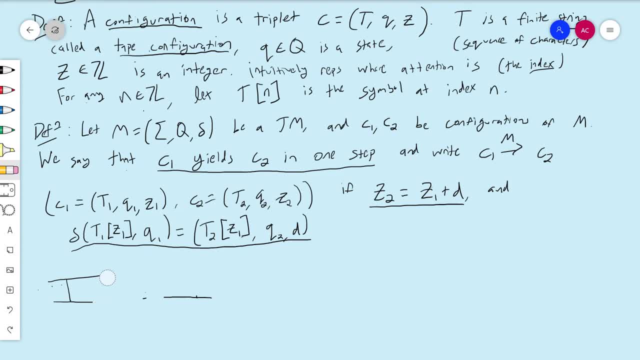 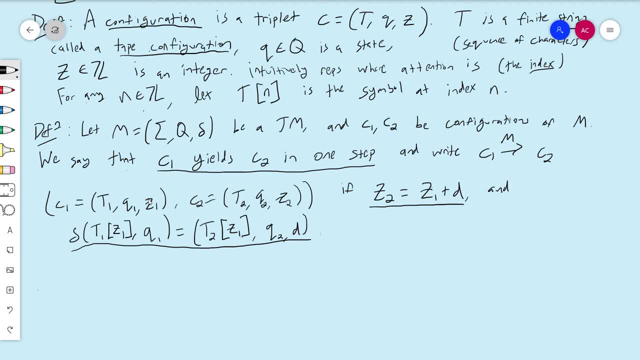 this, but it's important to go through the process of formalizing it just once. so that's what it means for c1 to yield c2 in one step, and then, inductively, we can extend this definition to what it means for c1. we can now. 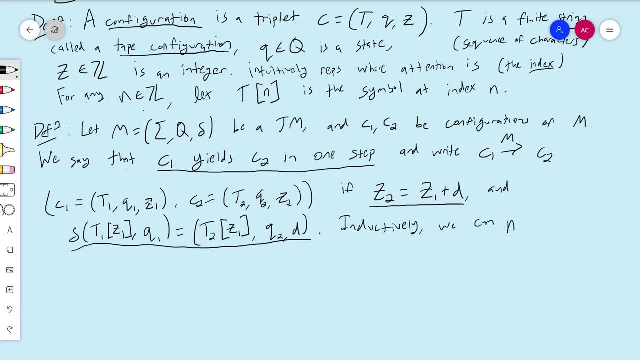 define what it means for it to be yielded in many steps. we can define c1 yielding c2 in k steps or some k in the obvious way. so I'm not going to go through all of that, but basically now for this: if c1 yields c2, 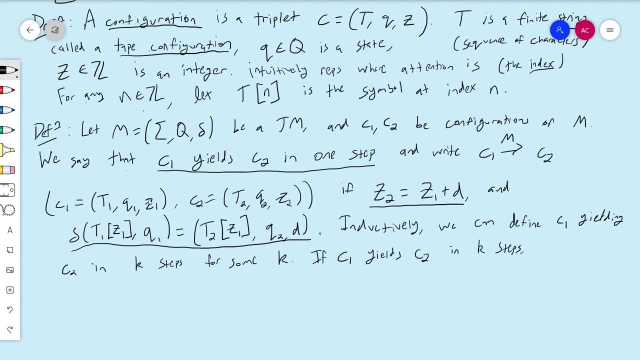 and k steps. for some k, we're gonna write c1, arrow c2, and we'll put an m here, but then we'll put a k as like the power to imply, kind of that. the machine is like that as like random power shift, so we get that. w here, and then we'll put an m here, but then we'll put a k as like the power, to imply kind of that the machine is going to yield c2, we're going to be able to e4- it's going to be almost equal. but then we'll put a k as like the power. 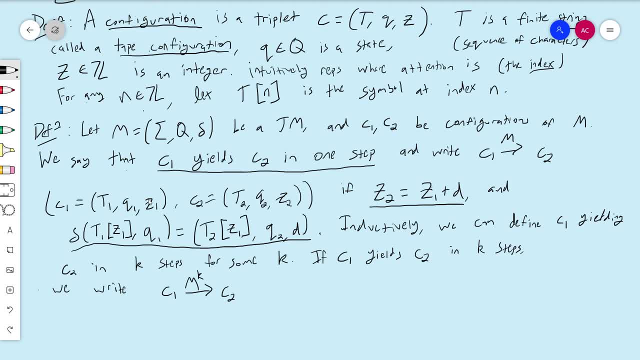 simply Hmf and we're just going to put a n if we work, just run and say that, because that's what this is, machine. the yields relation is just kind of being used, you know it's. we're kind of just doing k steps, we're doing the m? m is happening, k times is essentially what the notation is. 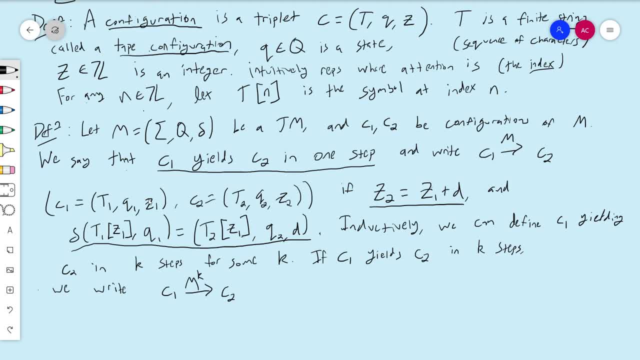 there for. So that's the yields relation. So I mean you can see how we're kind of defining semantics now. We define the Turing machine in terms of like just a collection of three things: two sets and a transition function. but also, you know, we've also got this yields relation. 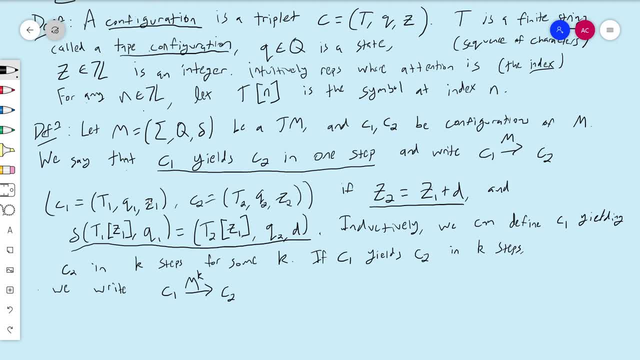 Now we're sort of talking about what a step formally means and what a configuration formally means and stuff. So this is what I mean by semantics. Now we need to define starting and stopping and halting and stuff like that and how to interpret that stuff. 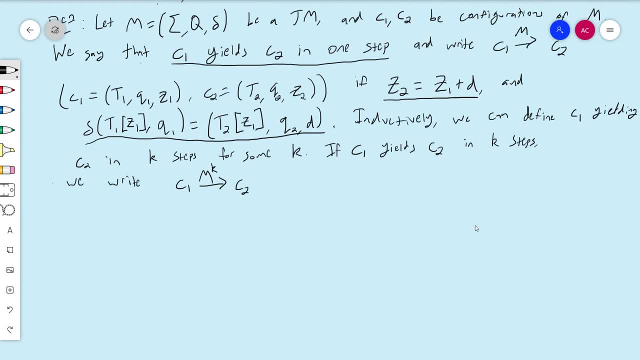 So first off, we want to talk about inputs. So I mentioned that sigma always has a blank symbol. We're going to require that inputs don't involve any blanks, except when there's- except when we're modeling functions that take more than one input. In that case, 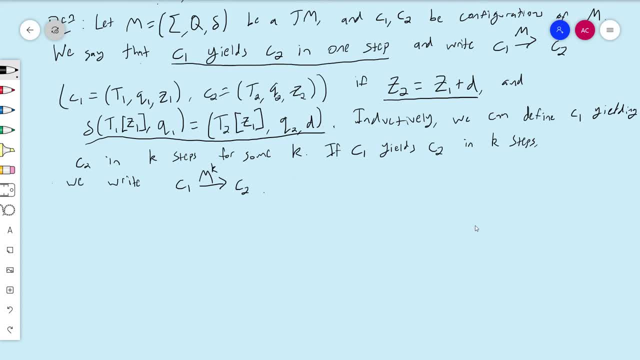 we'll split up the inputs by blanks. So we call so. for strings, you know, x which don't have a blank symbol. we don't have blanks, We'll call these inputs. We'll call them inputs, And then for any x. 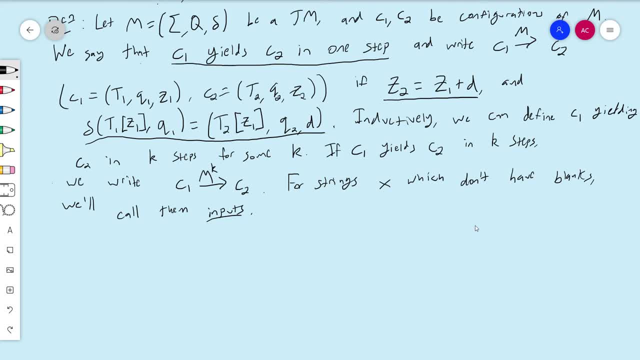 we want to define an initial need, an initial configuration for x. So that's what we're going to define next, And so that'll just be kind of what we need it to be. So T of x is how I'm going to denote that, And that'll be defined to equal. this is what 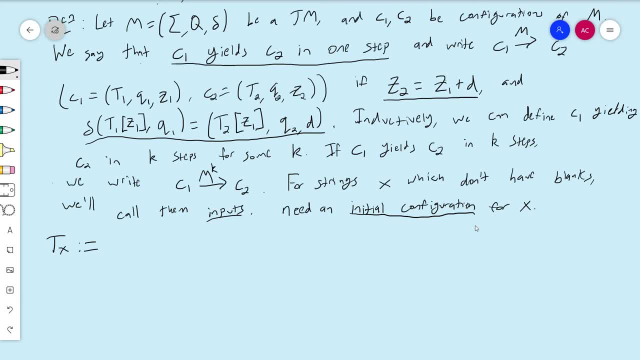 the colon equals is a definition. It means I'm defining T of x for any input, x to be what, But it's going to be- wait, I'm sorry, getting ahead of myself- cx. that's what's going to denote the initial configuration and that's going to consist of t sub x- and I'll define what that is in a minute- q sub i- whatever the initial state is, that's guaranteed to be there- and also 0, where z is 0.. 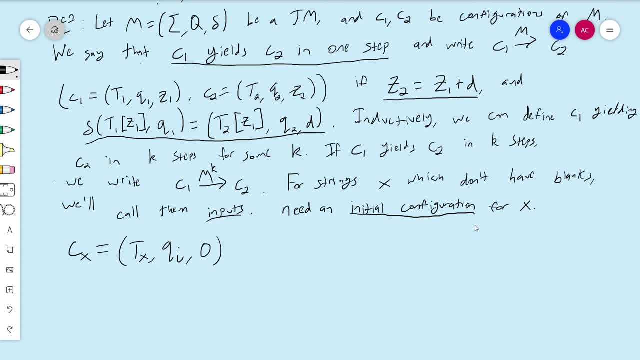 Remember, a configuration consists of a string that represents the tape contents, a state, which I want to be the initial state, obviously, and also 0, and to indicate that the location that I'm starting at is the 0 location, and then everything else is relative to there, where t sub x is equal to, effectively, just the play symbol followed by x. 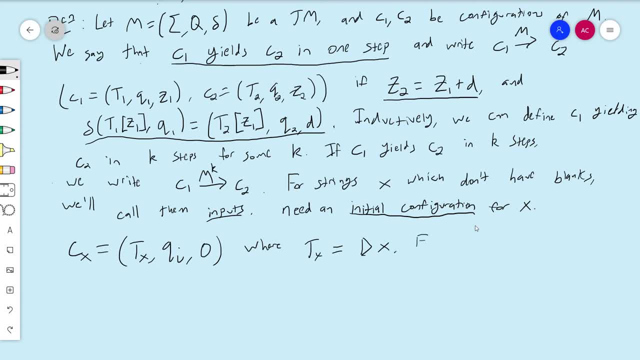 So they're kind of different. I'm going to be more formal. t of 1, I'm not going to be more formal than that. You get what I mean right? The initial configuration represents this. I'll be more formal. 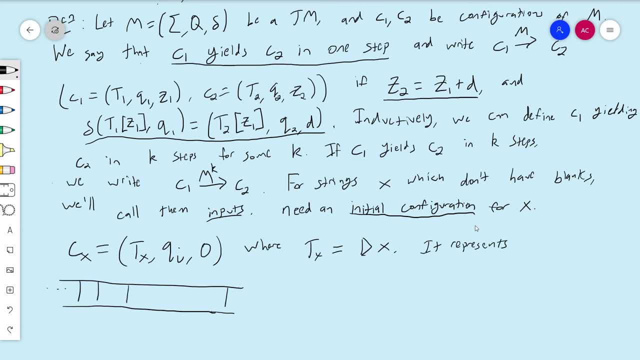 I'll be more formal with strings and stuff in a little bit, but I think hopefully people get the idea. Actually I don't want all those. So initially we have a situation like this where we have the play symbol, where we're pointed at the play symbol, we're at index 0, or we're just going to declare that starting point, index 0, and then x is just kind of as much as it needs to be. 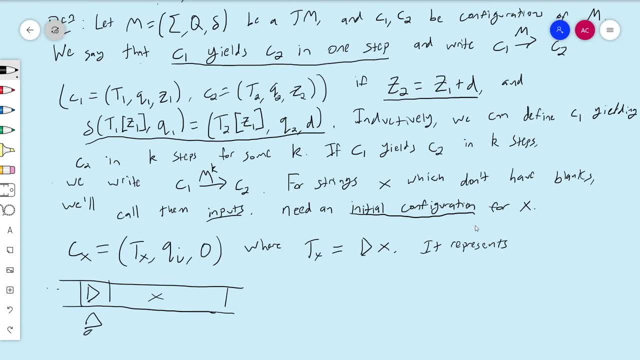 And we're in state qi. So when the turning machine starts up, this is how it's going to look: We're in the initial state, We're pointed at the play symbol. x is going to follow the play symbol, It's some finite string and then everything is blanks following that. 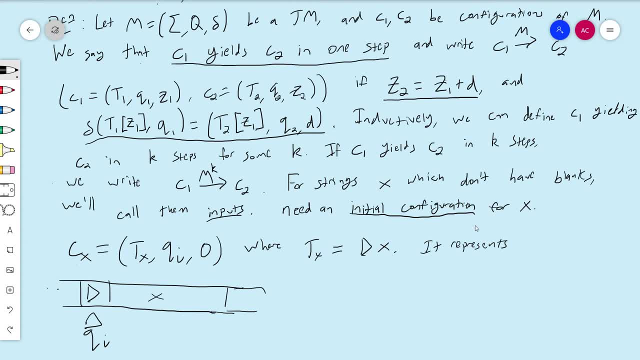 And so this, you know, c sub x represents this. This is our initial configuration. So now that we have an initial configuration, we also have defined. now, kind of, we can start to think about the turning machine doing things, because we take the initial configuration for an input and then we just use the yields relation repeatedly on it and then we get results. 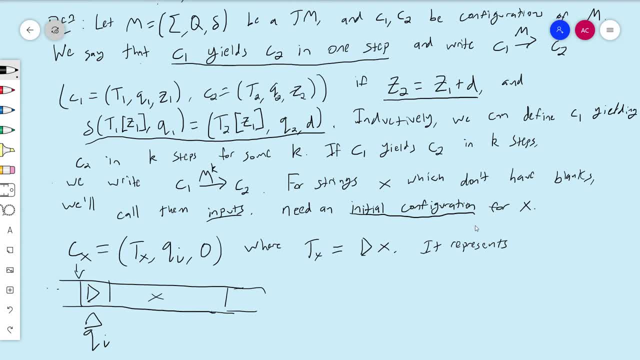 And now we've sort of semantically modeled: Yeah, Yeah, The steps, Okay. So now we need to define what it means for a turning machine to halt. So we say that m halts on input x in k steps. if I'm going to, 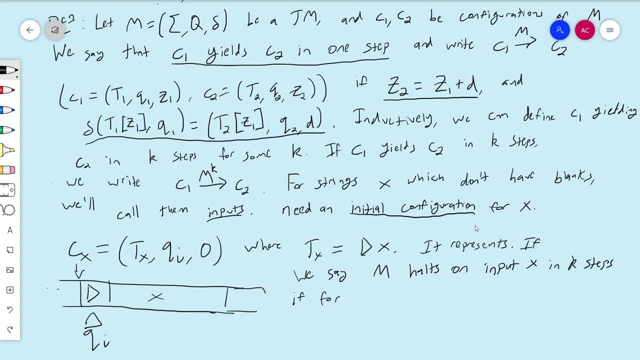 I'm going to define state. So if k is some, For some k if Oh, okay, We say m halts on input x in k steps. if this is true, If c x yields, I cannot draw my arrows without going up. 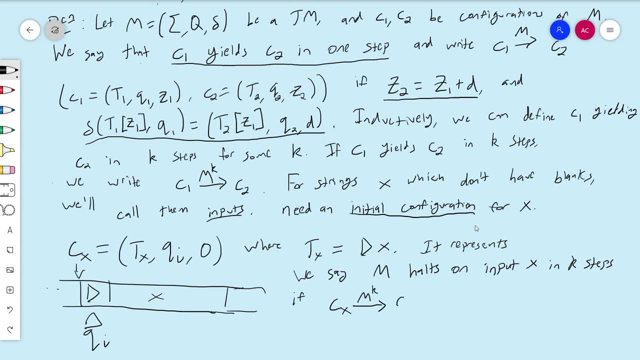 There we go In k steps c sub x yields some new configuration c, I'll call it ch. where ch equals this, It equals t, For some t we don't really care about. but more importantly, q has to be the halting state for some t and z. 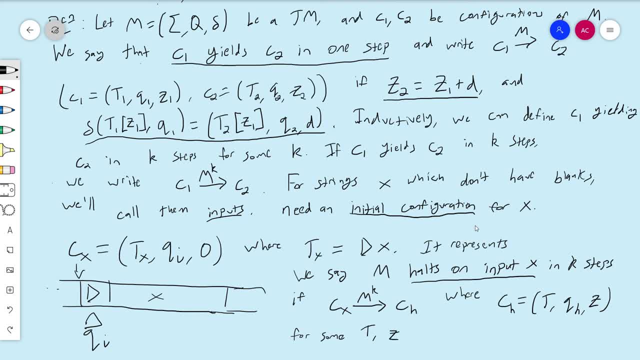 We don't care what t is, We don't care what z is, We don't care what t and z are. What we care is that at some point, for some number of steps, eventually the initial configuration yields a halting configuration in the sense that at some point, the state here will be the final state to indicate that my mental state has detected. I am at the end and I'm finished. 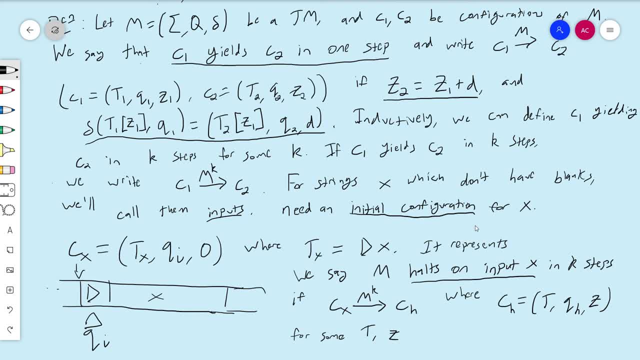 So to be a halting, To halt on an input is to say that eventually, for some number of steps, we get to a halting state. And the interpretation of getting to a halting state is that the turning machine stops computing. There's no more computing to happen. 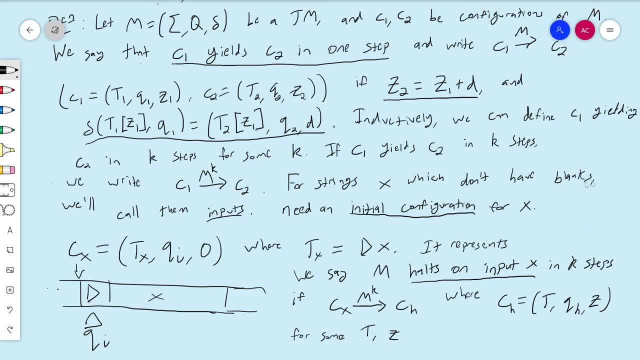 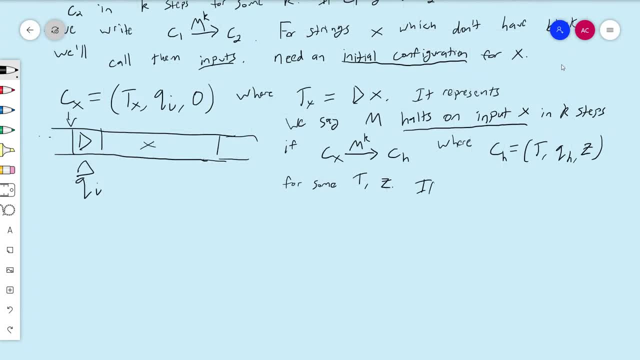 You know, if we're talking about accepting and rejecting, if we have q y and q n instead, then we say m accepts The input x If ch equals t, q, y, z And m rejects the input x. 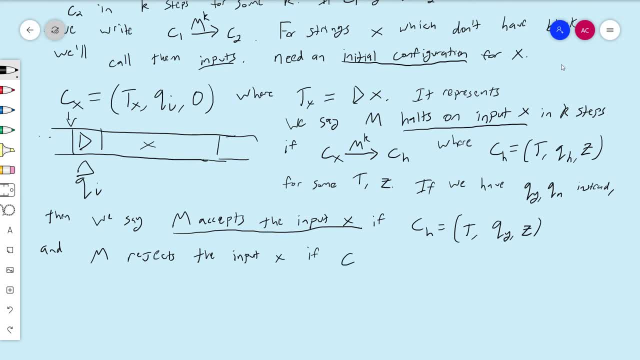 If ch equals t, q, y, z. So sometimes we're concerned with accepting and rejecting, And again, this is just there for convenience. We could easily, instead of doing accepting and rejecting, we could just erase everything. We could use just one halting state by saying: okay, you know you've halted. 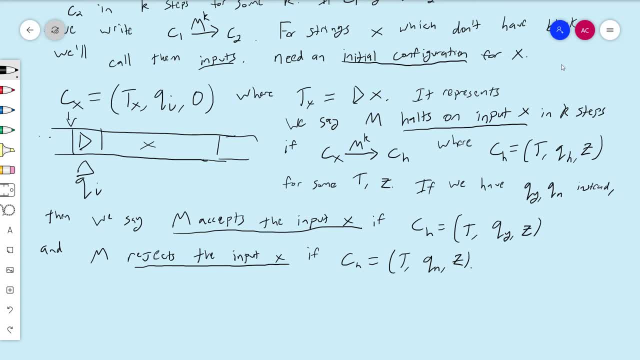 You have an answer supposedly: Just erase everything, Print a one and then stop. But then that leaves one last thing to define, which is the output. Okay, Also define also if m halts in k steps, in some number of steps in configuration. you know t, q, h, z. 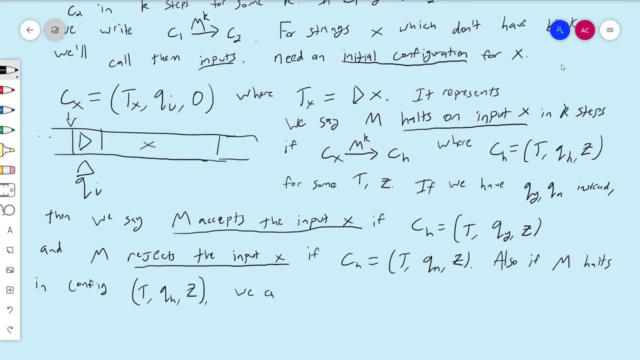 We call the string t the output of the machine. So the string that we're left at when we halt, If we halt, is the output of m on input x, which we denote m of x. So that's the output. So sometimes we're concerned with accepting or rejecting, in which case we don't really care what t is. 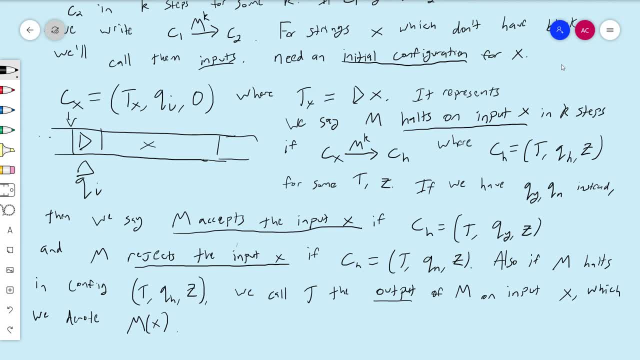 We just care if we get into a halting state, that's yes or no, And then this is just the scratch work we use to get there. Okay, We're concerned with the output. Sometimes we want to think about m as like computing, a number for us, in which case the output will supposedly be that number. 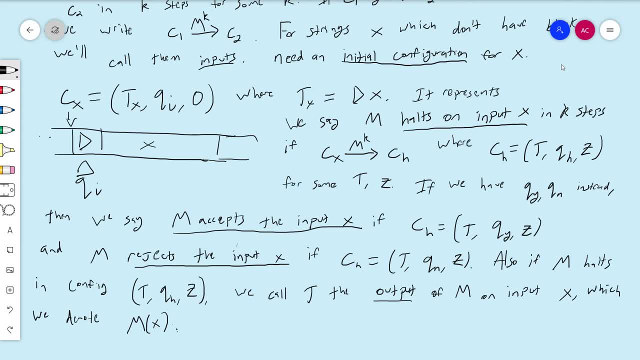 And we're going to denote m of x Also. however, the machine might never halt. If the machine does not halt for any k, then we're going to write this For the output Instead of: I still want to say that m of x equals something. 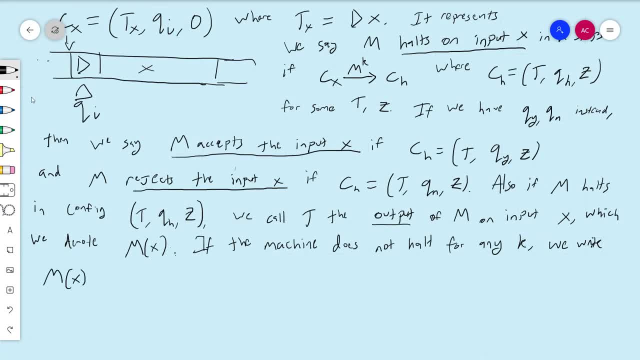 Instead I'm going to write: m of x equals diagonal arrow. So the machine output will always- I can always- say: m of x equals something. If it halts, then it's going to equal, whatever the tape configuration was at the time that it halted. 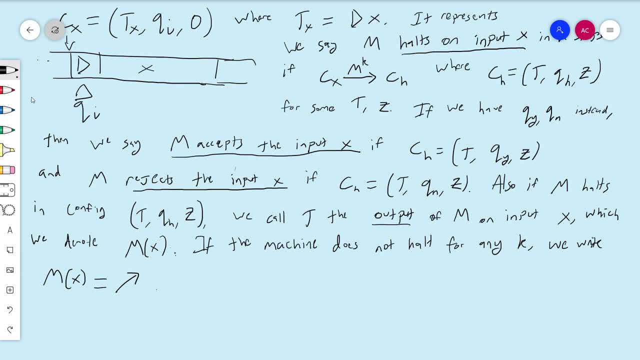 And if it doesn't halt, it equals this arrow to indicate that it does not halt. It's just notation for me. So you can sort of think of the Turing machine as a function that takes inputs and spits out outputs In this way. 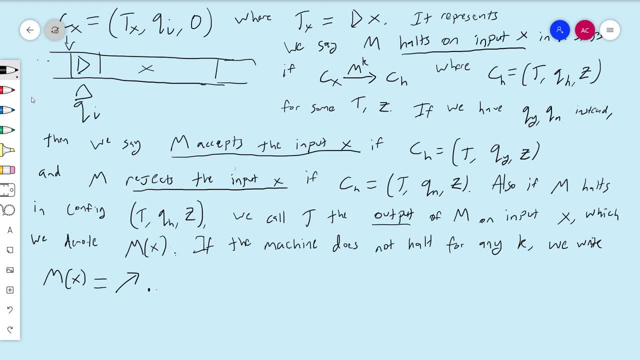 It sort of double functions as a function. It models a function, right. It only really models a real function if it always returns an output, In other words, m of x. the Turing machine only really represents a function if this never happens. 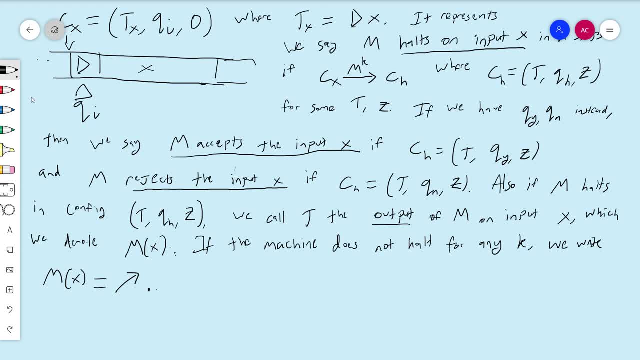 So that's that. So that's a Turing machine. That's the whole definition of a Turing machine. I know it's extremely. that's probably the most complicated math definition that most people have seen before. Let's zoom out and see how much we just did. 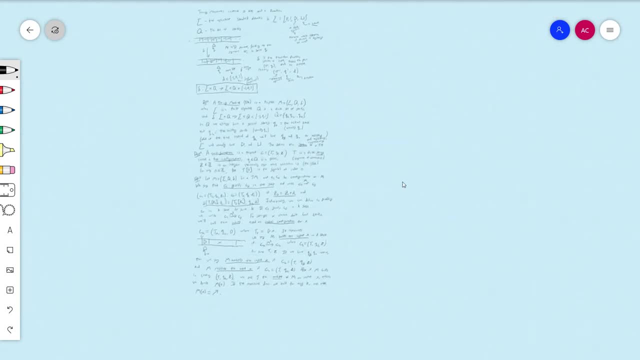 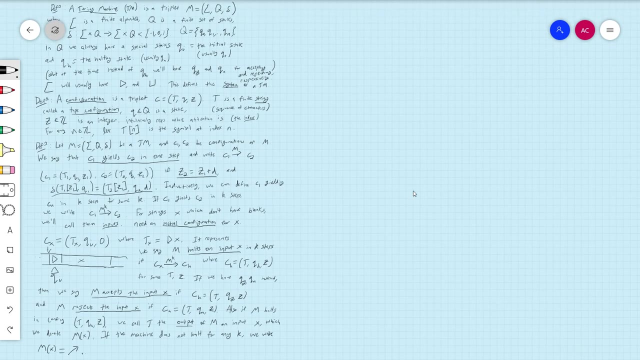 Whoops, Yeah, all of this, All of this is one definition. really Starting, I guess, starting here, This is all one definition And we're sort of not done yet, Because what I want to do now is I want to define what a problem is. 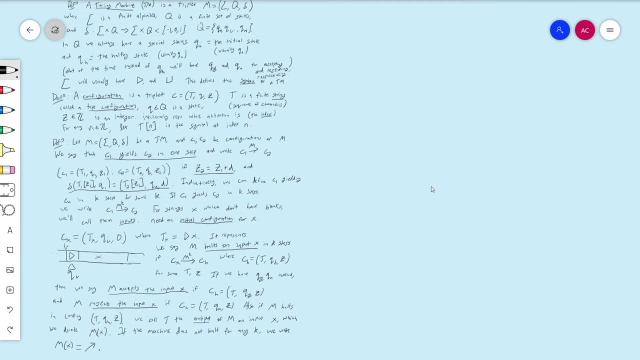 And I want to define what it means to solve for a Turing machine. to decide a problem, To solve a full-on problem. I have what it means to accept and reject inputs, But now I want to talk about problems themselves being computable. So let's do that next. 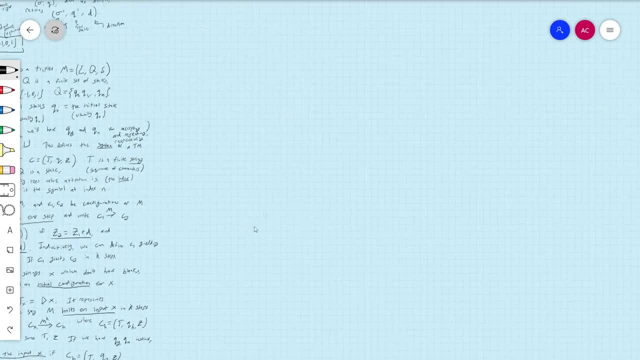 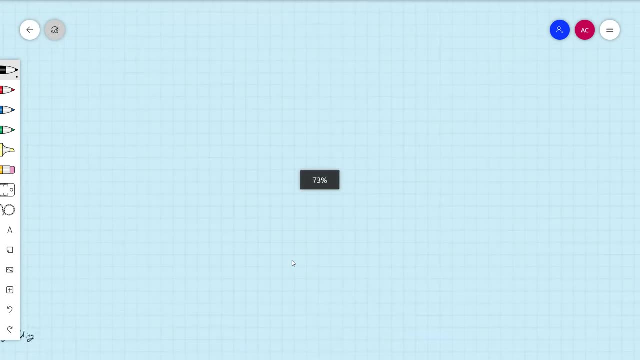 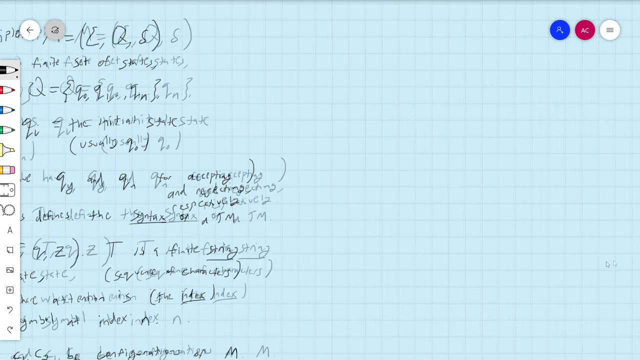 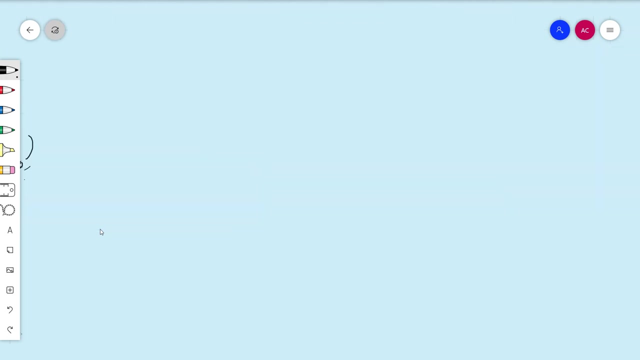 I'll do that on the side here. So next we want to formalize decision problems And say what we mean By a Turing machine, solving it Or deciding it. Okay, So let's formalize what we mean by decision problem. 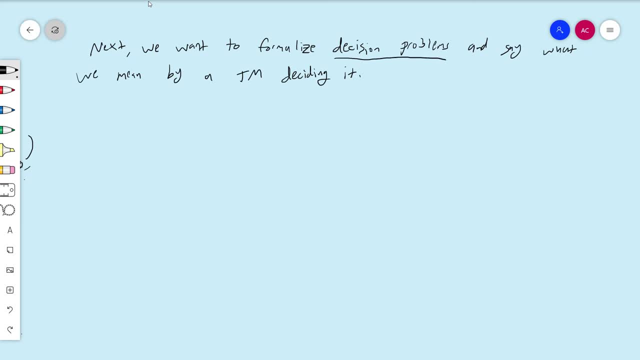 Well, a decision problem- recall from the last video- is a problem that it's a problem where the answer is yes or no. So an example of a decision problem would be, you know, factoring. The factoring problem, that's going to be an important one, right? 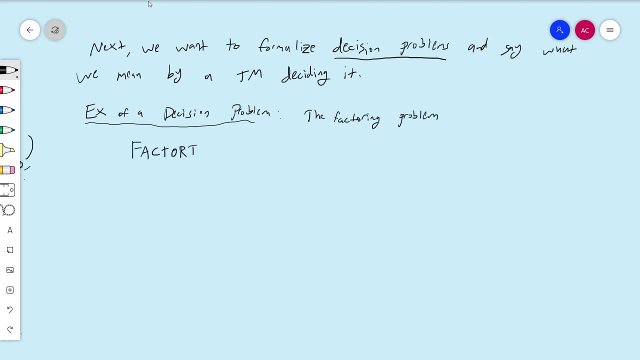 So factoring, you know, is the problem. So, given an integer z, does it have a fact, does it have a non-trivial factor? That's the question. So you know if I gave you a 4, the answer is yes, it has 2.. 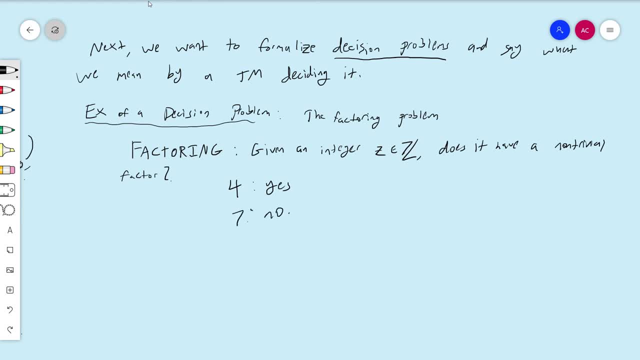 You know if I gave you a 7, the answer is no. That's the factoring problem. It's a decision problem. Does the number have a non-trivial factor, Yes or no? That's informally what the factoring problem is. 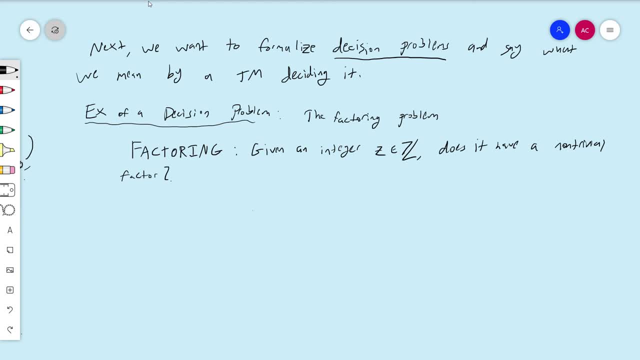 So that's another example of a problem About add. This is a stupid problem. It's sort of the addition problem. It's sort of the decision problem. version of addition. Given three integers, You know a, b, c. 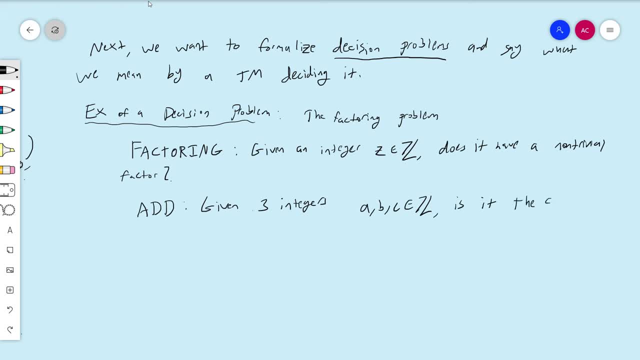 Is it the case that a plus b equals c? Right? So that's sort of the yes or no problem version of addition, You know. so these are decision problems. I'm stating them informally and what we want to do is kind of view them as objects. 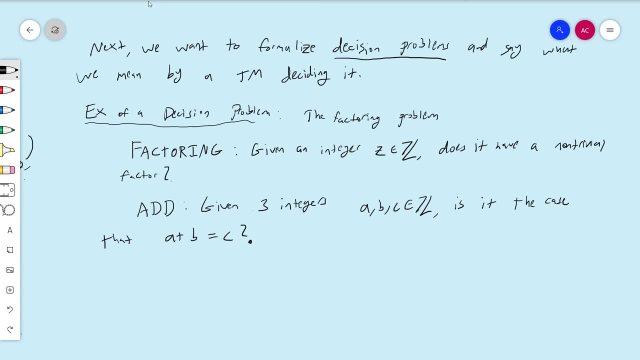 But how do I do that? How do I view them as objects? So this is the informal Kind of thinking, Thinking about a decision problem, And we can formalize this By Looking at a decision problem As a collection. 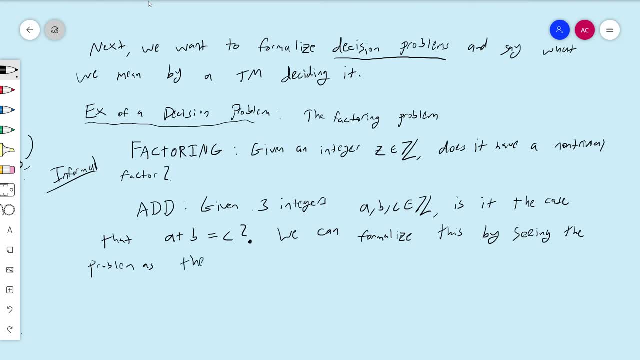 As the collection, As the set Of all yeses And all of the yes answers. That's how we view it. So, in other words, it's a set of strings. A decision problem is a set of strings, Where the interpretation of the decision problem is that you're. 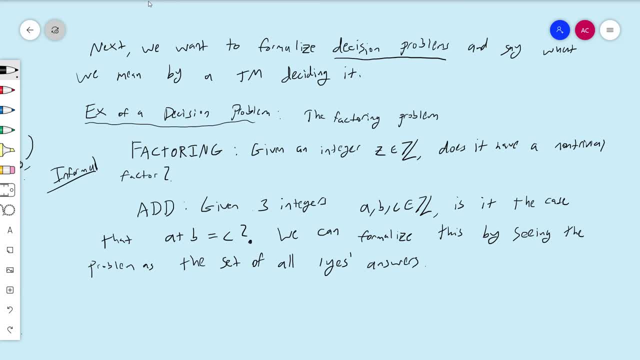 That the answer is yes if you're in the set And the answer is no if you're not in the set. So, formally, Formally, The factoring problem, The factoring problem is the set of all of the yes answers. 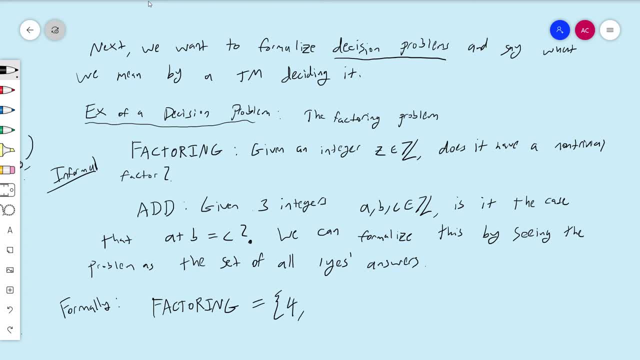 So the first one would be four. One and two and three are not a prime. Yeah, one is prime, I guess: Six, seven, eight, nine, ten, twelve, fourteen, fifteen, sixteen, eighteen and so forth. 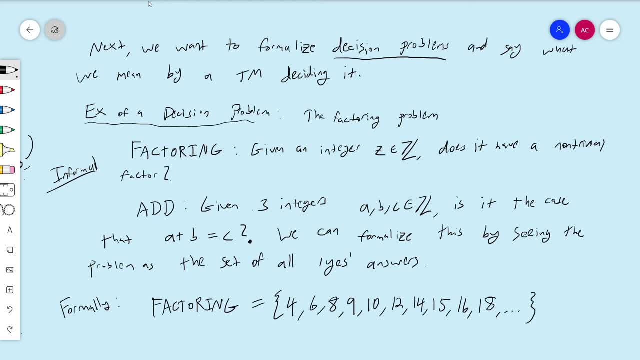 So this is the factoring problem As a set. So it's a set. Now it's a set of numbers. But remember, when I was talking about Turing machines, I was talking about strings. So this is the formal way to define the factoring problem. 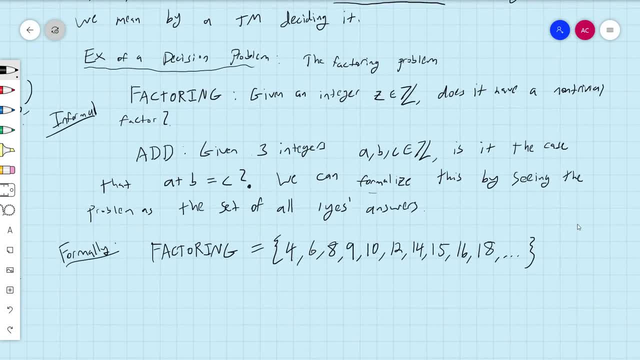 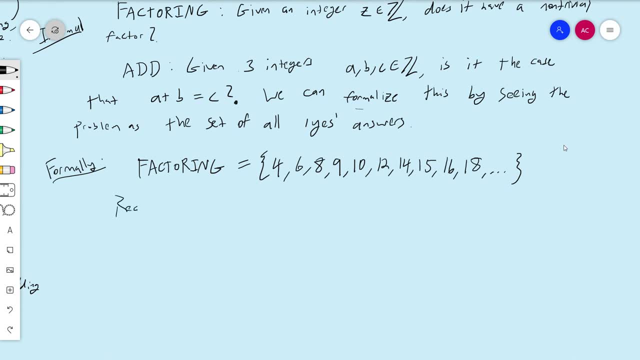 But let's talk about kind of more generally, formally defining a decision problem in general. What kinds of objects are decision problems? So again, recall, Recall: we have a finite alphabet sigma. Doesn't matter really what it is In the case of, and so you know, what I'm going to define here is: define sigma star to be the collection of all finite stars. 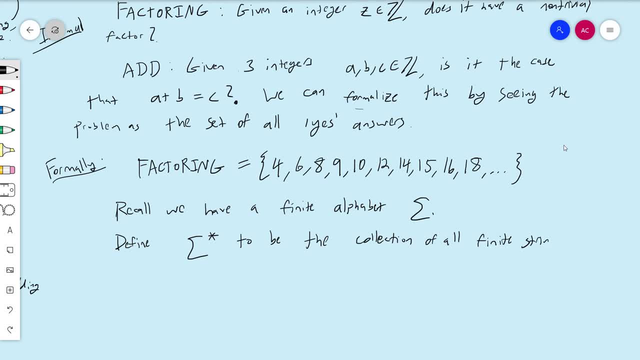 And what I'm going to do is define some strings of characters from sigma, This star. this is an operation that you can do to an alphabet. So I take an alphabet which is a finite set of characters and I can kind of apply the star operator to it. 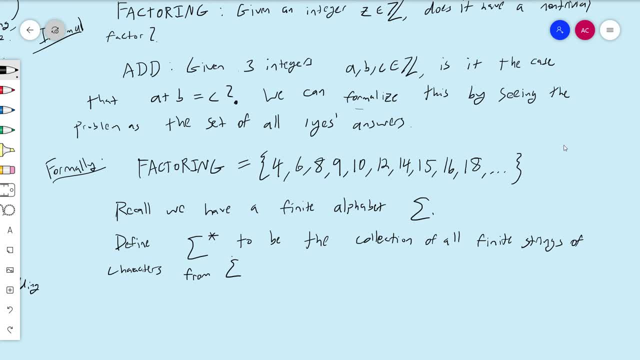 And what I get is this infinite set. It's infinite regardless of how many things are in the alphabet. It's the set of characters. It's the set of characters of all finite strings. Sometimes the star is called the Kleene star operator. 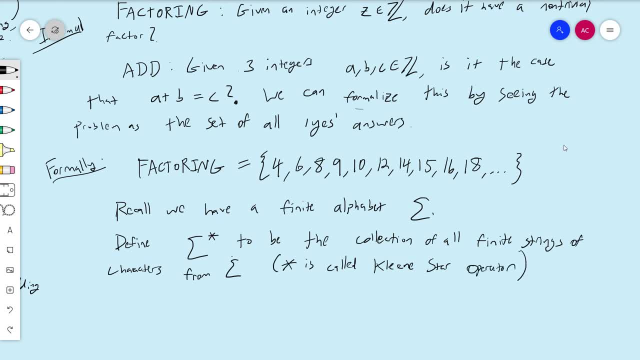 That doesn't really matter. But so this is the set of all finite strings. And so, for the factoring problem, what is sigma, Sigma for the factoring problem is the set of digits. It's 0,, 1,, 2,, 3,, 4,, 5,, 6,, 7,, 8,, 9.. It's a 10-symbol alphabet for the factoring problem. 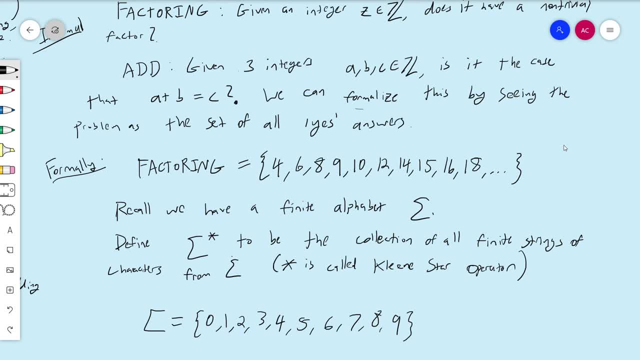 That's kind of the natural alphabet for it, And so you can kind of think of all these numbers. It's going to get into three digits, four digits, five digits. They are numbers, but we're really more thinking about them as strings, really more thinking about them as. 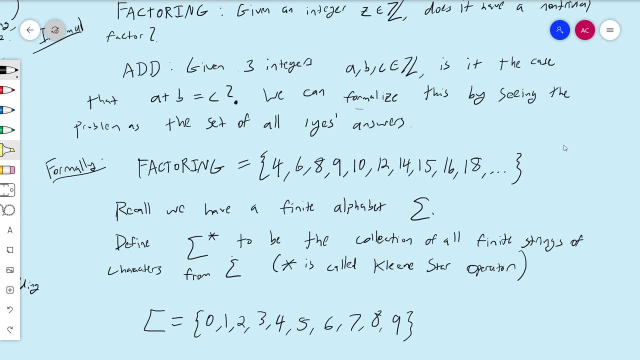 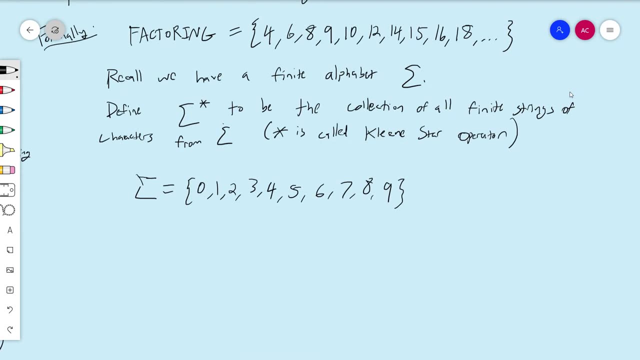 collections of characters over an alphabet, And so what the factoring problem is? oops, I don't want to erase this yet. So what is the factoring problem then? as an object, What it is is factoring. It's a subset, right? The factoring problem is a subset of this sigma star. 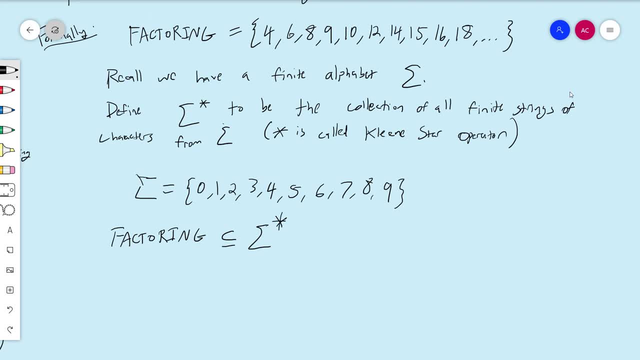 for this particular alphabet sigma. It's a subset of sigma star, And that's how we're going to define a decision problem in the abstract. So here's my definition: A decision problem, otherwise known as a language. I'll talk about why that is in a bit. 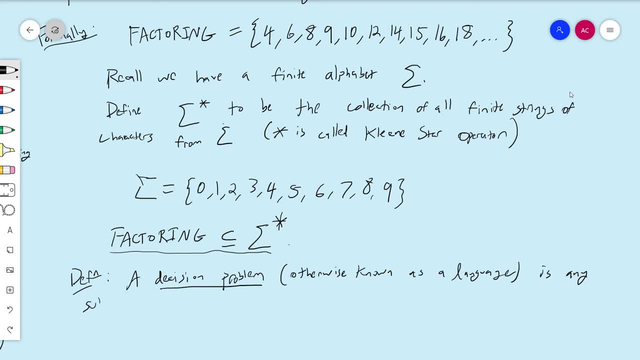 is any subset L contained in sigma star. That's what a decision problem is. A decision problem is a set, It's a set of strings over an alphabet where the interpretation is that the decision problem is always, intuitively the decision is: is X in L. 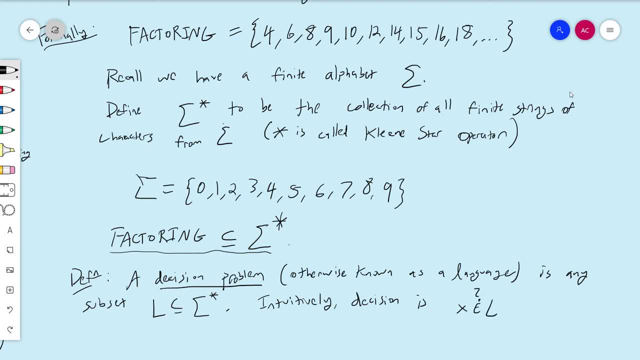 X in L X. in L X is the input and the machine is supposed to give me a yes if it is in the set and a no if it's not in the set. So the factoring problem here: I give it a random integer and 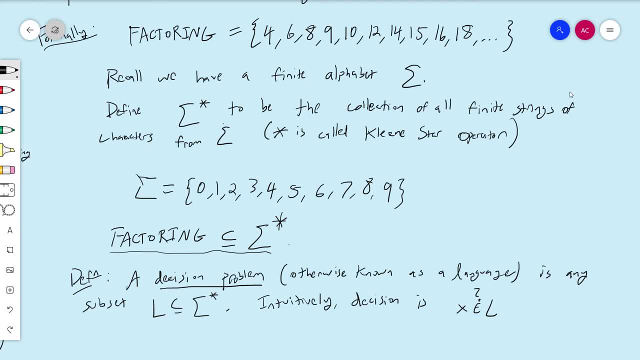 I can sort of frame every decision problem in the exact same way. Not only is it a yes or no answer, but now I can always kind of say that it's not only the same answer but it's the same question. The question is just: are you in the set or aren't you? 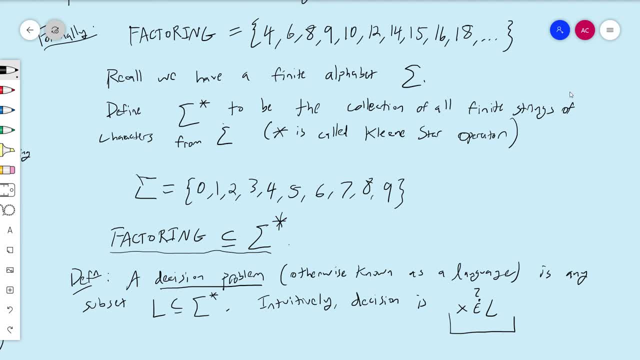 That's the question, and so a decision problem is the set of all the yes answers, It's the subset of the alphabet, And so this is what a decision problem means in the abstract, and now, Now we can finally define what it means for a Turing machine to compute a decision problem. 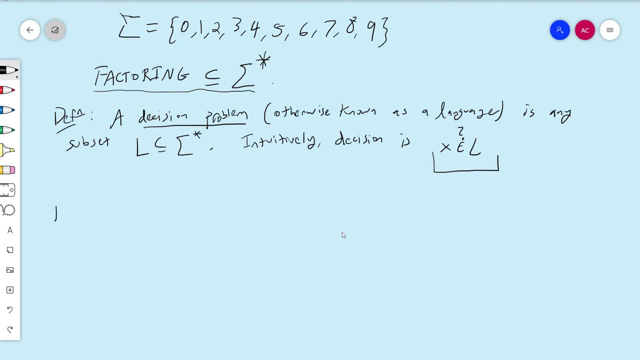 Okay, so Let L. Okay. why is this a language? by the way, Why is the other word for decision problem a language? I am going to use the word language a lot, by accident. It's because there's this very deep connection between computability theory and actually formal linguistics. 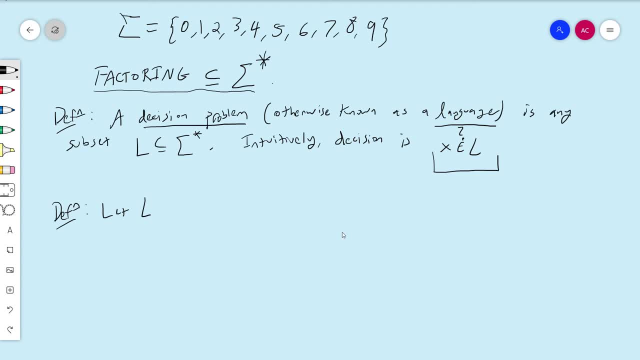 In the sense that: how did I get? There's a way to build languages out of an alphabet. You know if, instead of thinking about an alphabet, don't think of it as an alphabet, but necessarily In order to understand why it's called language, instead of thinking about alphabets, think about these symbols as sort of like words in a language. 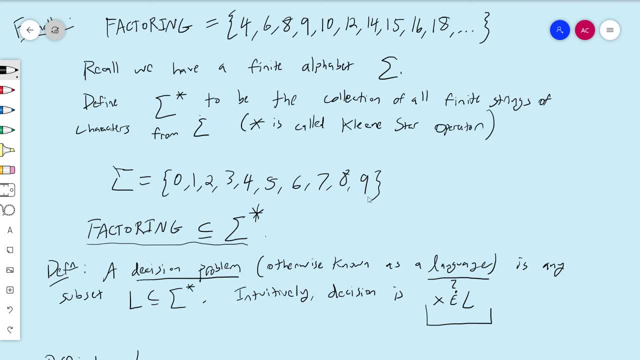 And then I could specify, I could give. What I could do is I could create a grammar. I could define rules for how to put these things together, Like what does sentence structure look like, and stuff like that. I can define a set of rules called a grammar. 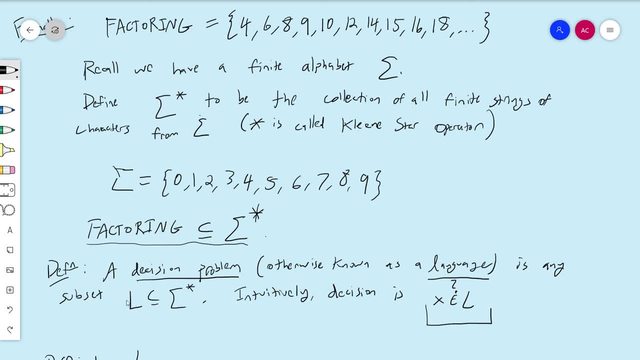 And then out of that grammar you do get a set of all valid things, You get a decision problem. And so the decision problem in that context of linguistics is: is this a valid sentence in the language, Or is this a valid sentence? 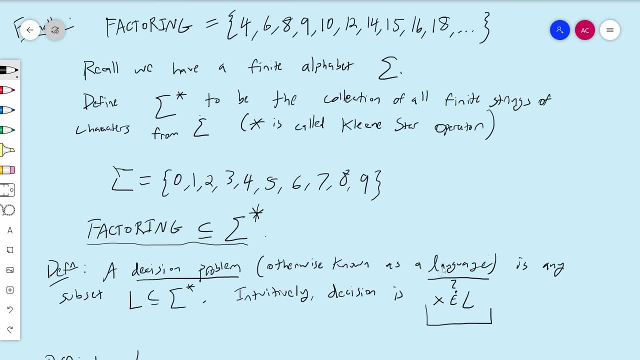 Yeah, So that's why you call these languages. It's kind of you start with a set of words or symbols and then you define a grammar And then that creates for you a decision problem And there's a deep connection between categories of machines and languages. but that's not something I'm going to get into anytime soon. 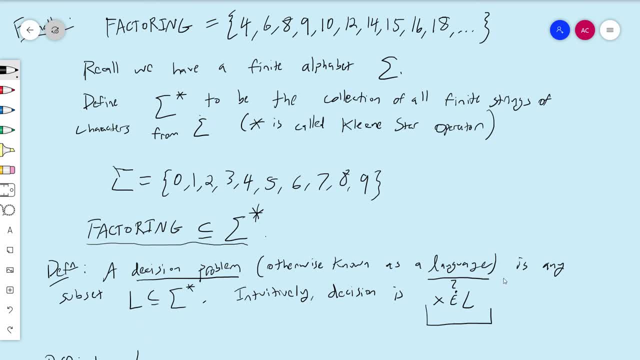 But because it's less syllables, I think people like to say the word language instead of decision problem, And I am one of those people, So I will say the word language quite a bit. When I say language, I mean decision problem. 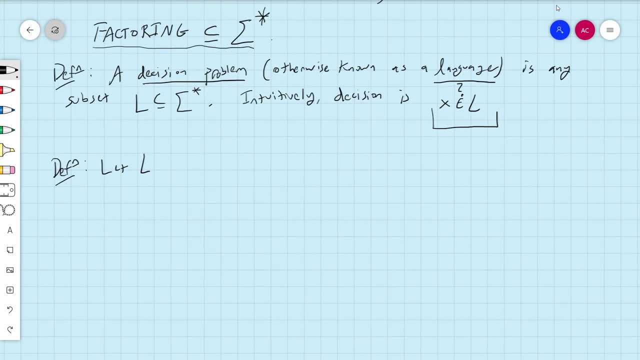 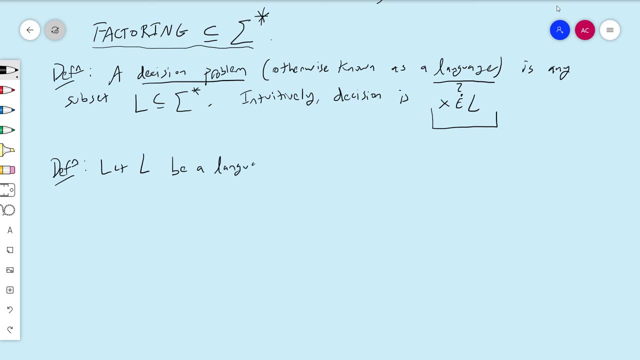 Kind of weird, but it is what it is. In a lot of textbooks they use languages too. So let L be a language or a decision problem. Let L be a language and then M be a Turing machine. We say that M decides L. 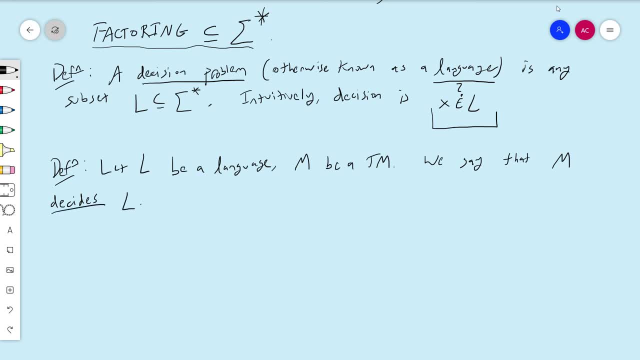 Oops, Other words. There's a lot of words for this, because this is the definition. We say that M decides L, but instead of decides I could have used the word computes, I could say the word solves, I can say the word decidable, computable. 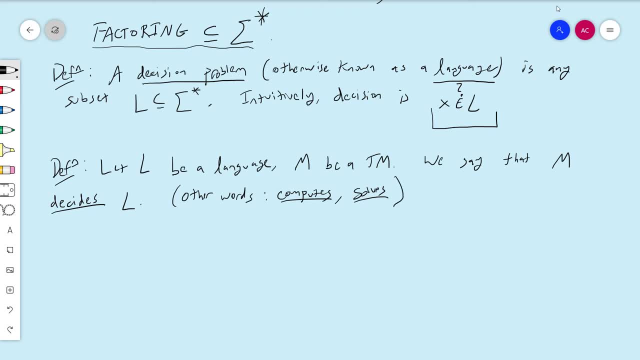 I could say: well, yeah, that's pretty much the only two other words. So M decides L, M computes, L, M solves L. We're defining what it means to decide To actually solve a problem in general, If the following is true: 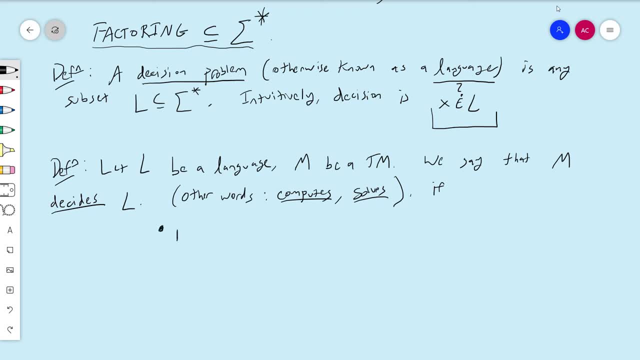 Two things have to be said. One, if X is in L, Let me just go ahead and say it like this: If X is in L, then what should happen? Well then, M should accept it In some number of steps. 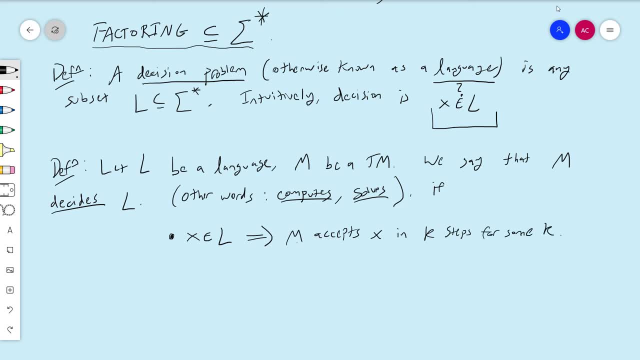 So if X is in L, then M accepts X in K steps for some K, And then if X is not in L, then M rejects X in K steps for some K. That's what I mean. This is the definition of deciding a language. 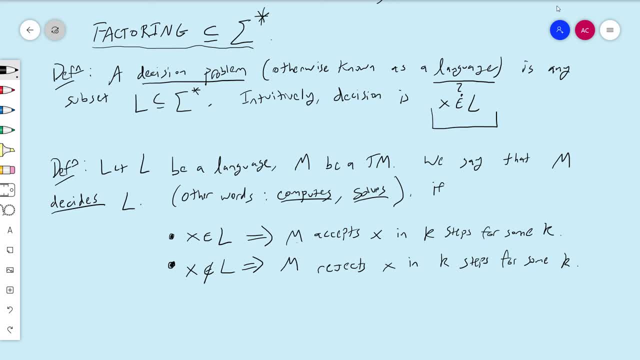 If you're in the set, then M accepts the input, And if you're not in the set, then it rejects it. That's the definition. So there's a thing I want to say about that, But before I do, we're almost done. 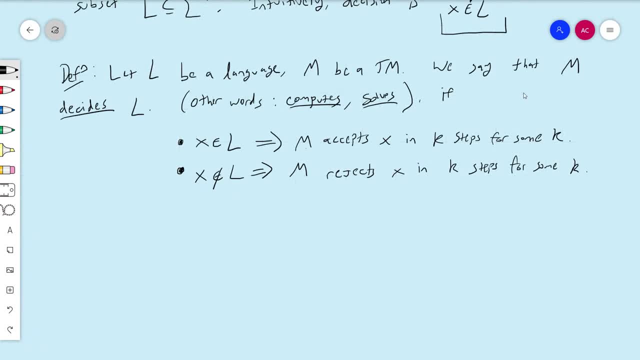 I know this is going very long, But this is the hardest part. This initial definition is probably going to be the hardest part of any of my videos that I'm going to make. Okay, In terms of just, there's a lot to digest here. 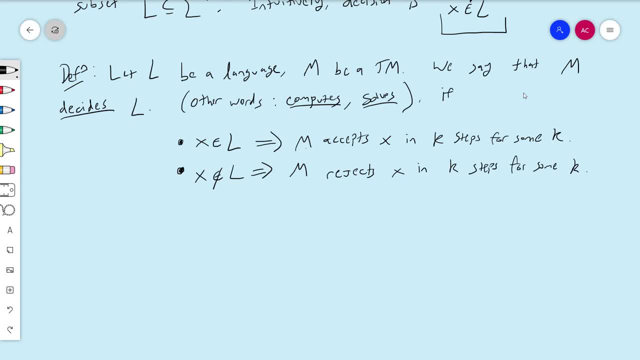 You're going to have to go through this a few times and really kind of categorize it, I guess. So now we want to talk about the problems. We say that a language, L, is decidable- Decidable, I, you know- or computable. 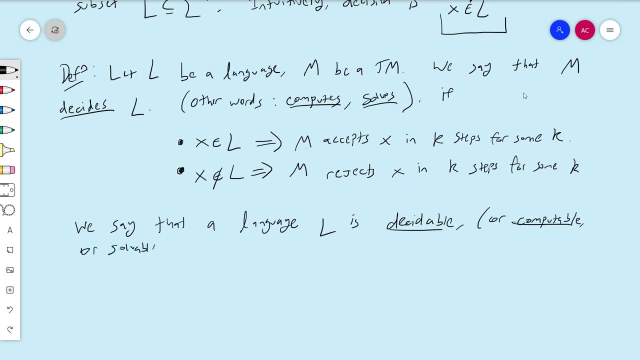 Or solvable or whatever, And there's actually one other word that we use for it- or recursive, That's another word for it. All of these are words for the same thing: to say that L is computable, Computable, solvable, recursive, decidable. 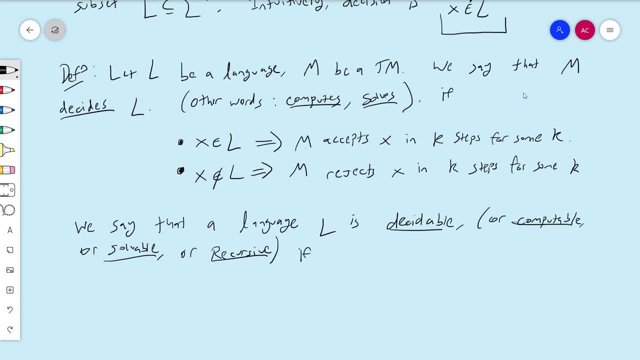 These are all going to mean the same thing: L is decidable if there exists, If there exists, a Turing machine that decides it. That's what it means. So we finally did it. It took I don't know how long, But we finally defined, we finally formalized what we've been talking about. 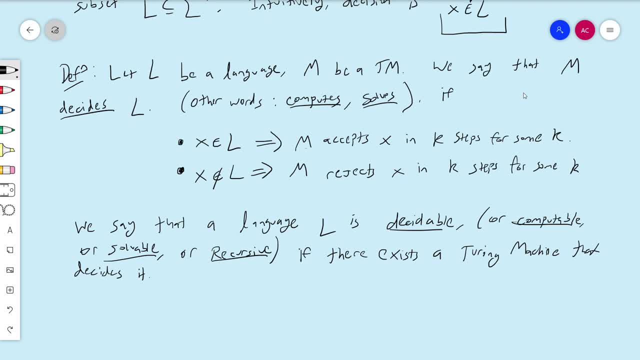 We have what a decision problem means. We have what it means for a decision problem to be, To be computable. We defined our Turing machine model formally And now we know exactly what it means to say that a language is computable. I know that was a lot. 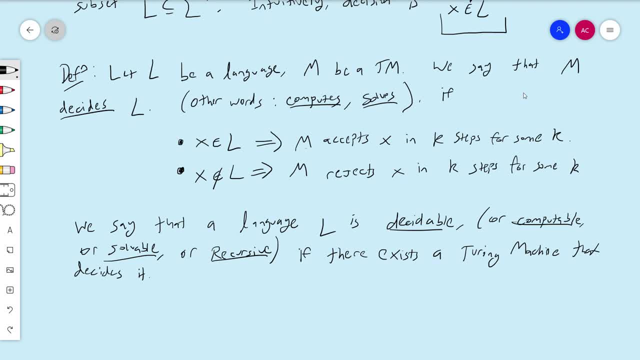 I know that was a lot to absorb in one video, But what we're going to do in the next couple of videos is we're going to do a lot of examples. We're going to do examples. I'm going to show you. We're going to go through the process of designing Turing machines that compute problems. 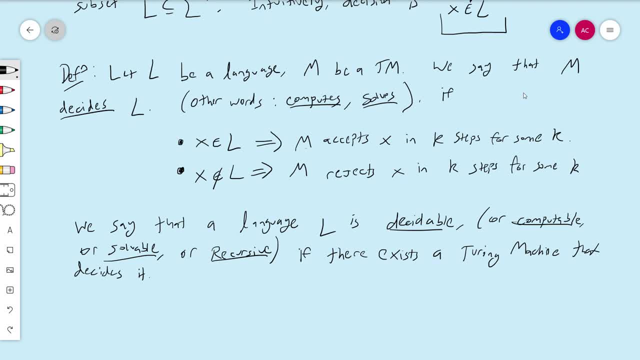 And we're going to think about them And you'll get used to them through that. But I do recommend, before moving on to those videos, That you look through this definition closely, That you maybe write it down yourself And that you think about it. 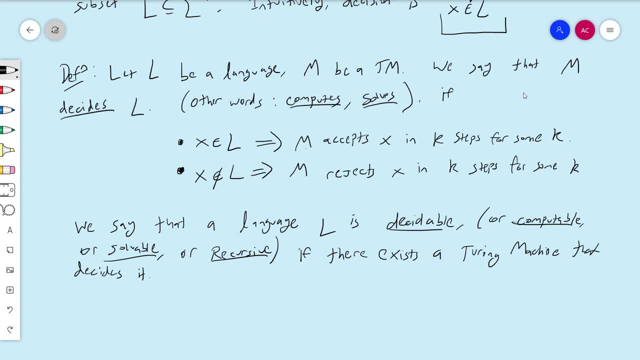 And if you have any questions about it, please ask me in the comments. A couple last things I want to point out. One: why did I have to say two different things here? Why wouldn't it have? Why wouldn't? Why isn't it enough to just say: 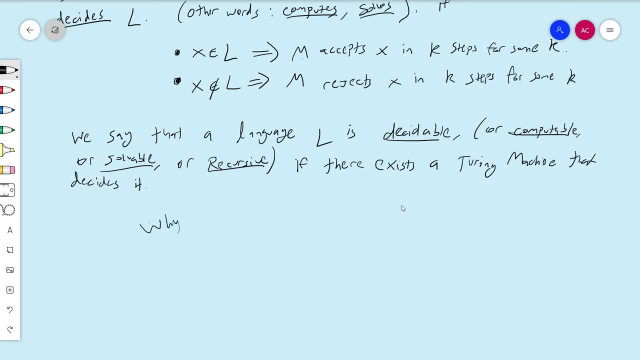 Oops, Why can't I write Instead of: Instead of these two separate points? why can't I just write one point? Why can't I just say X is an L if, and only if, M accepts X in K steps For some K. 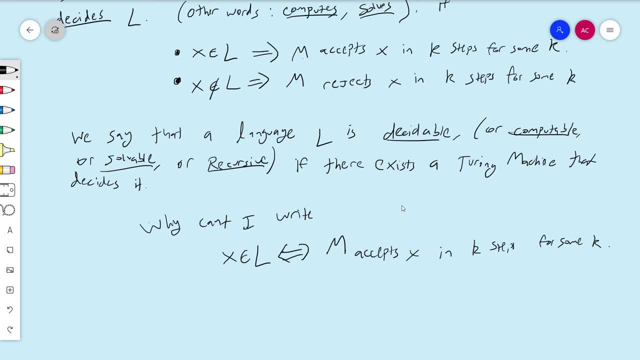 Why can't I do that? Why don't you think about that? In fact, actually, I don't want to tell you the answer. I mean, this should be something that you should be able to figure out the answer to. I'll tell you in the next video what the answer is to this. 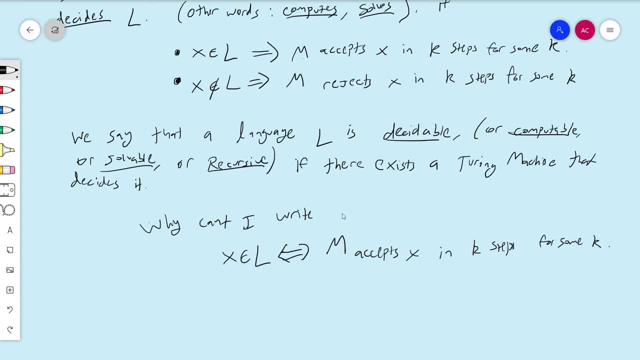 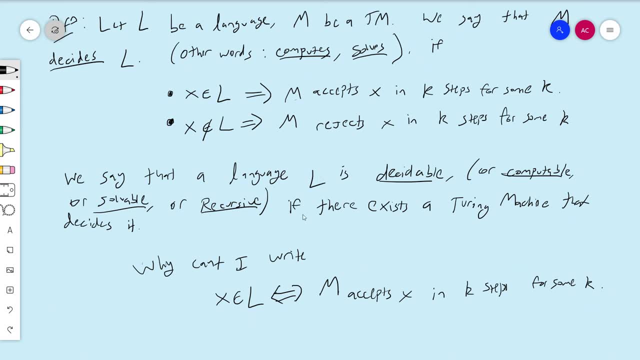 Why, Why, Why does the definition of deciding a language have to involve two different points? Where X is an L means M accepts, And where X is not an L means M rejects. Why isn't this good enough? Why can't I just make it a two-way street with the positive? 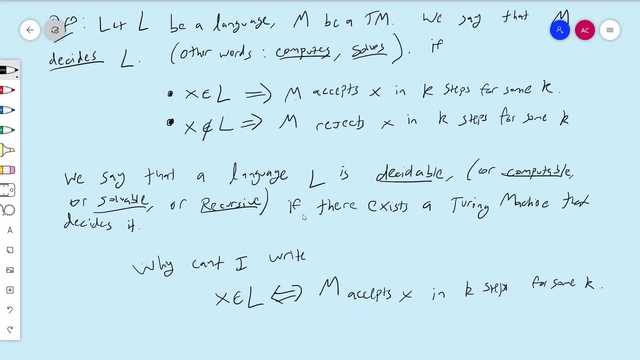 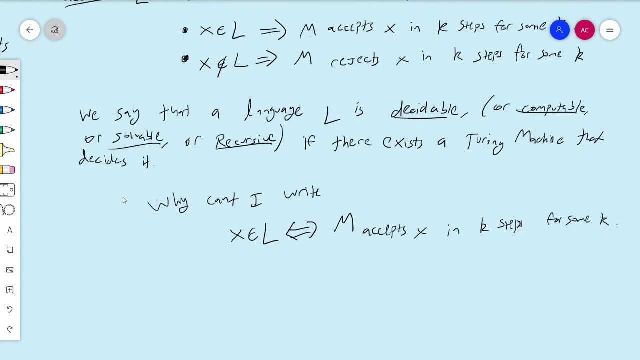 Where X is an, L means M accepts. Think about that. And then another thing to do is one last definition, Really important definition. We're going to come up with our first category of problems. So So we call the set of all recursive or computable problems or languages. 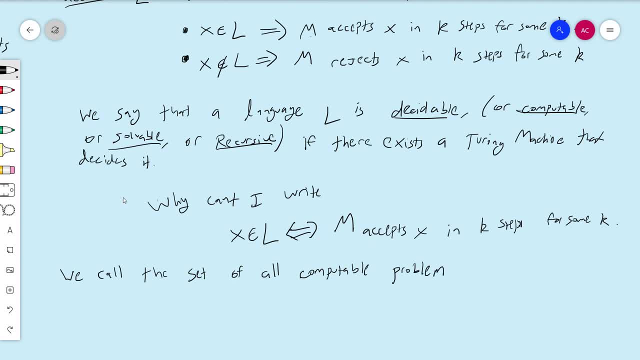 Again, problems and languages are kind of the same. They are used interchangeably. R- That's what we're going to define it as The set of all languages that have Turing machines that compute them is denoted R. This is our first complexity class or computability. 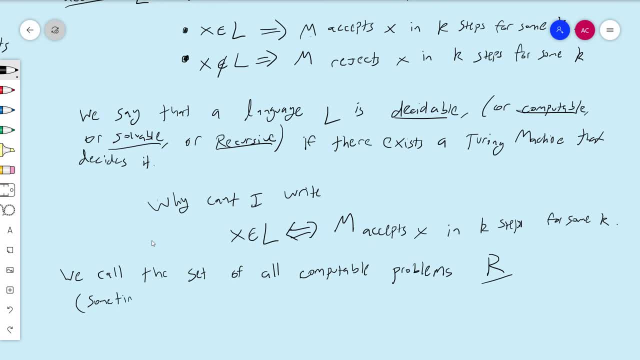 This is our first class of problems. And then sometimes also sigma star is referred to as all, All languages, Because that's what it is right. It's just the set of all languages. Well, actually, No, it's not actually. 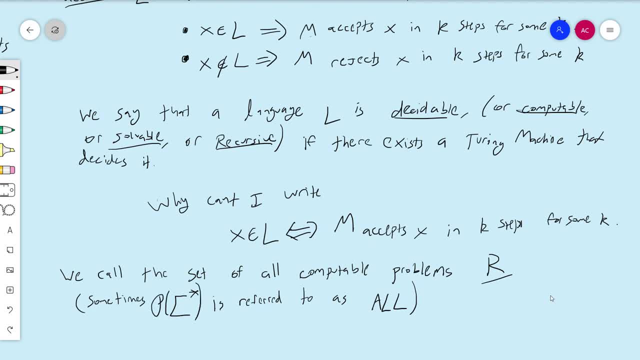 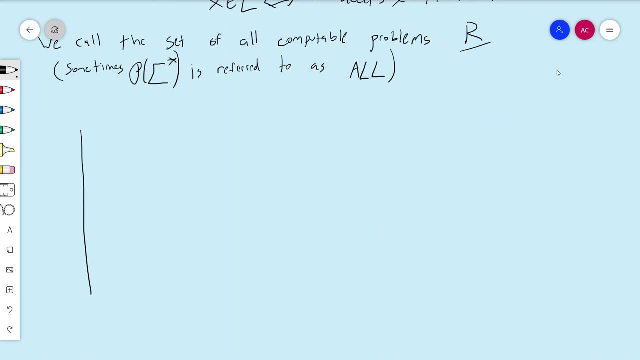 I'm sorry, The power set Of that is all, And if you don't know what power set is, again, check my set theory notes. But we can finally draw the landscape. What you're going to see is that this class sort of turns into a zoology class where our job is to categorize things. 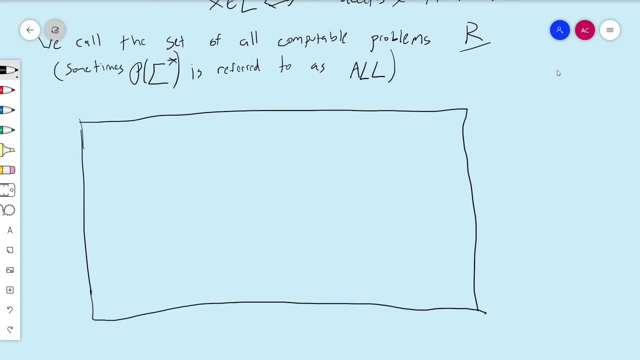 We have a fixed alphabet And then we have kind of two big classes, We have all, All languages, And then we have the recursive languages, R, And so you might be questioning: What is the difference between these two things? The fact that I drew it this way implies that there does exist a language that is not recursive. 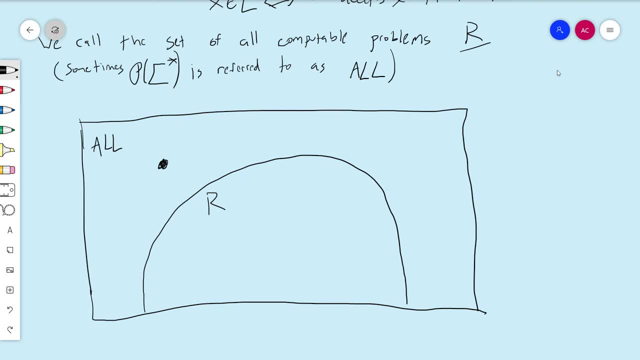 And there is plenty- Most of them, in fact- And so we'll talk about that very soon. We'll define a language that is not recursive- That there is not. We'll talk about problems that are not computable, But most of our time is going to be spent inside of R. 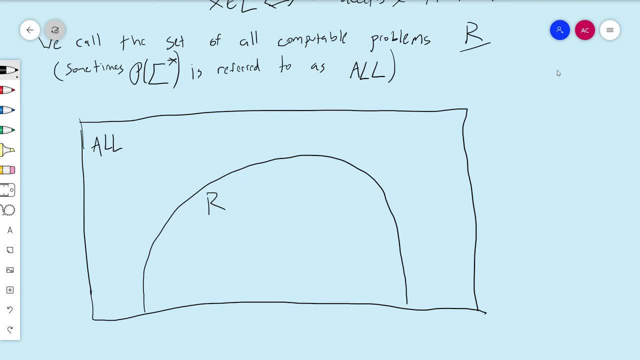 In fact inside of a special class called re, But the beginning of our zoology project has happened at this point. We've defined the two biggest kind of complexity classes- Not really biggest, but anyway. next time we will do examples, We will make Turing machines that solve problems for us. So look through what I just told you and I'll see you then. 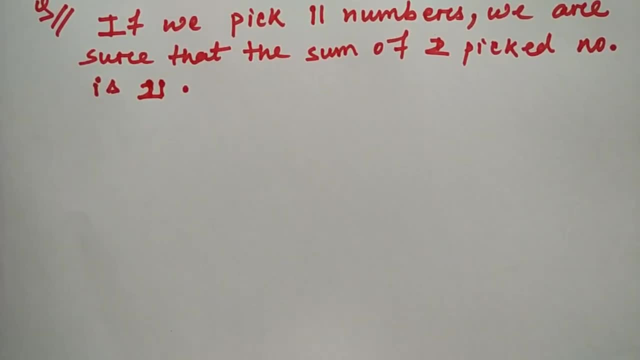 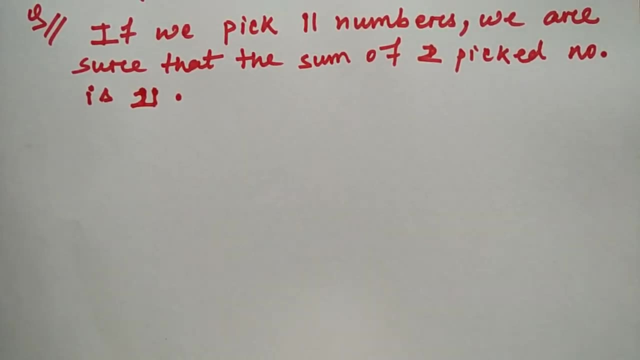 We will solve some problem of pigeonhole principle. So you can see here this is a question. If we pick 11 numbers, we are sure that sum of two number is 21.. So let me write down first all the 11 number. 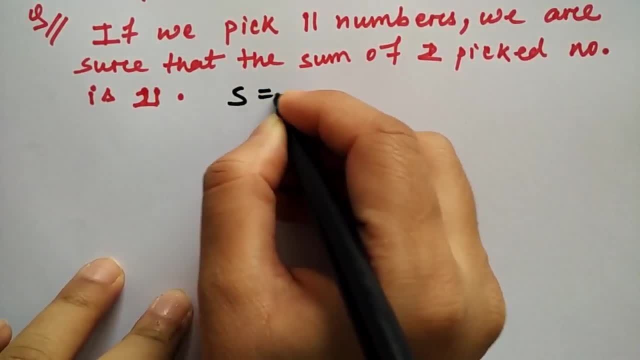 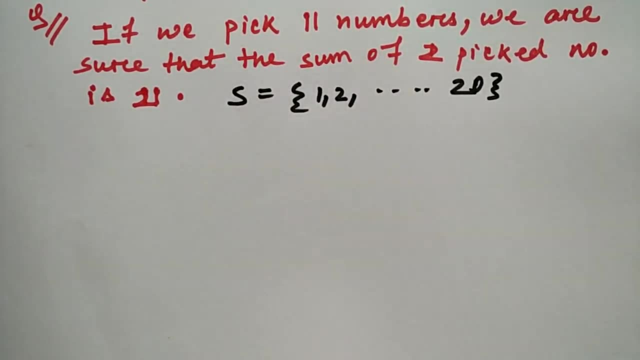 And the most important. the set is given as 1,, 2 up to 20.. So the question is: if the number between 1 to 20 selected is 11, then out of the 11 number, when you are picking two number, the summation of those number will be 21.. 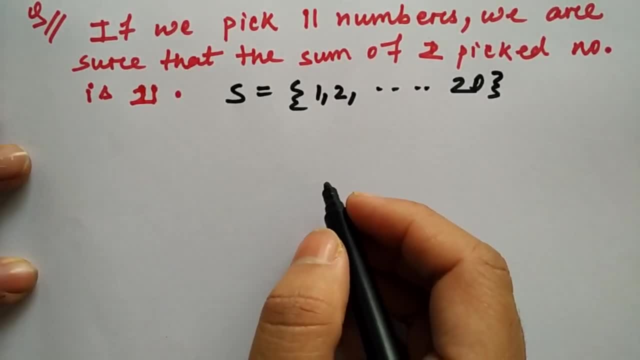 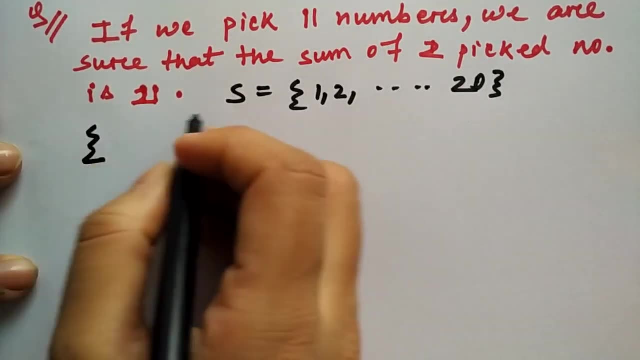 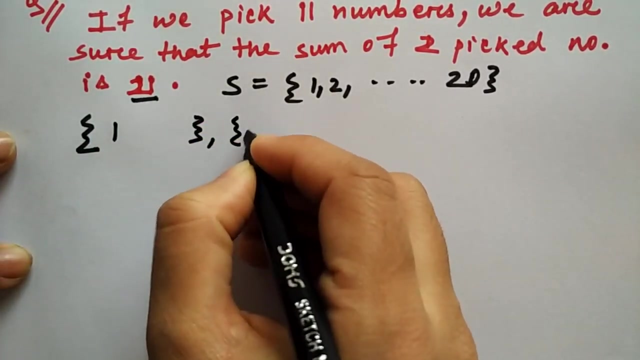 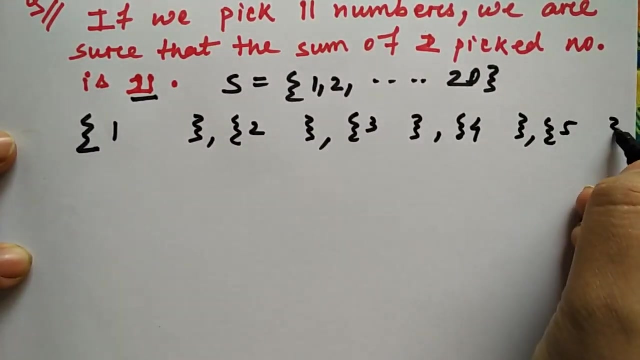 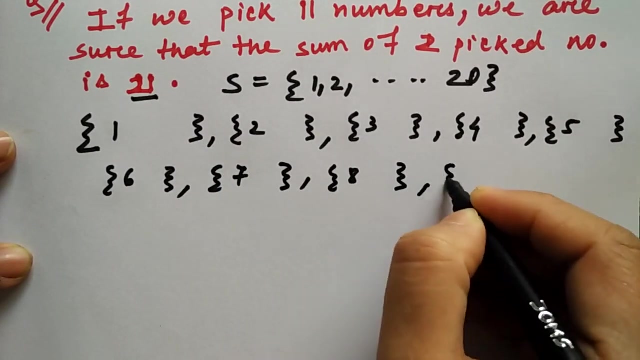 So 1 to 20,. let me write down the numbers first In place in accordance with what Summation is 21.. So how to write this? First, let us write 1,, 2,, 3,, 4,, 5,, 6,, 7,, 8,, 9, and 10.. 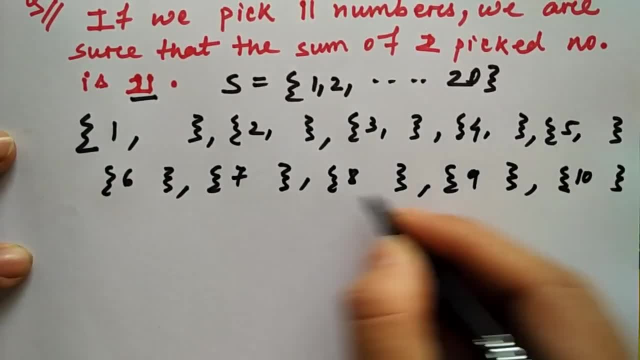 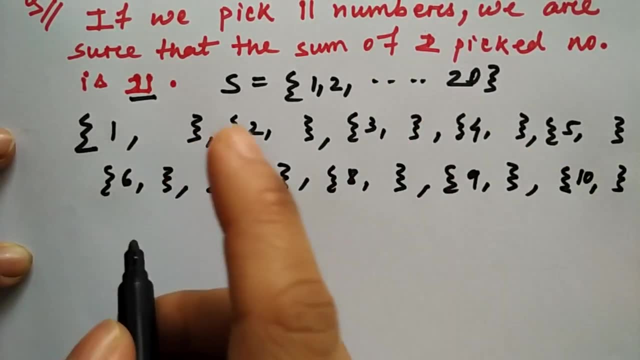 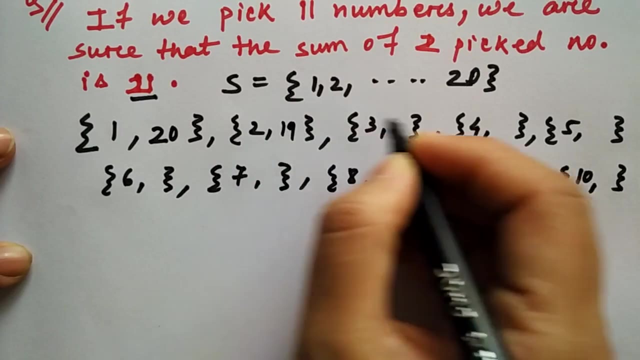 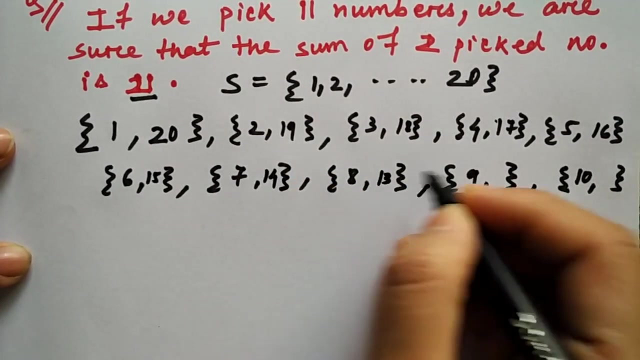 Okay, So I have written all the 10 numbers. So, with this number, what are the other number you are adding So that you will be getting the summation as 21.. So first will be 20.. In between 1 to 20, remember that 19,, 18,, 17,, 16,, 15,, 14,, 13,, 12, and 11.. 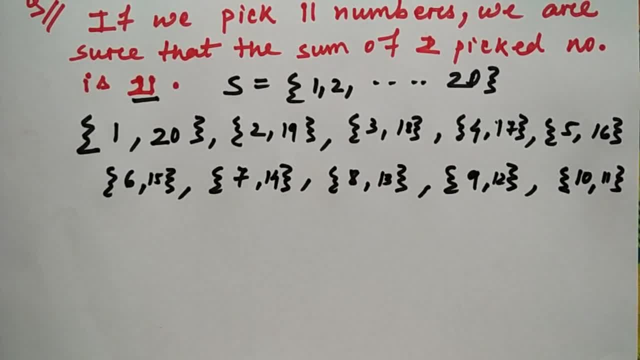 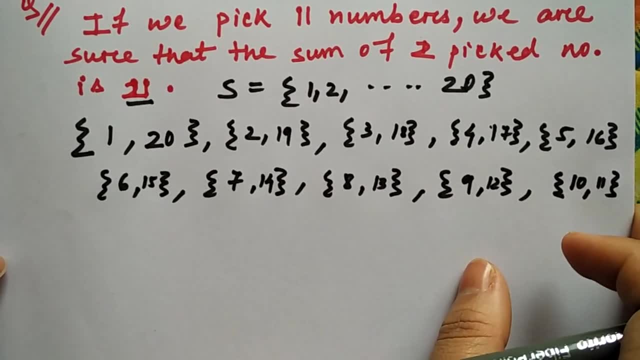 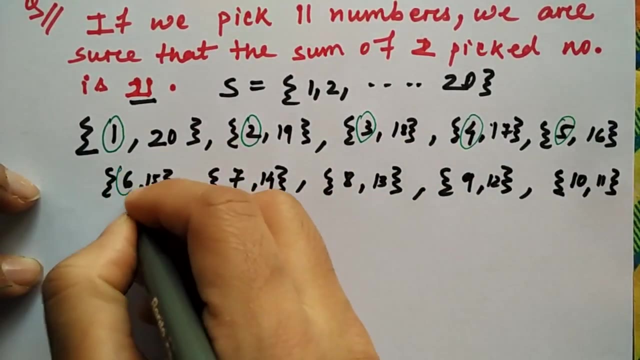 Okay, So this is very clear Now what it is saying: that out of all the 21. 20 number, if you are picking 11 number, the sum of any two number will be surely 21.. So let me randomly pick 10 numbers, that is, 1,, 2, 3,, 4,, 5, 6,, 7,, 8,, 9,, 10.. 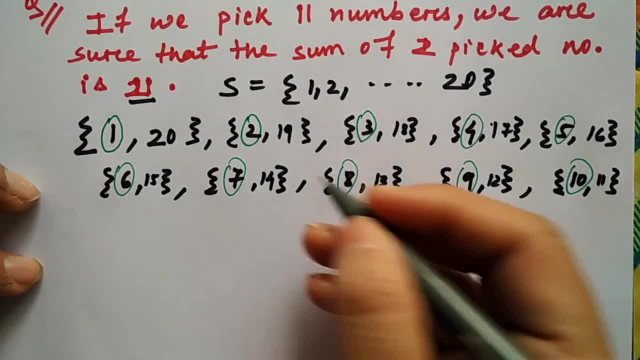 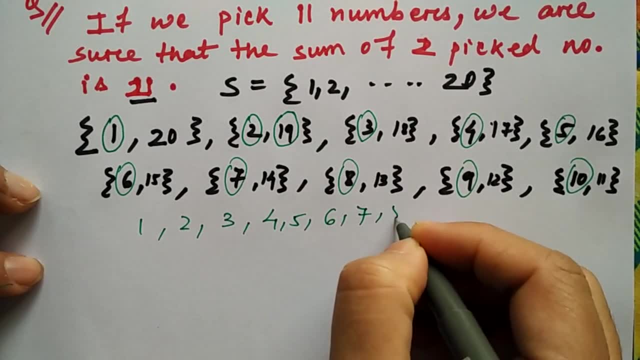 So I have selected 10 number. Let me take the 11th one as 19th. Okay, So my 11 values are 1,, 2,, 3,, 4,, 5,, 6,, 7,, 8,, 9,, 10, and 19..